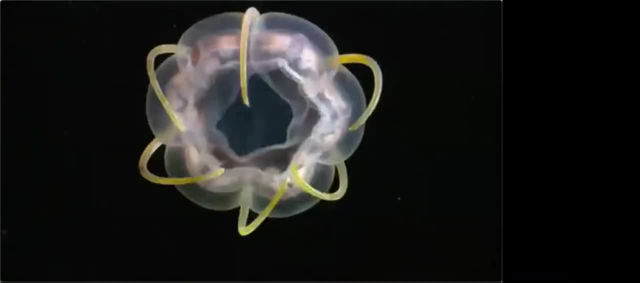 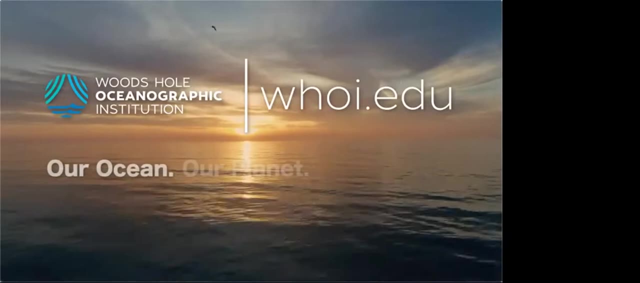 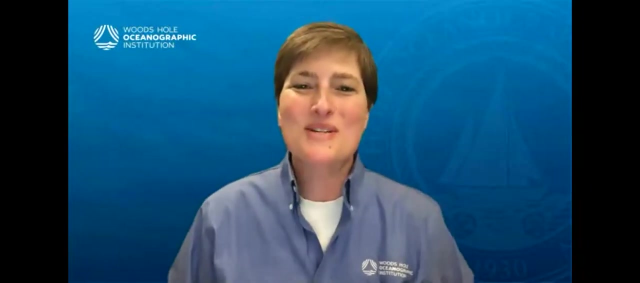 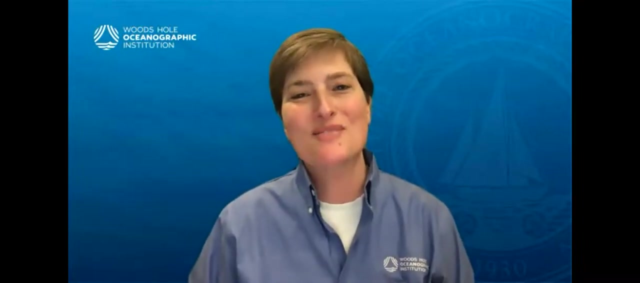 exploration and education, working to understand and sustain one of humanity's most precious common resources. Join us today for our ocean, our planet and our future. Welcome to the Ocean Encounters. virtual series from Woods Hole Oceanographic Institution, or HUI as we like to call it for short. Tonight's presentation is Making Ocean. 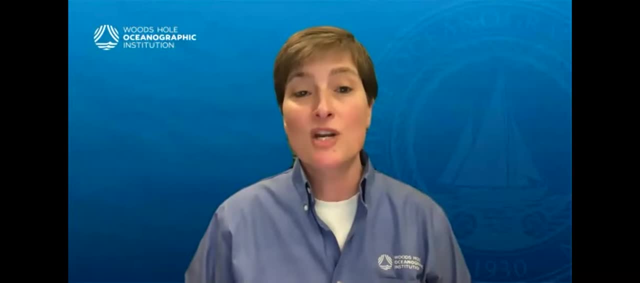 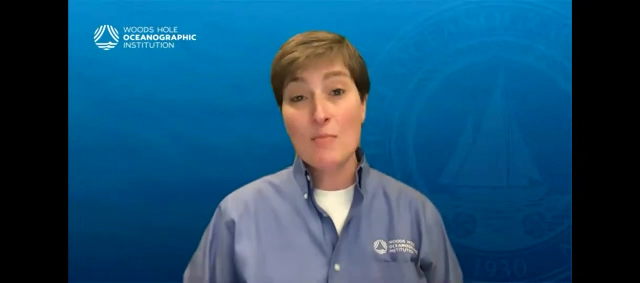 Conservation Work, Combining Science, Community and Policy for a Sustainable Future. HUI's Ocean Encounters- online events are made possible by the Avatar Alliance Foundation and Dalio Philanthropies. Thank you, My name is Veronique Lacapra. I'll be your host for this. 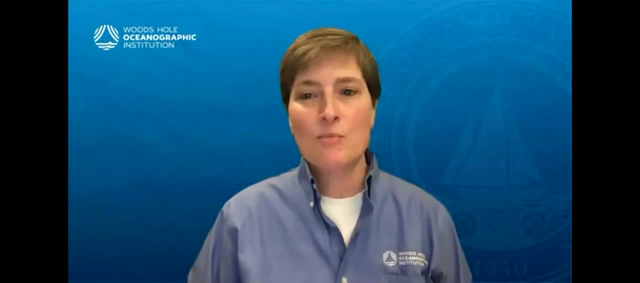 evening. Before we hear from tonight's presenters, I'd like to take a minute to share some tips on how you can optimize your Zoom experience with us. Later on in the evening, our panelists will be taking questions from all of you, and if you'd like to participate in this live Q&A, please use. 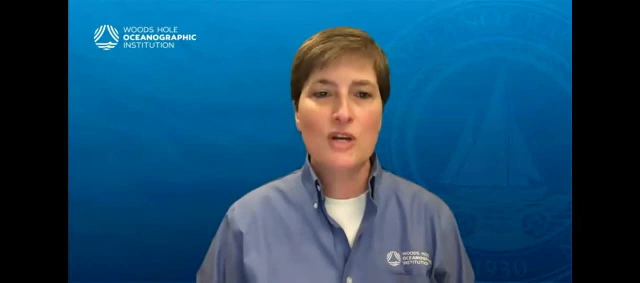 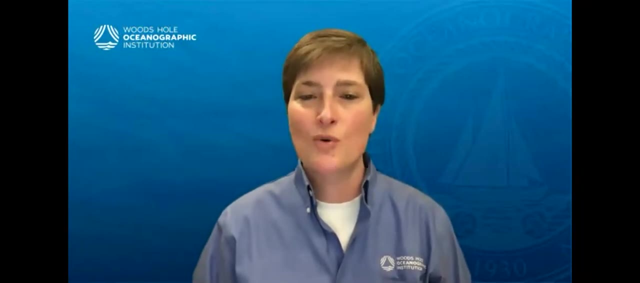 the Q&A button on your Zoom screen to type your question in the window that appears. You may be more familiar with the chat function in Zoom, but for tonight, please use the Q&A function instead. We often get hundreds of questions, so I apologize if we don't get to yours while we're live. 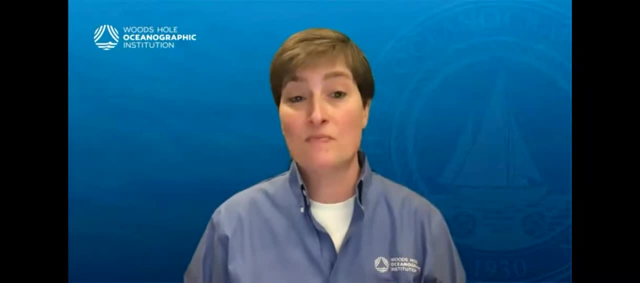 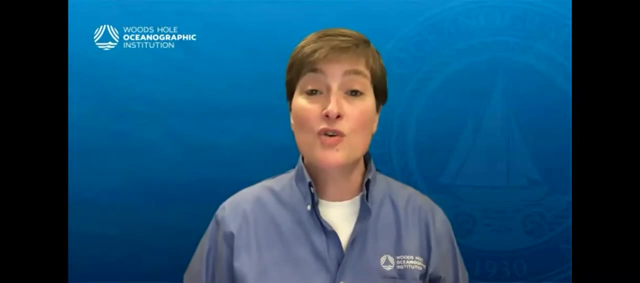 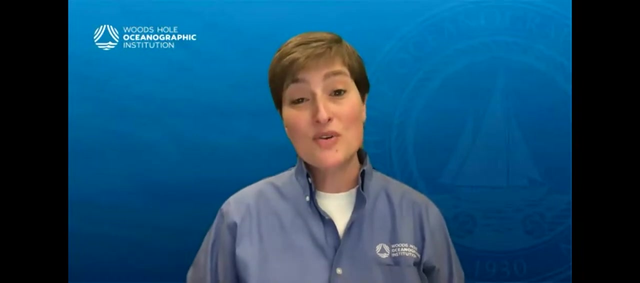 You can ask questions anytime, starting now. I also want to let you know that we are recording this event. That recording will be made available on the huiedu website, That's w-h-o-i dot e-d-u. We had more than 1,200 people pre-register for this event, so you're in very good company. 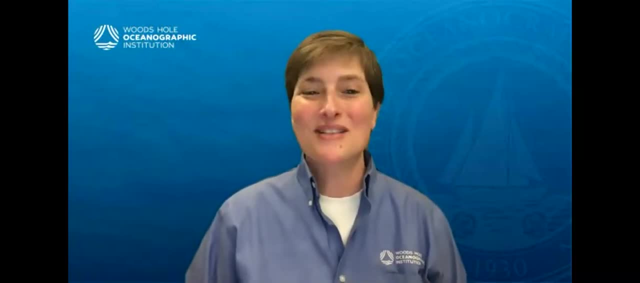 Thank you and welcome to you all. All right, let's get started. Achieving success in ocean conservation. Ocean conservation is a complex navigation of science, policy and the needs of local communities, but it is achievable. Tonight we'll hear how scientists, communities and 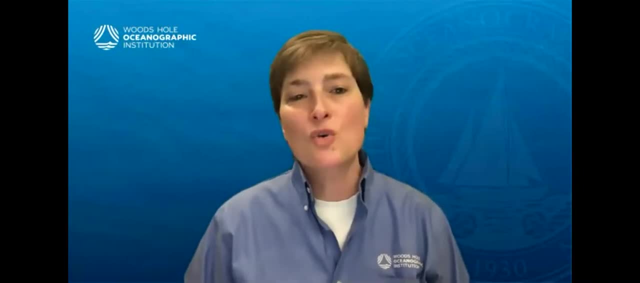 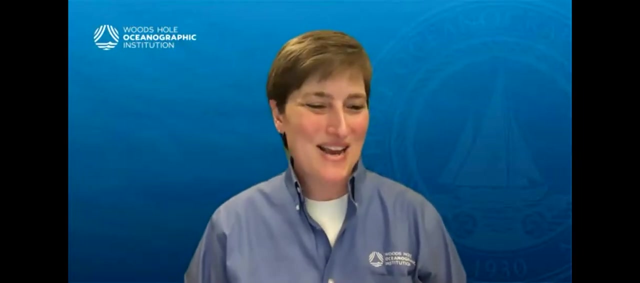 non-governmental organizations or NGOs are joining forces to inform policy and together create workable, sustainable strategies for critical ocean ecosystems. We have three speakers with us this evening. They are Hui Coral Scientist, Anne Cohen, the Executive Director of the Center for Ocean Conservation, and Anne Cohen, the Executive Director of the Center for Ocean Conservation. Anne Cohen, the Executive Director of the Center for Ocean Conservation, and. Anne Cohen, the Executive Director of the Center for Ocean Conservation. Anne Cohen, the Executive Director of the Center for Ocean Conservation. Anne Cohen, the Executive Director of the Center for Ocean Conservation. 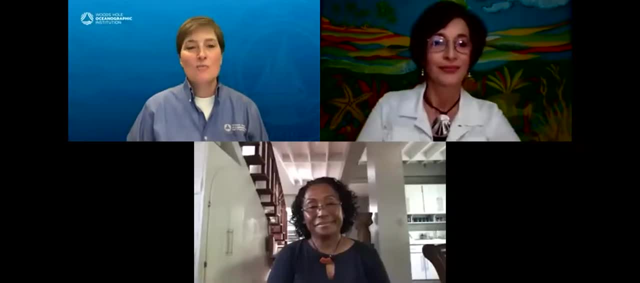 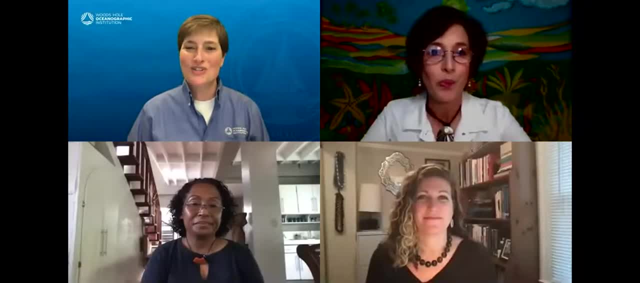 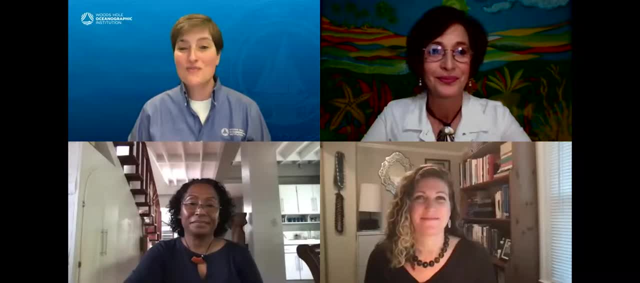 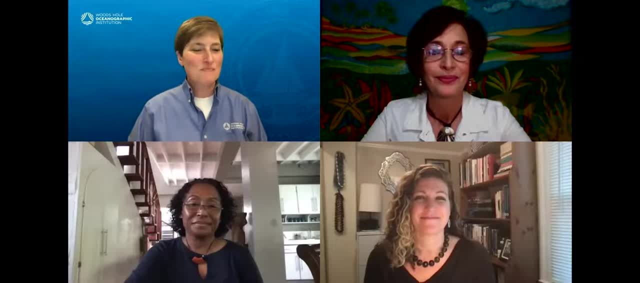 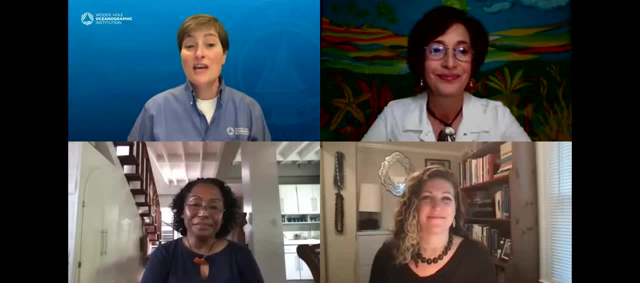 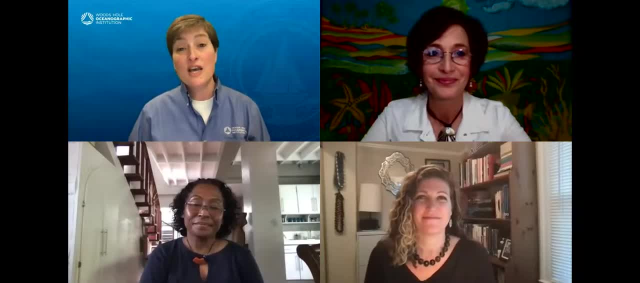 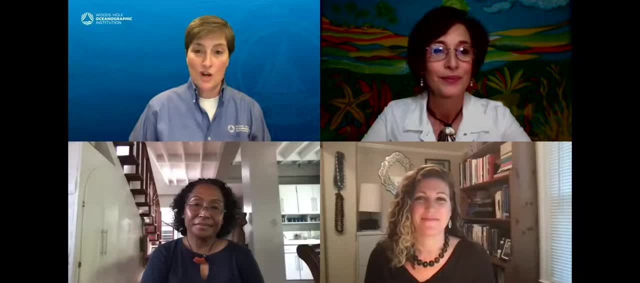 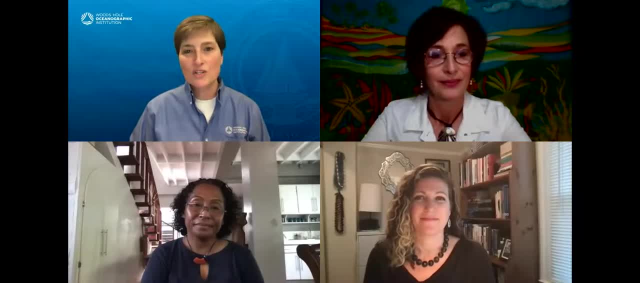 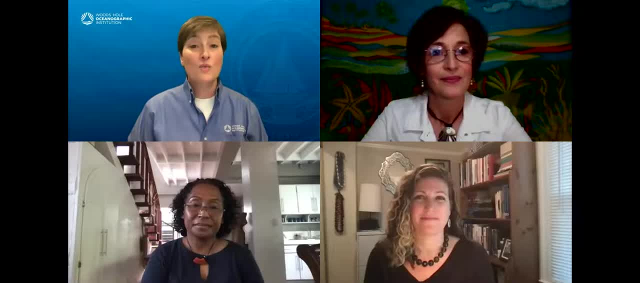 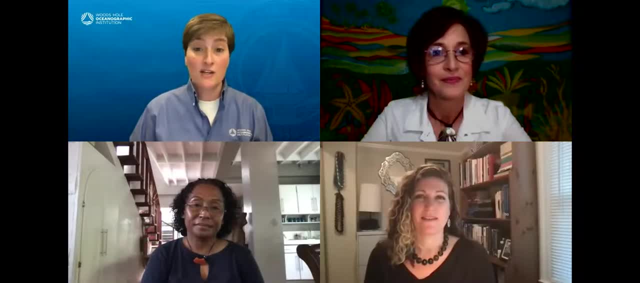 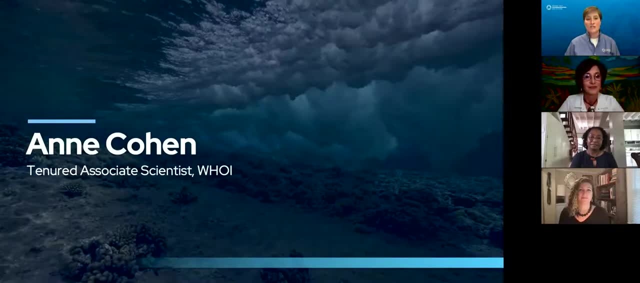 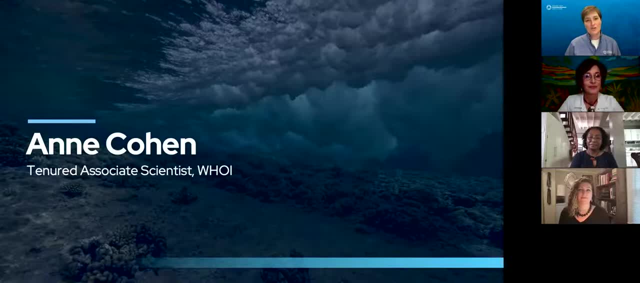 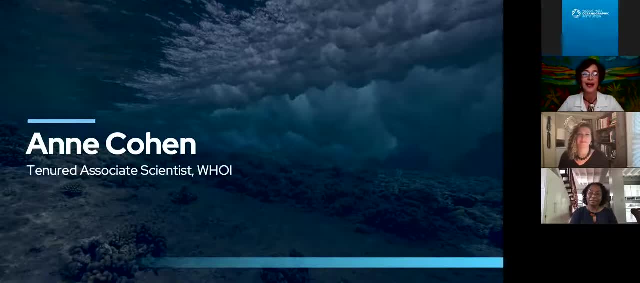 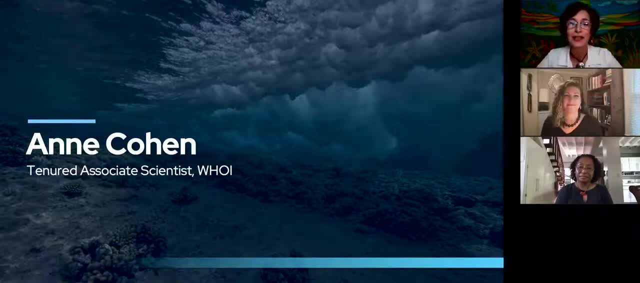 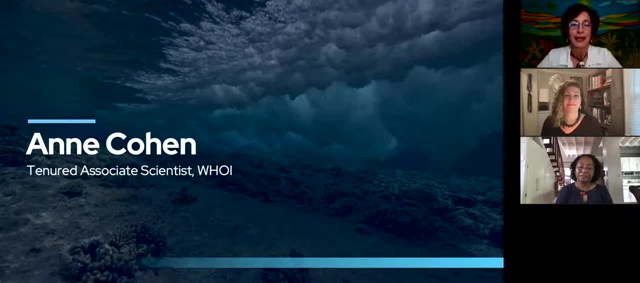 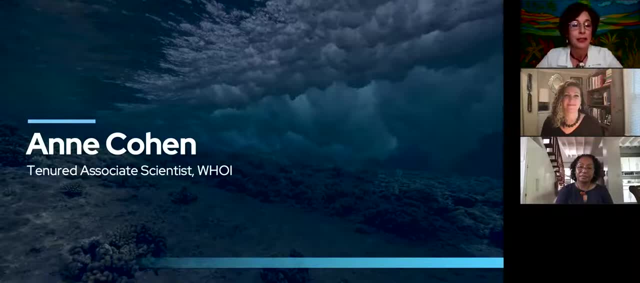 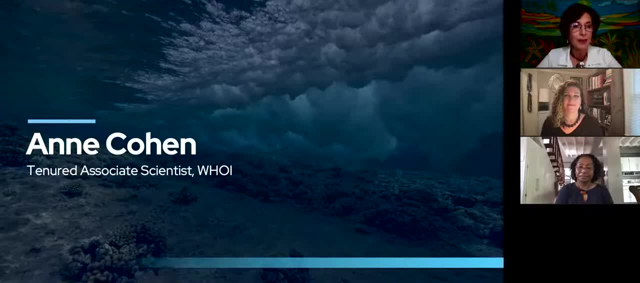 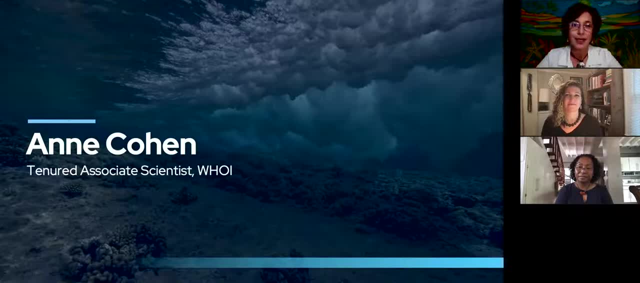 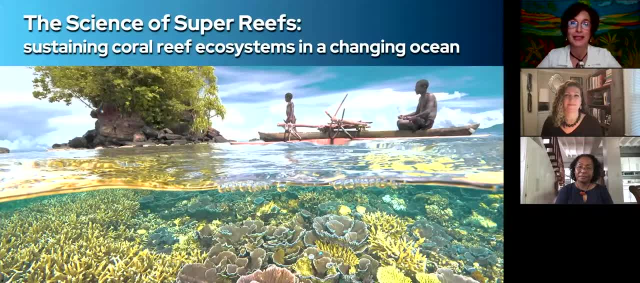 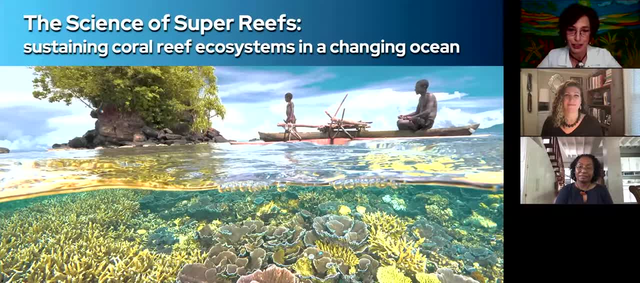 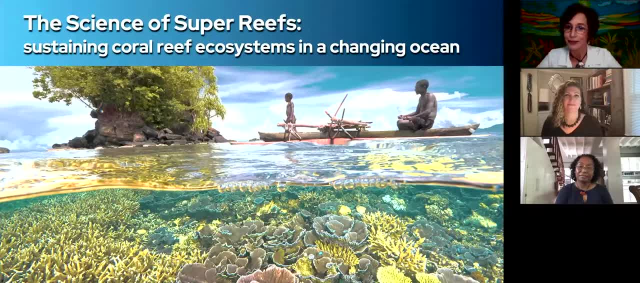 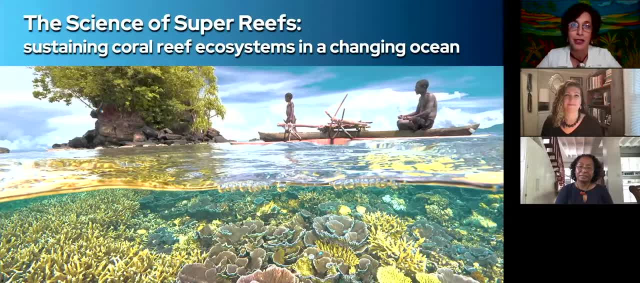 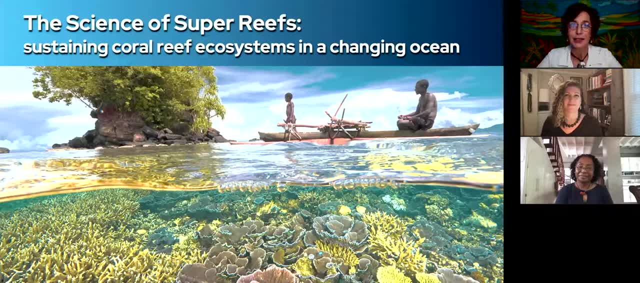 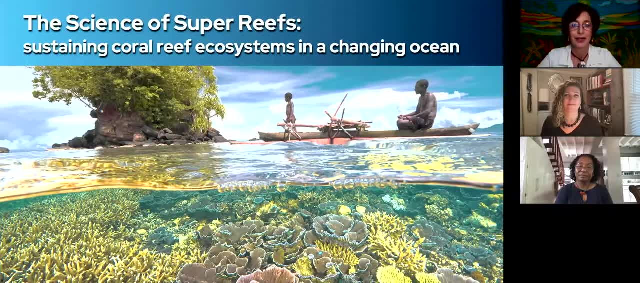 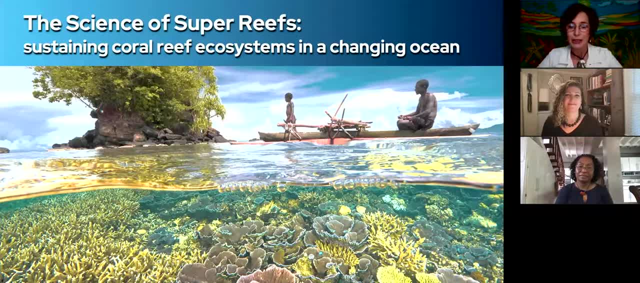 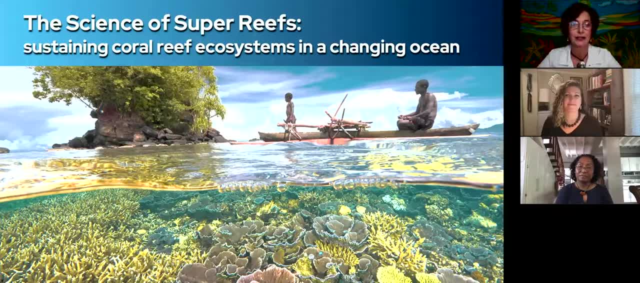 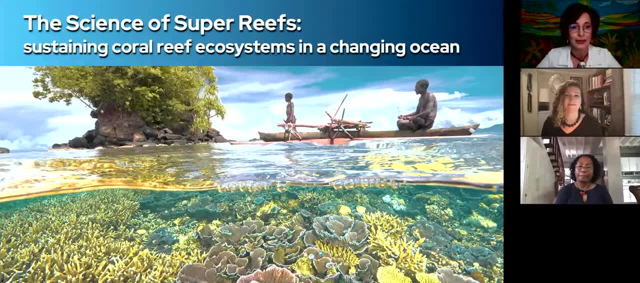 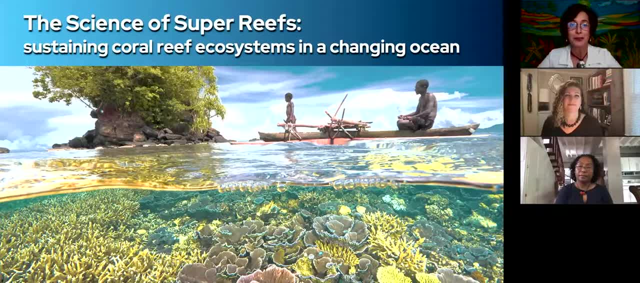 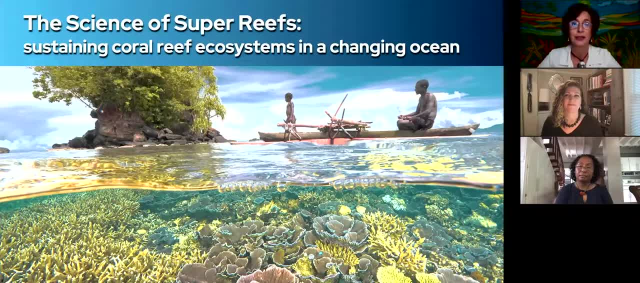 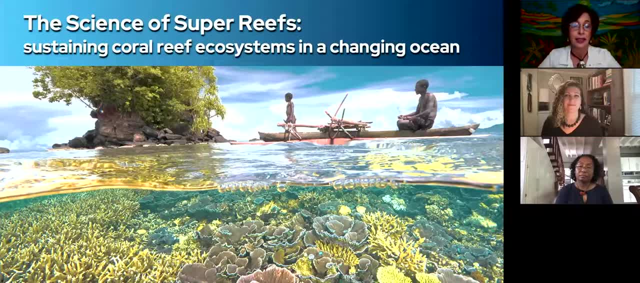 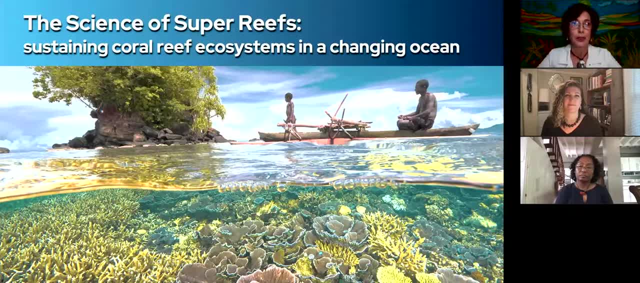 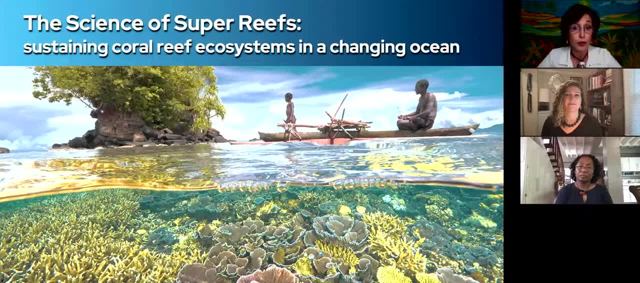 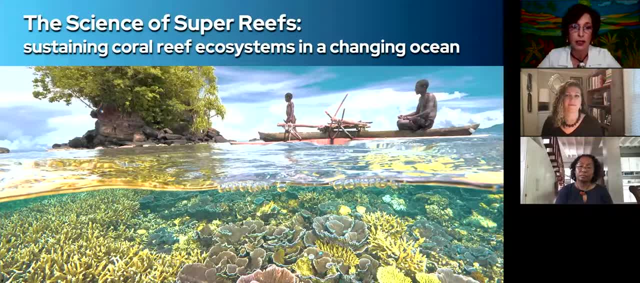 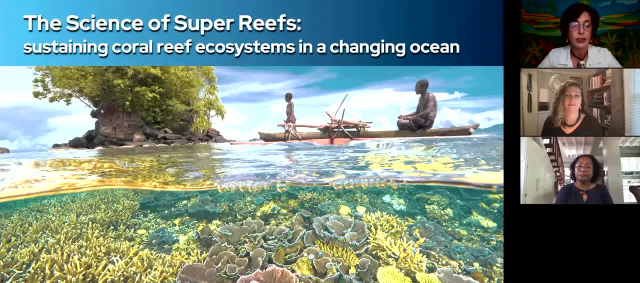 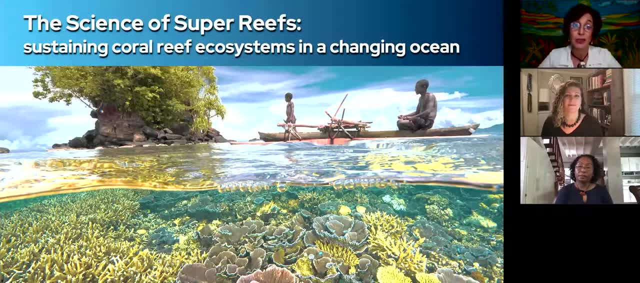 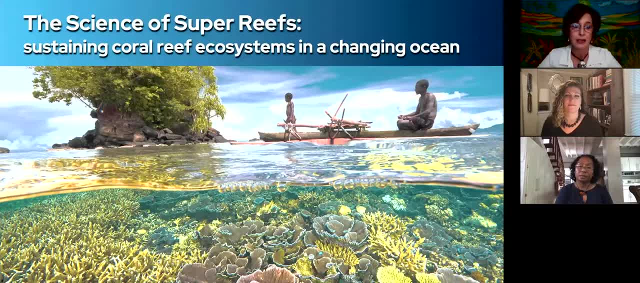 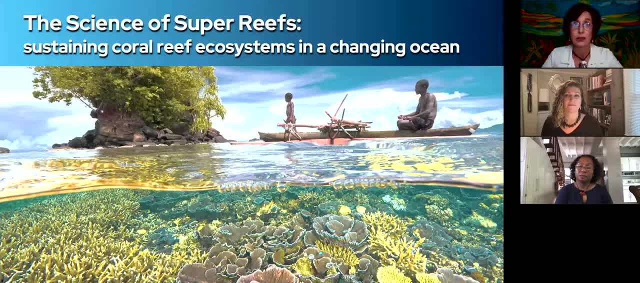 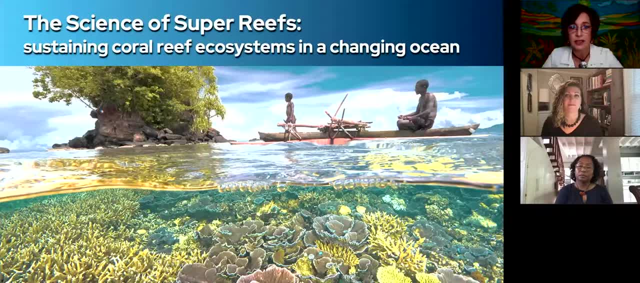 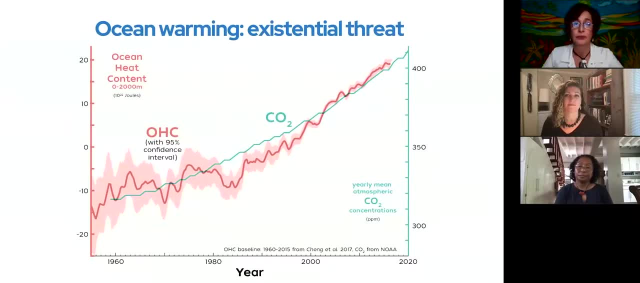 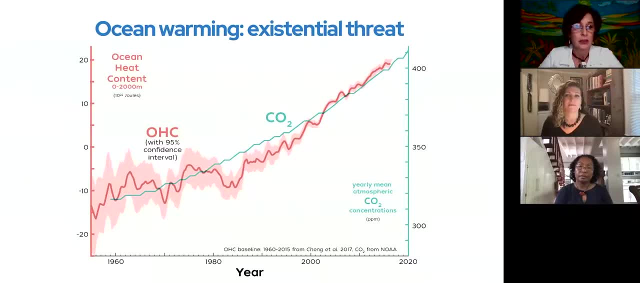 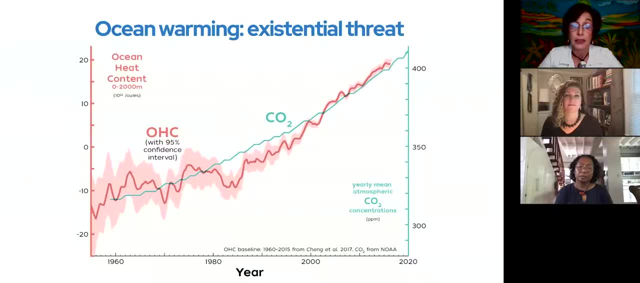 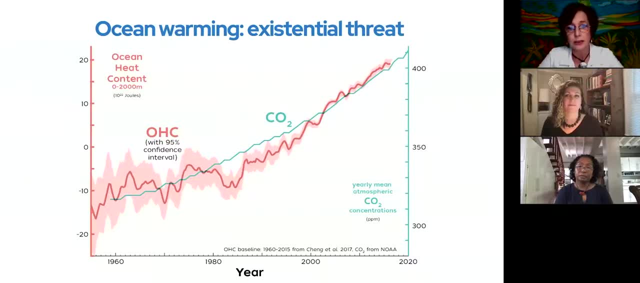 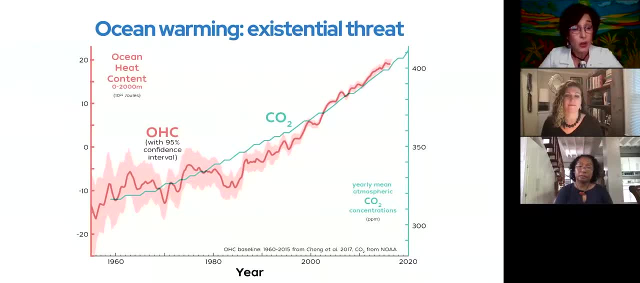 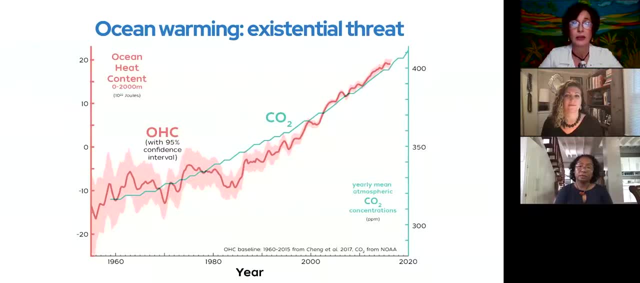 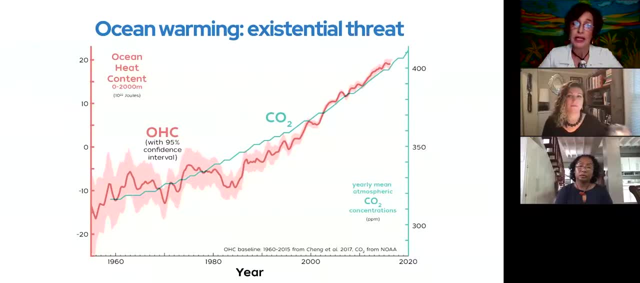 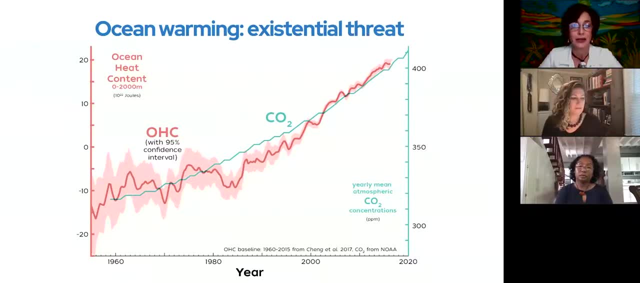 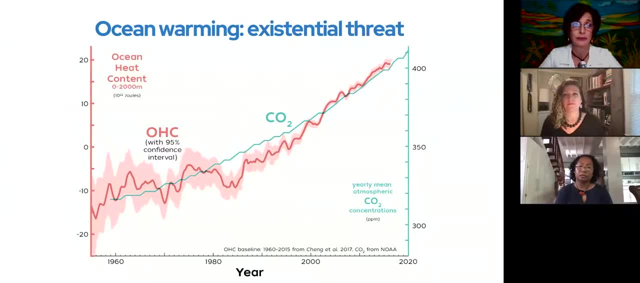 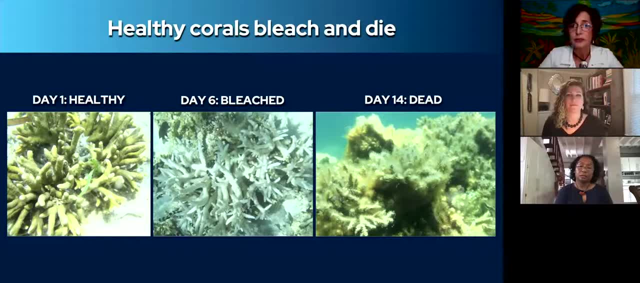 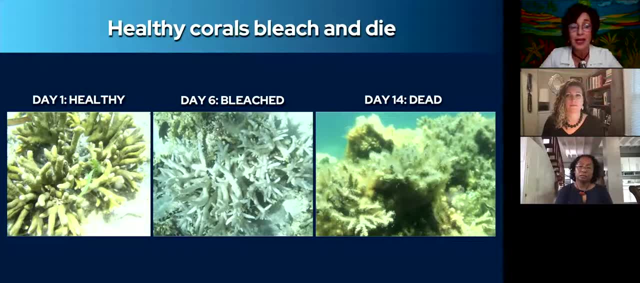 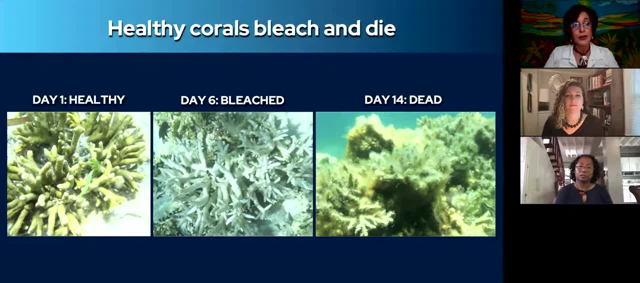 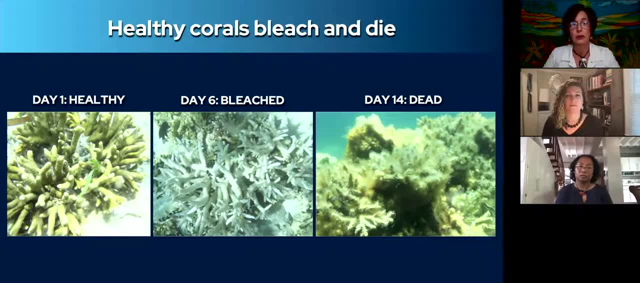 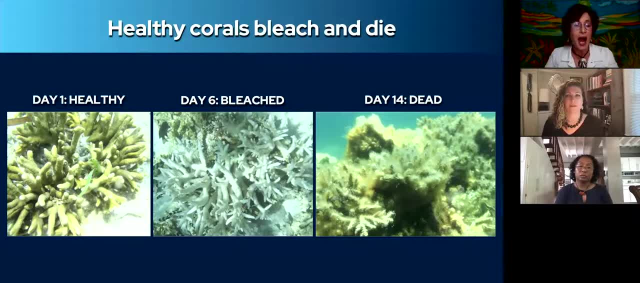 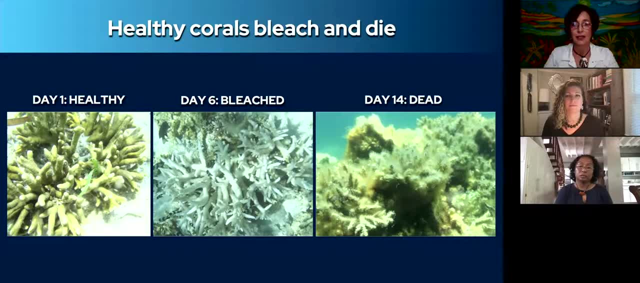 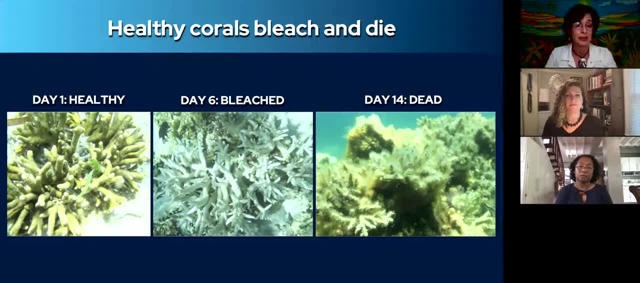 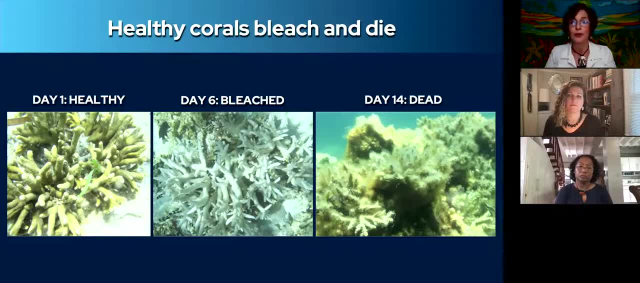 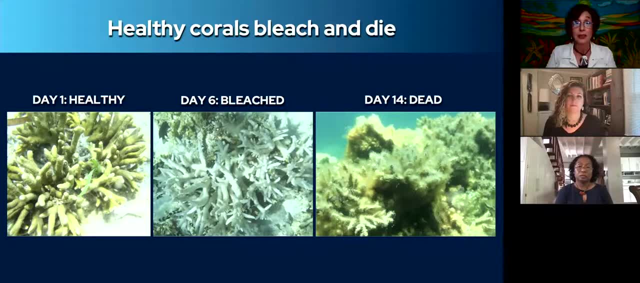 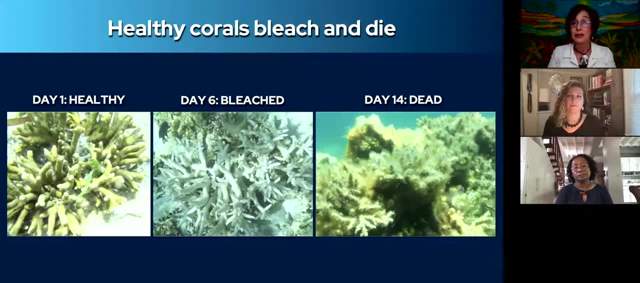 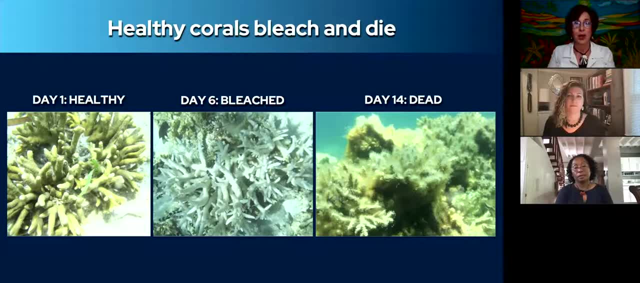 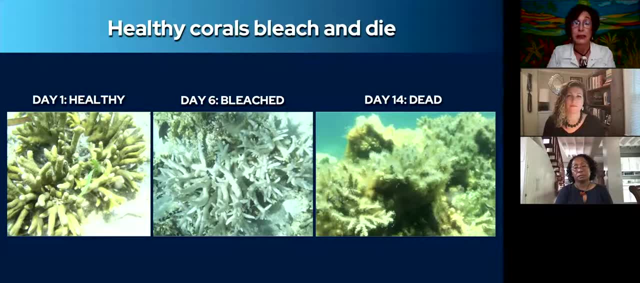 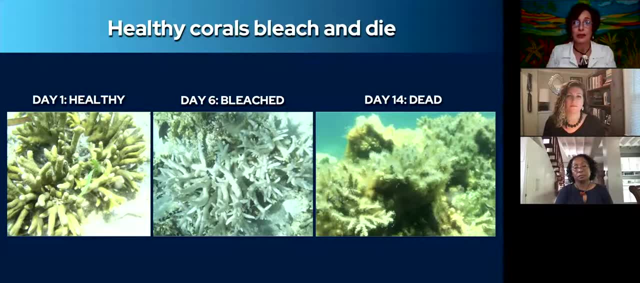 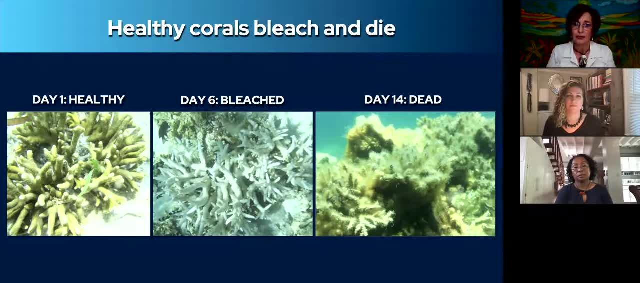 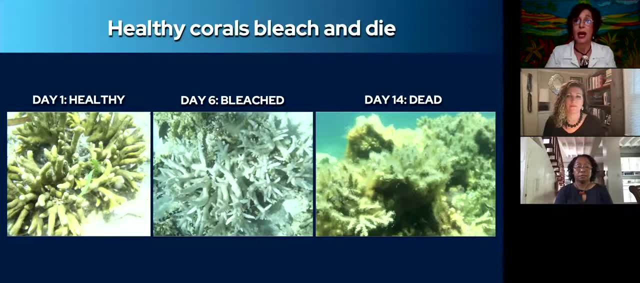 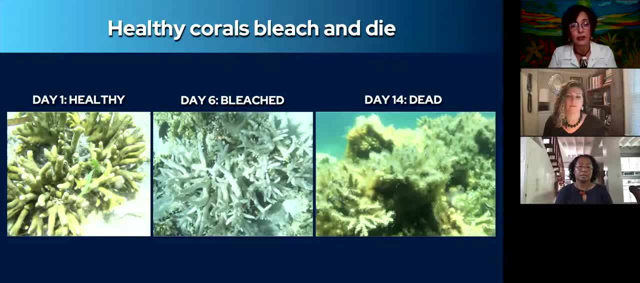 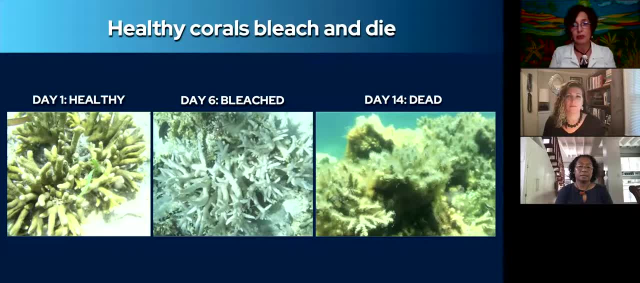 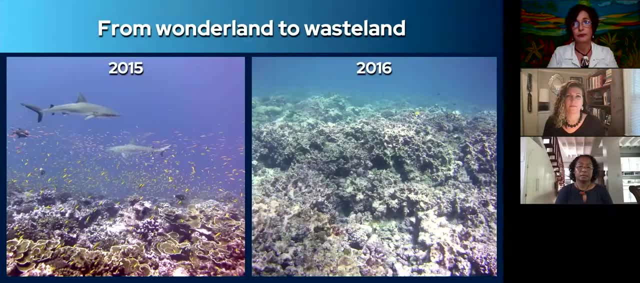 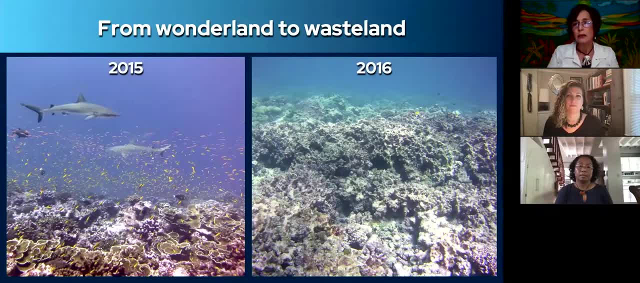 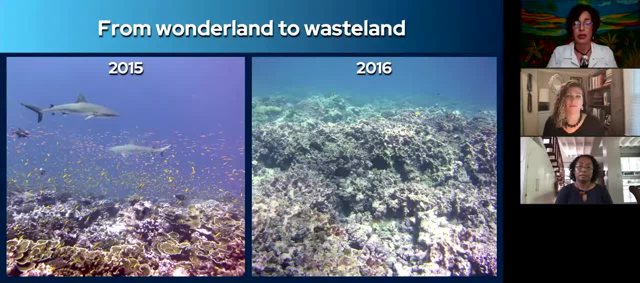 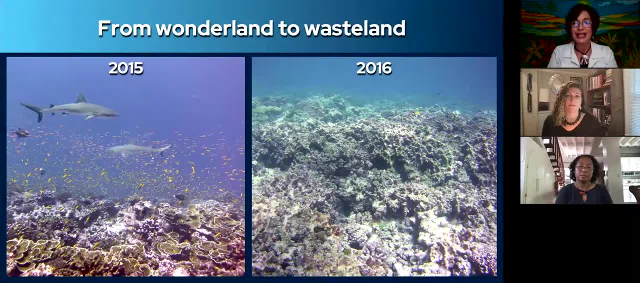 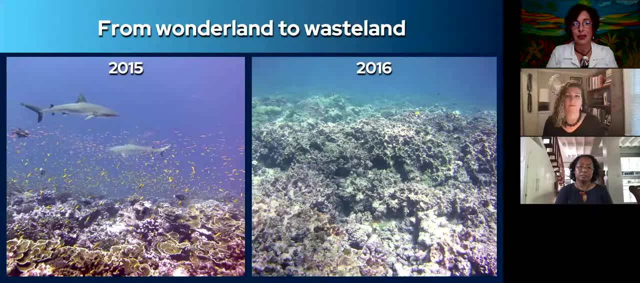 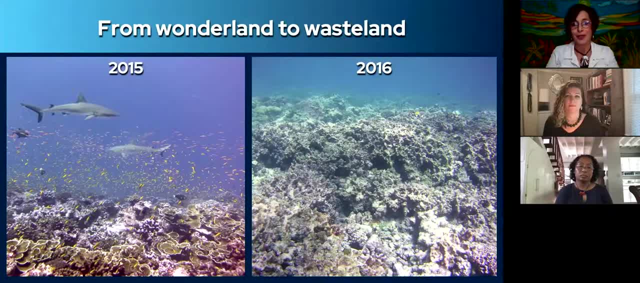 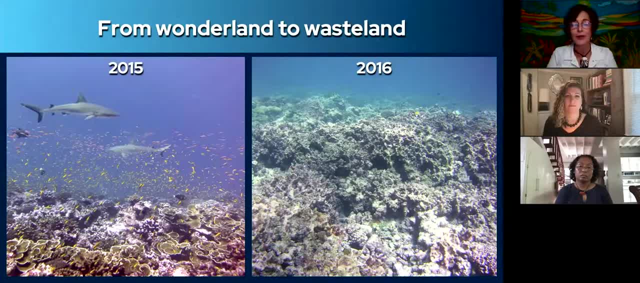 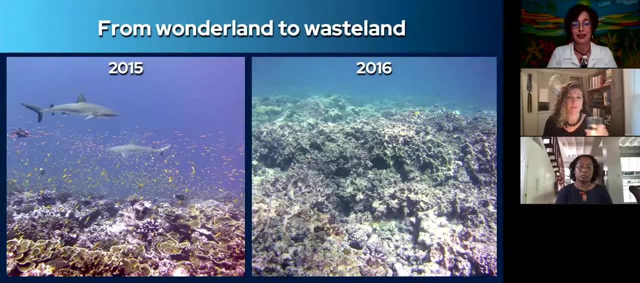 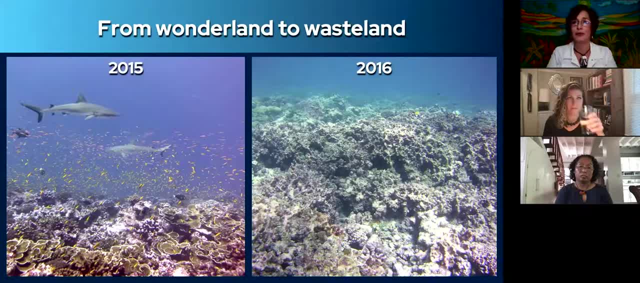 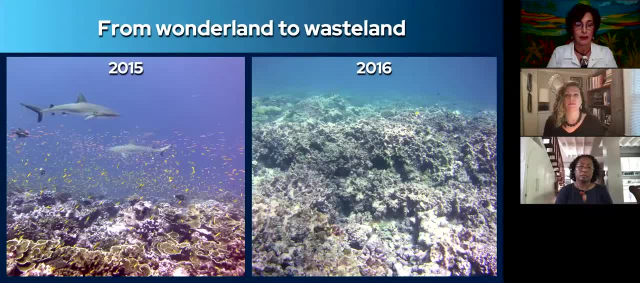 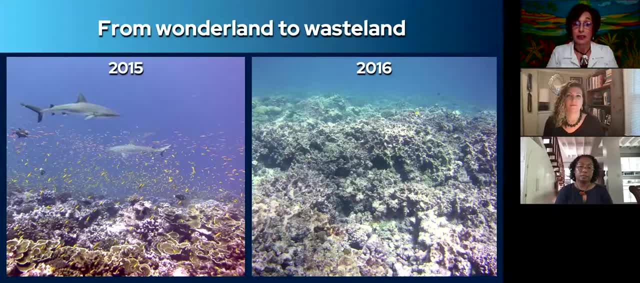 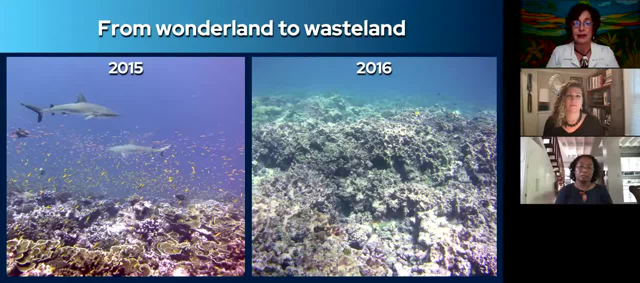 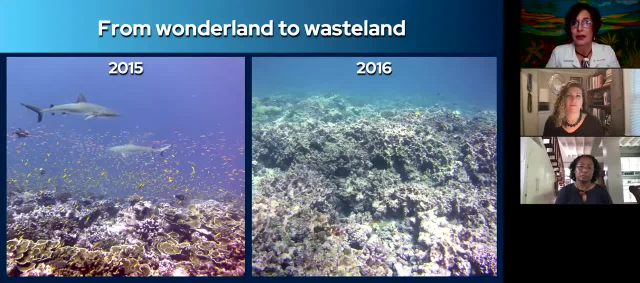 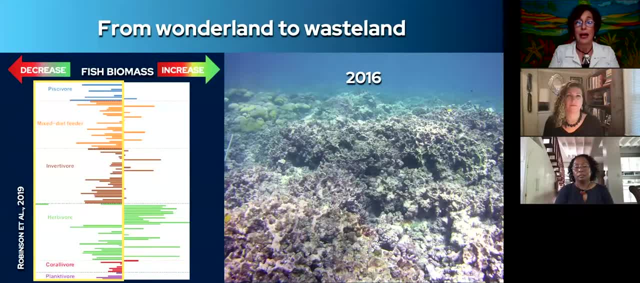 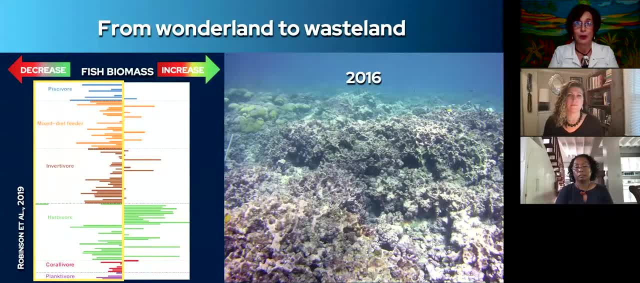 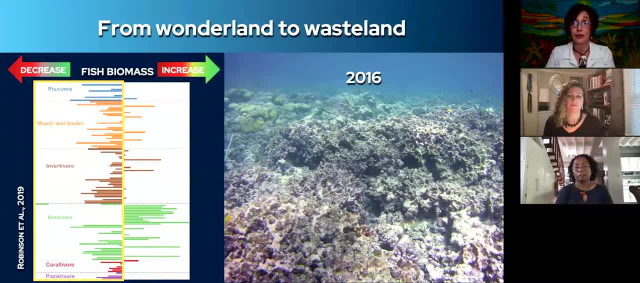 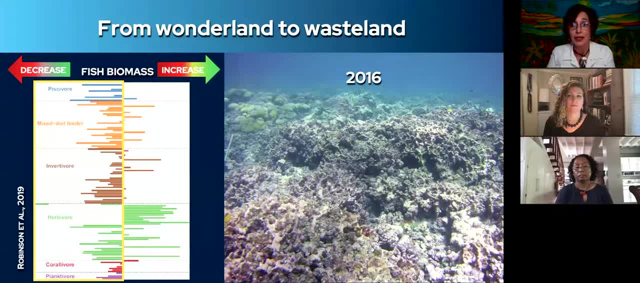 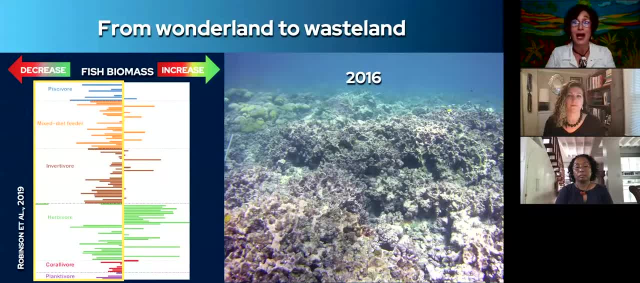 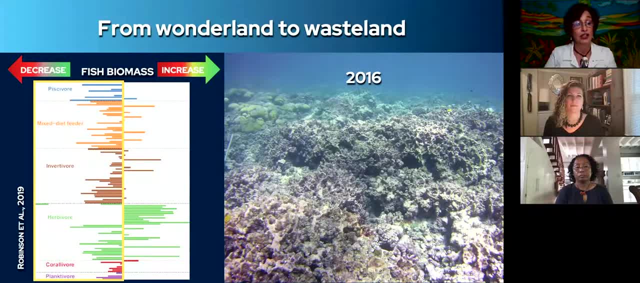 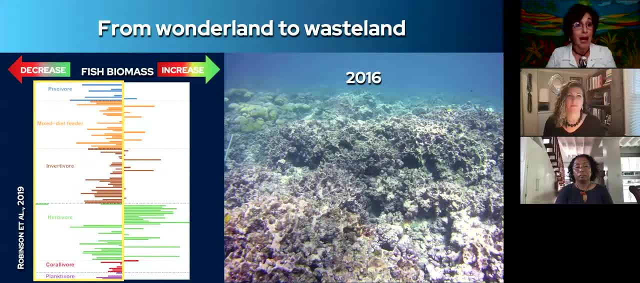 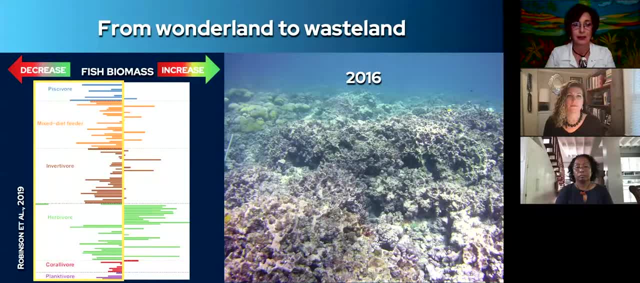 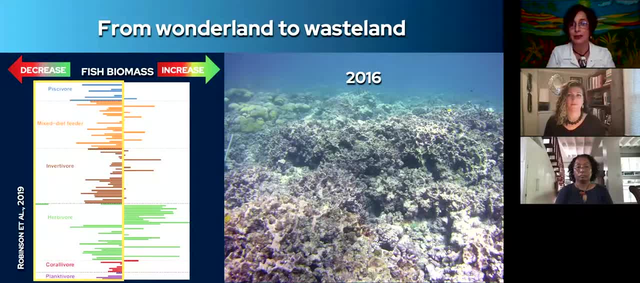 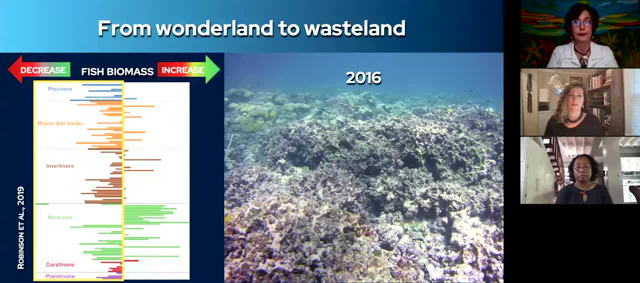 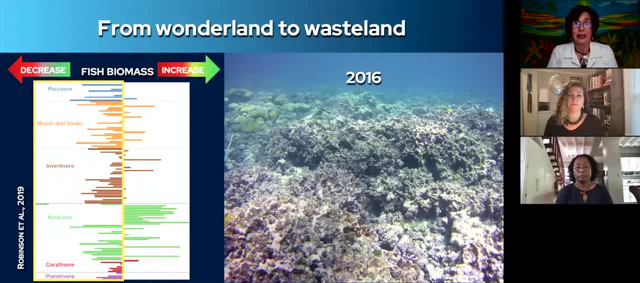 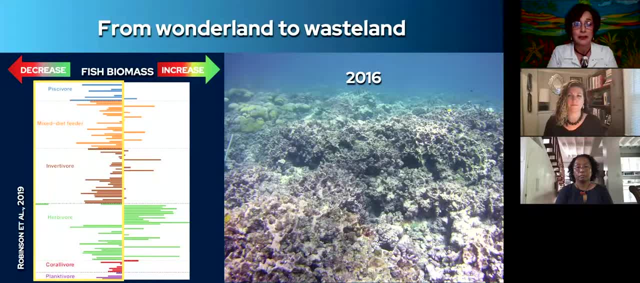 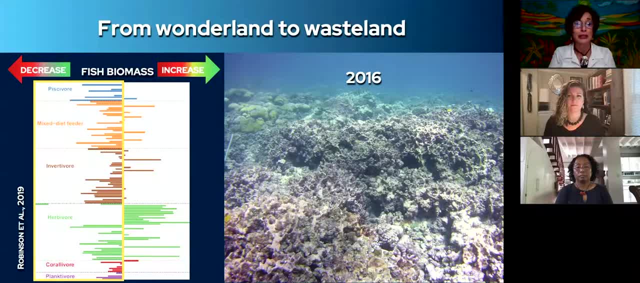 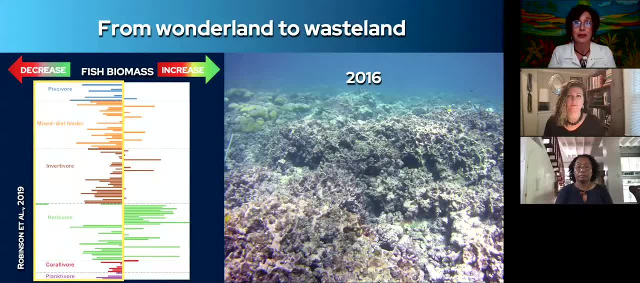 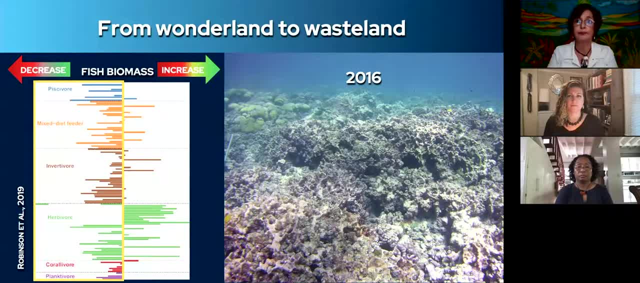 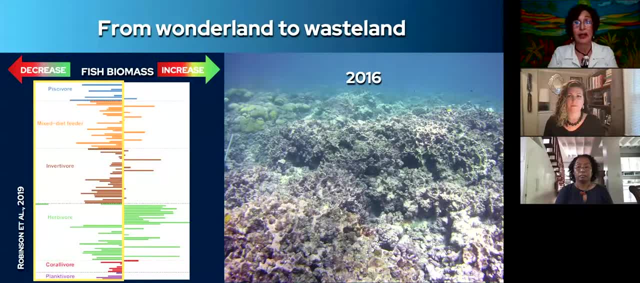 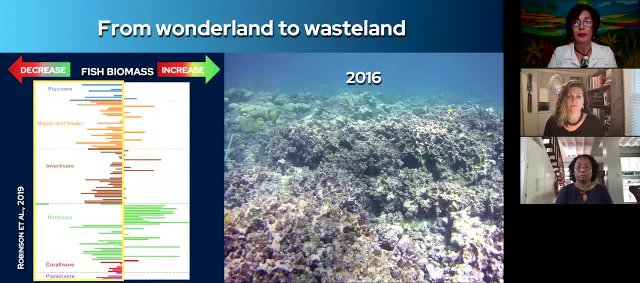 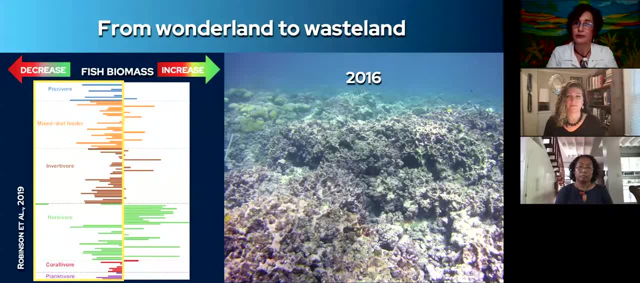 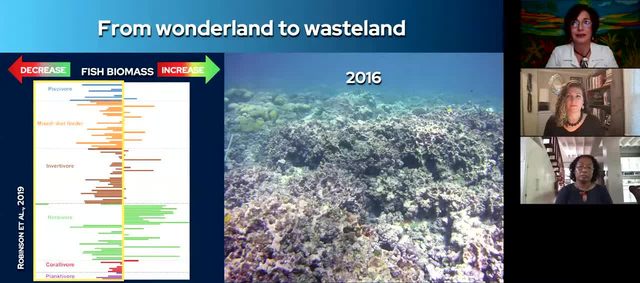 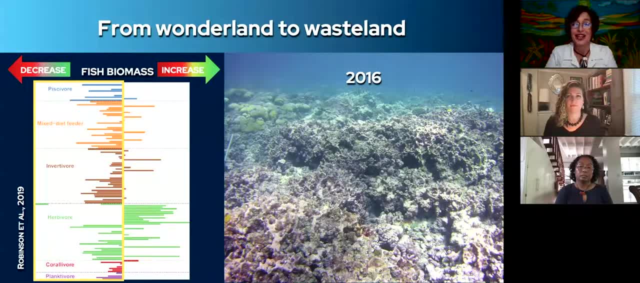 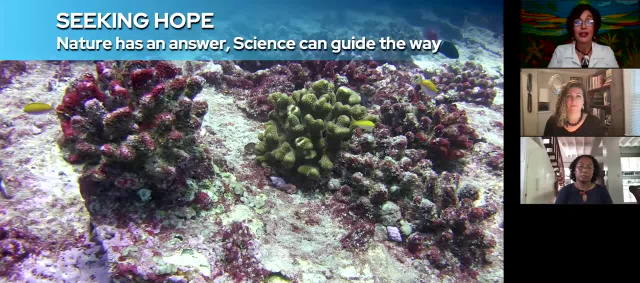 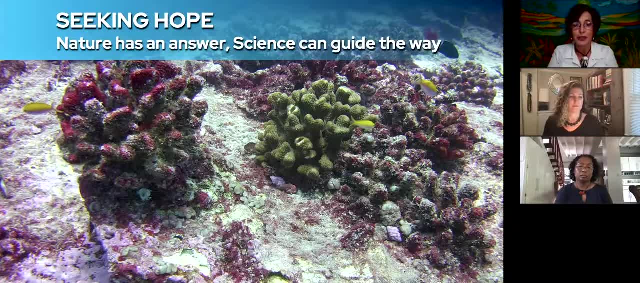 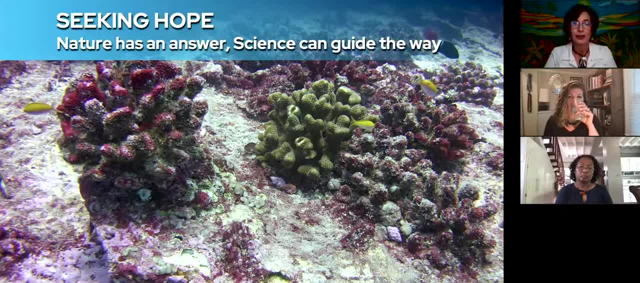 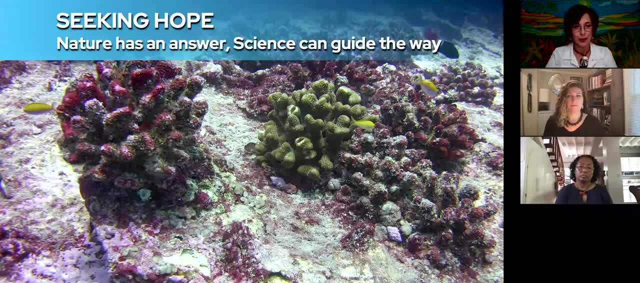 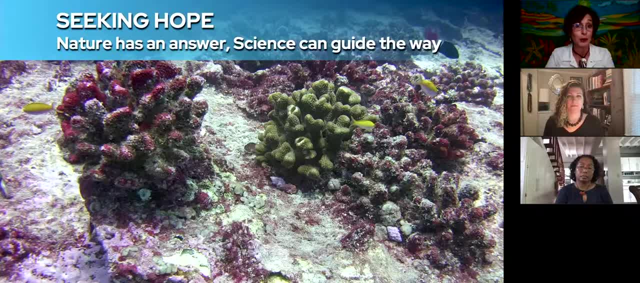 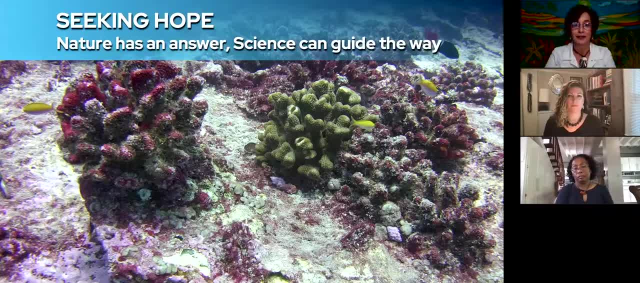 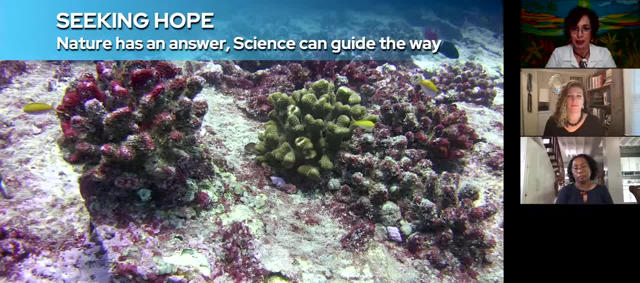 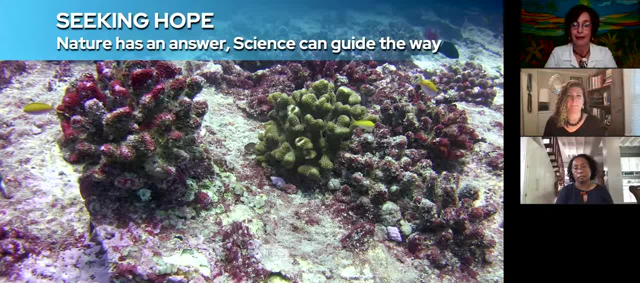 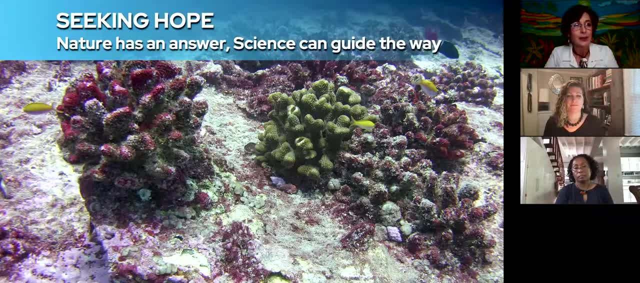 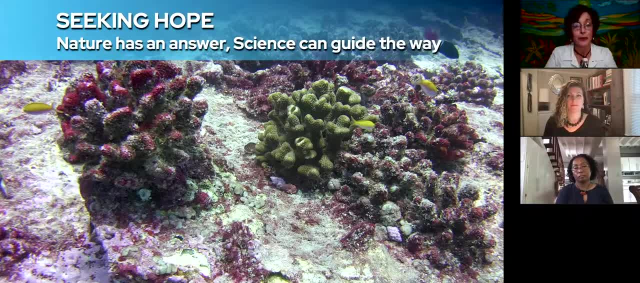 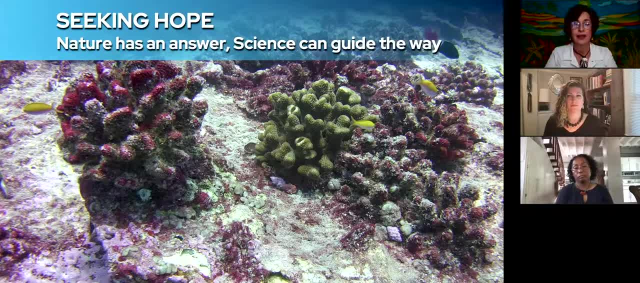 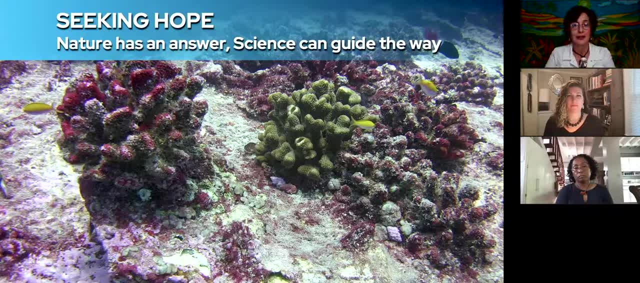 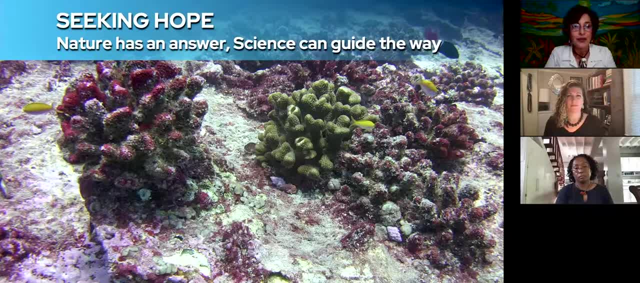 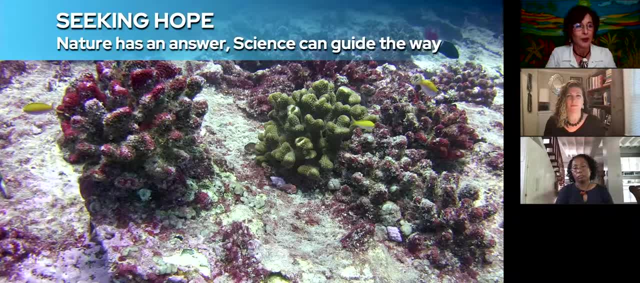 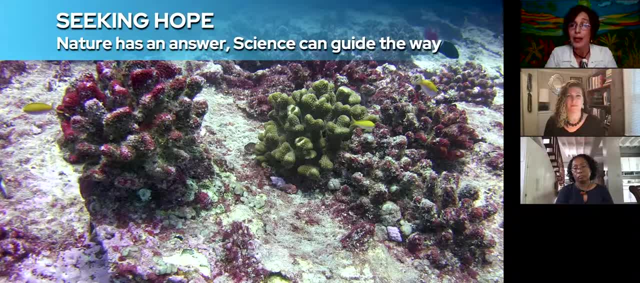 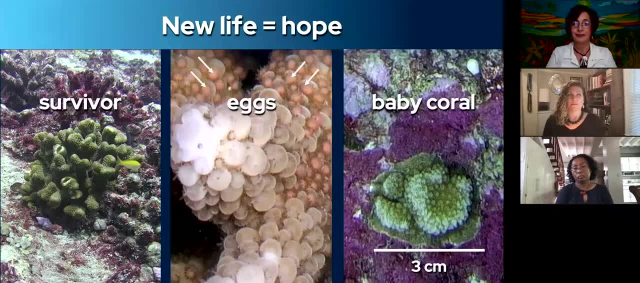 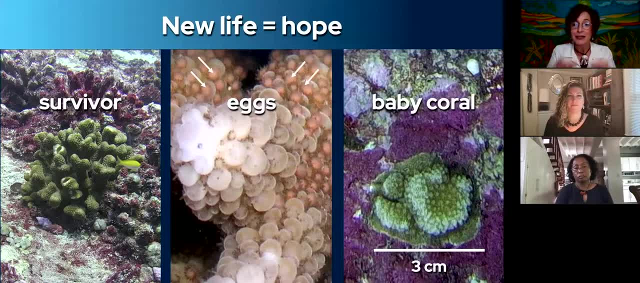 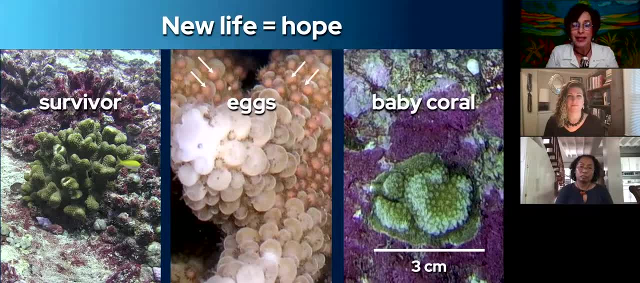 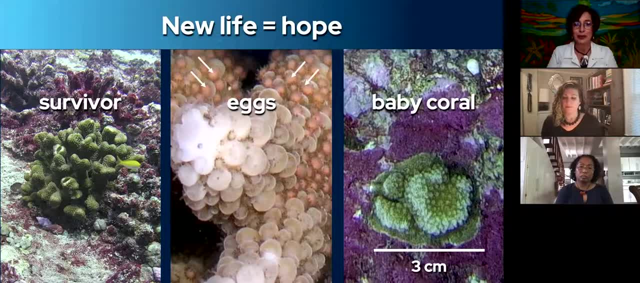 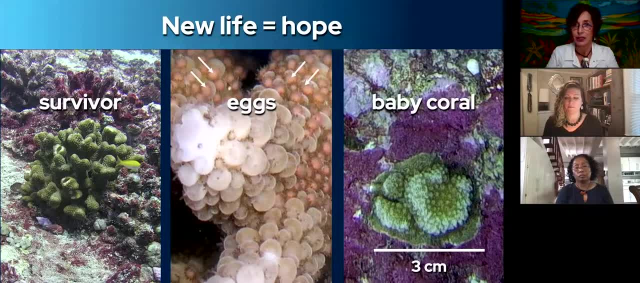 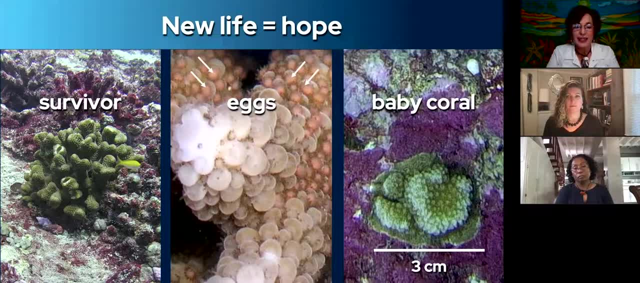 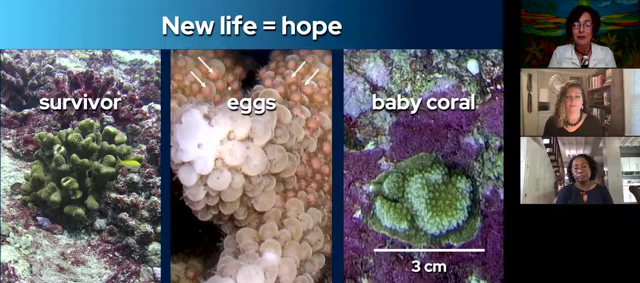 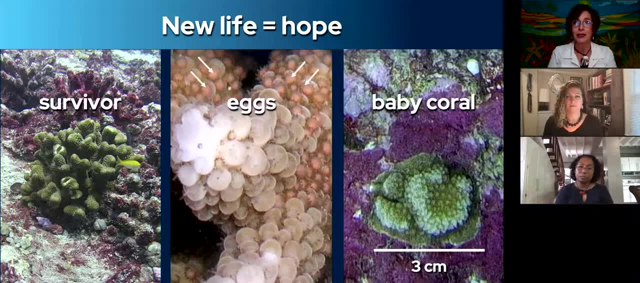 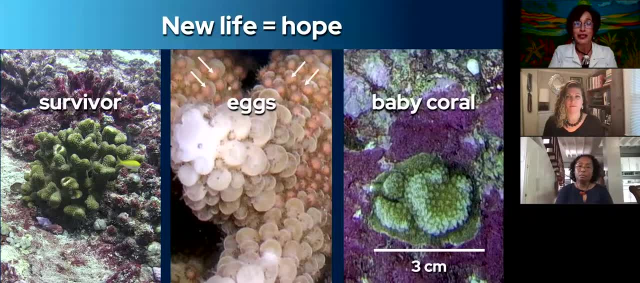 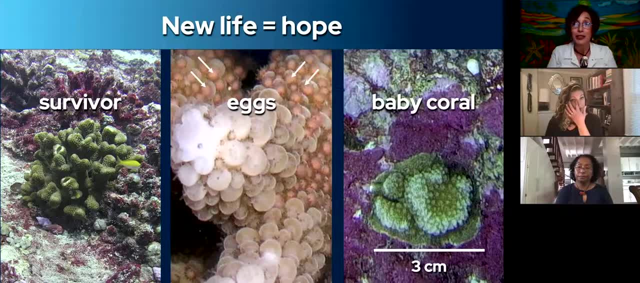 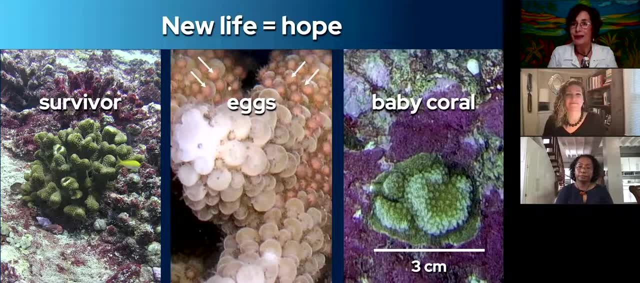 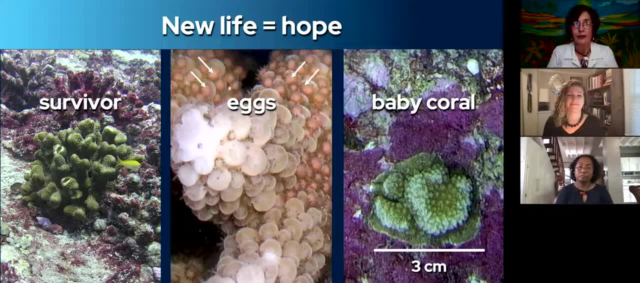 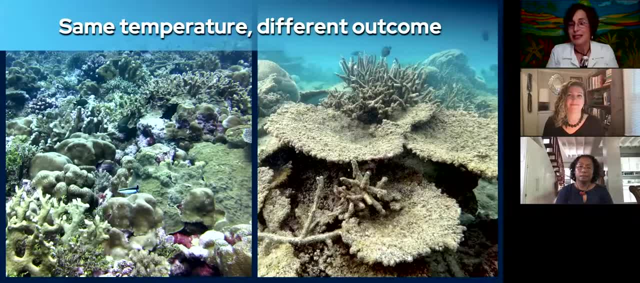 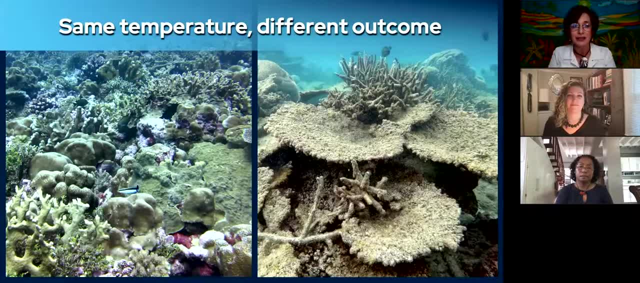 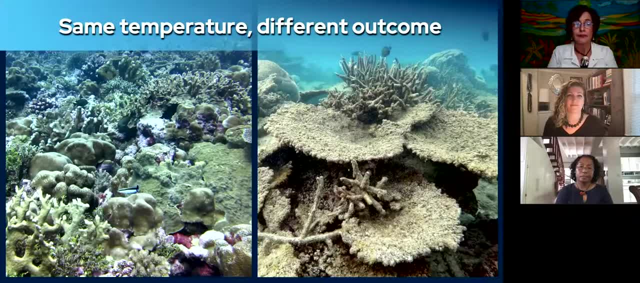 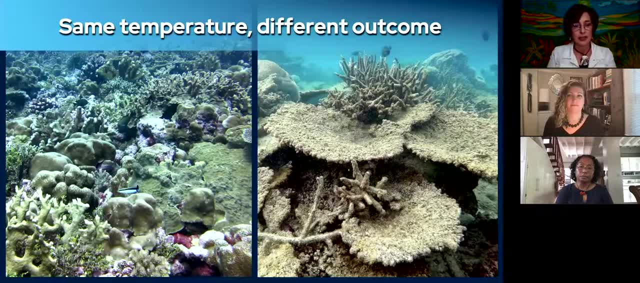 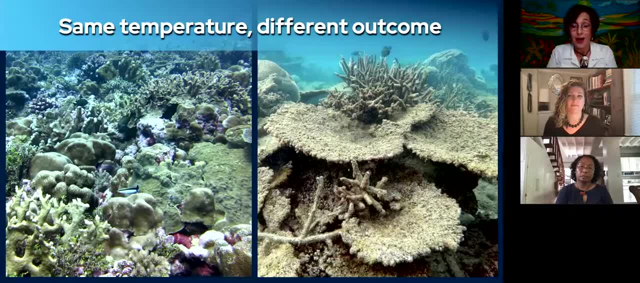 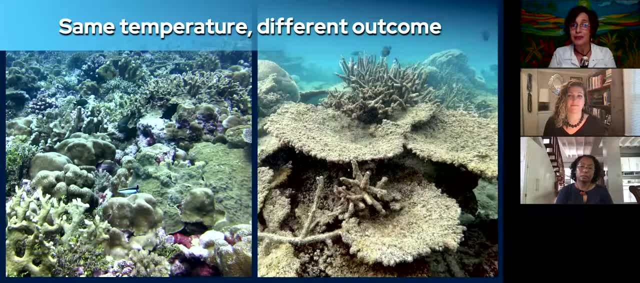 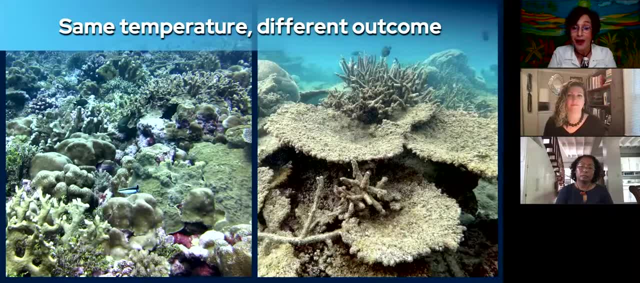 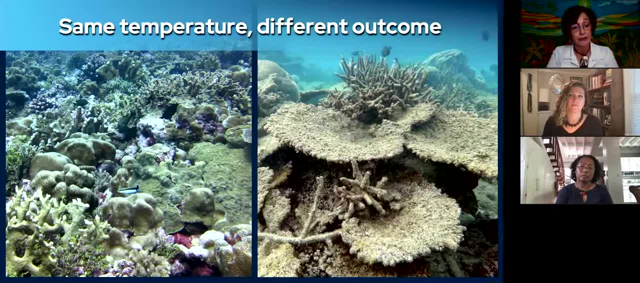 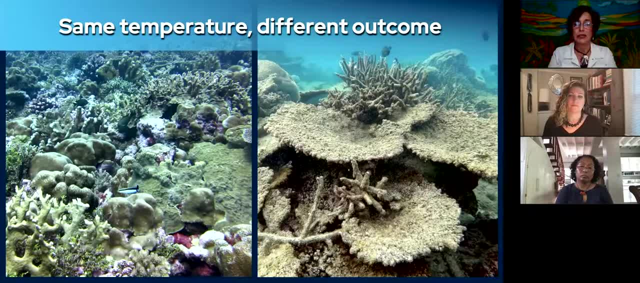 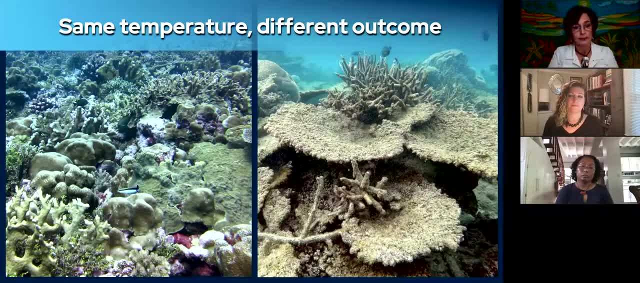 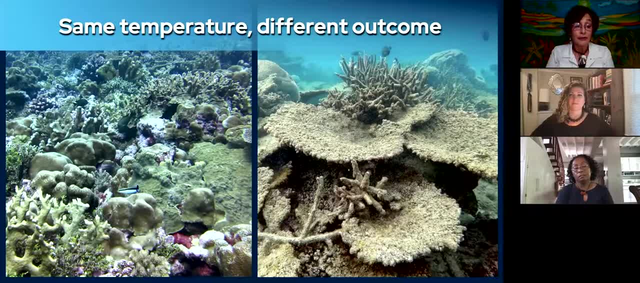 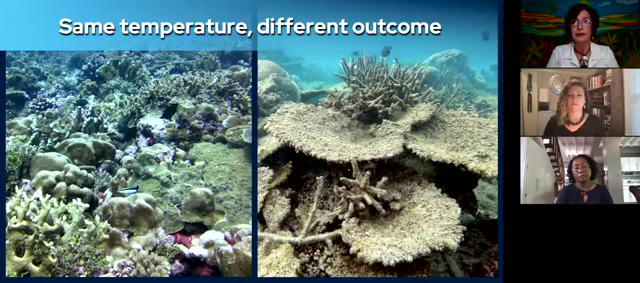 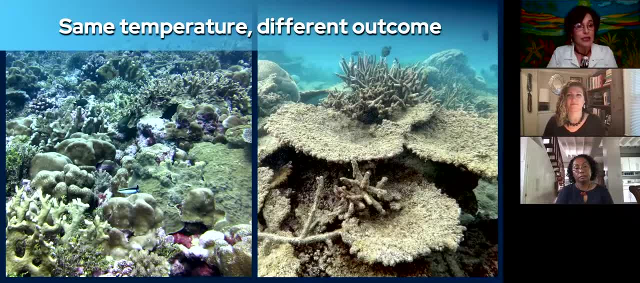 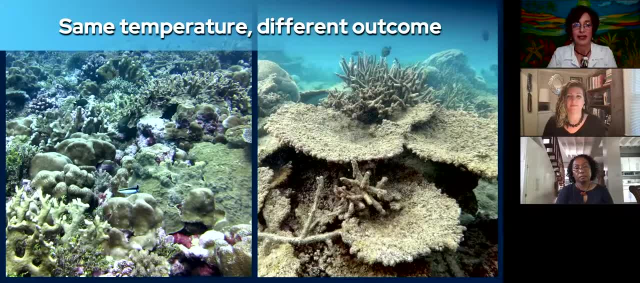 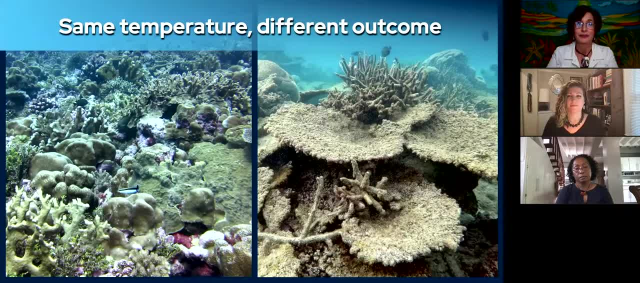 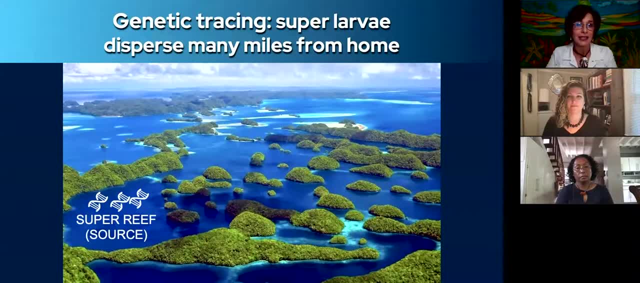 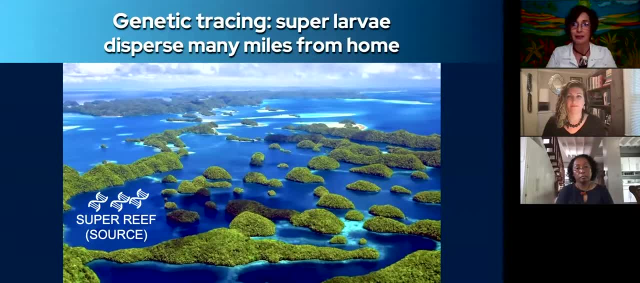 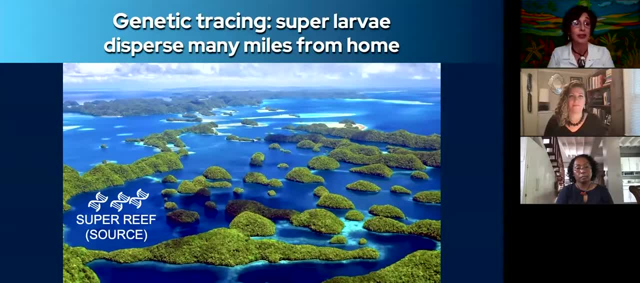 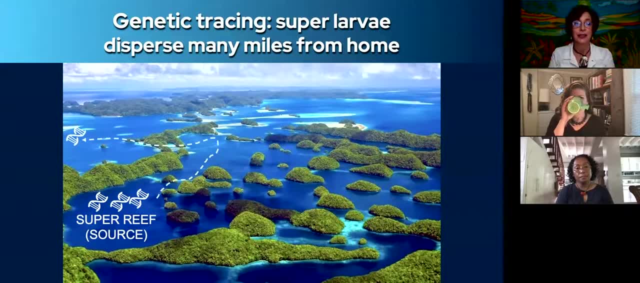 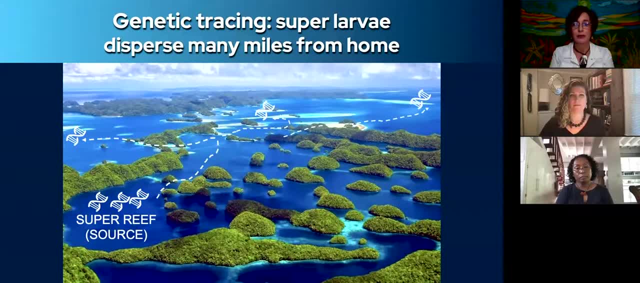 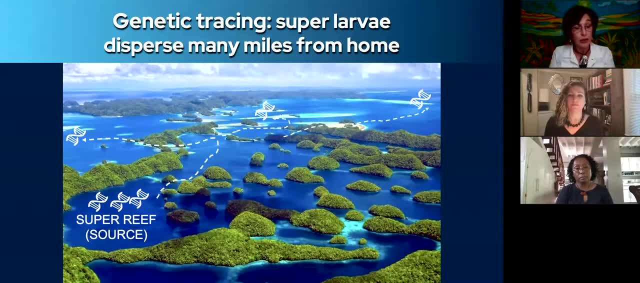 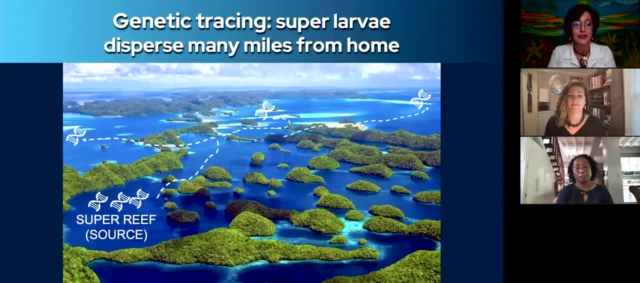 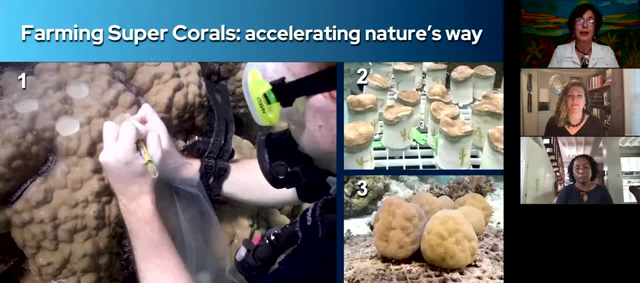 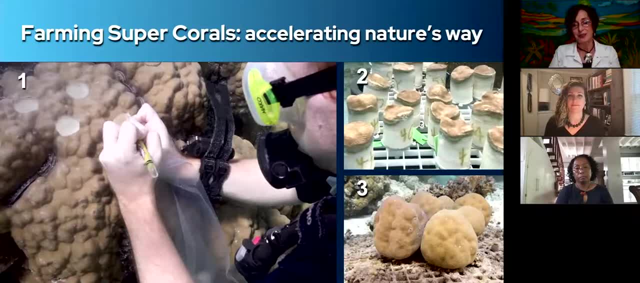 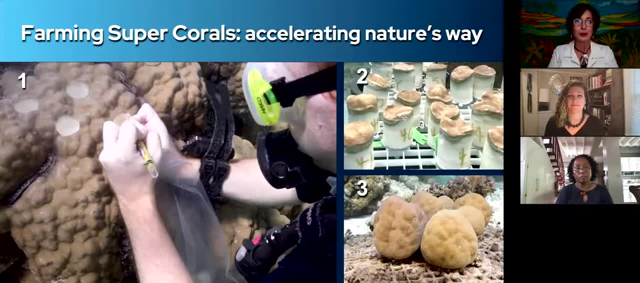 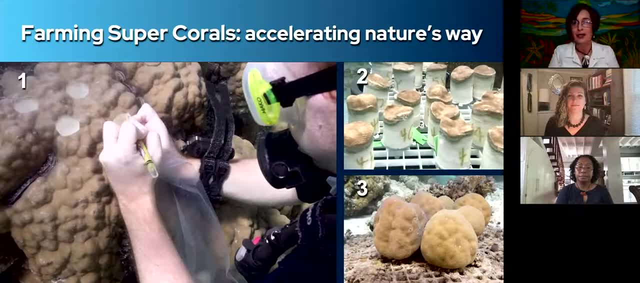 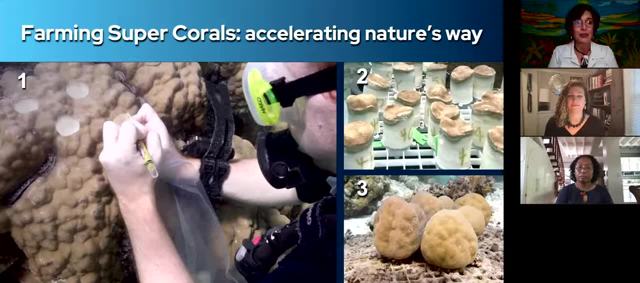 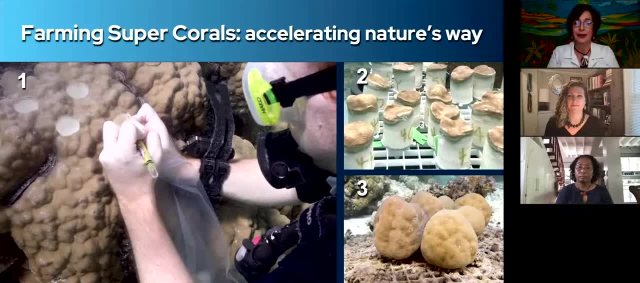 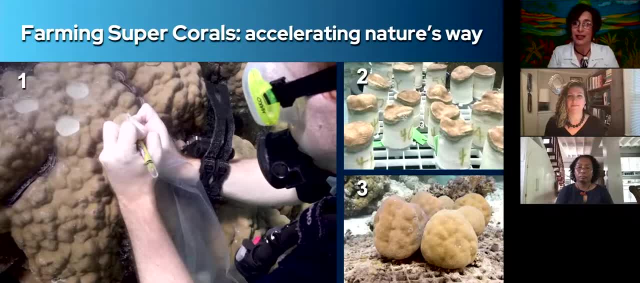 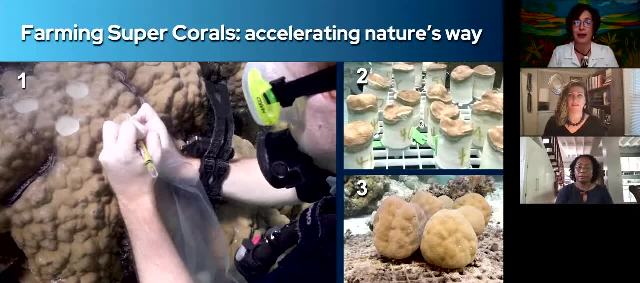 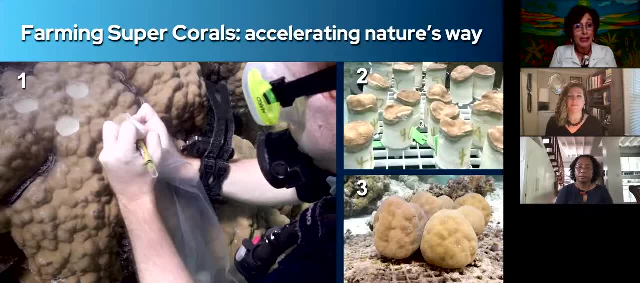 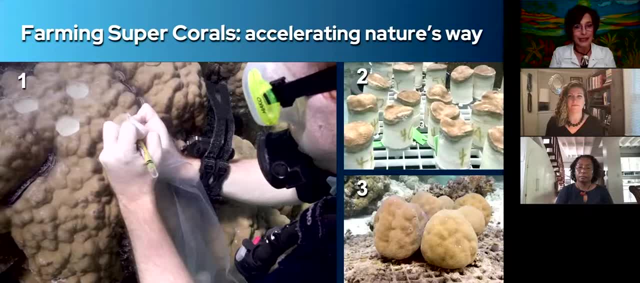 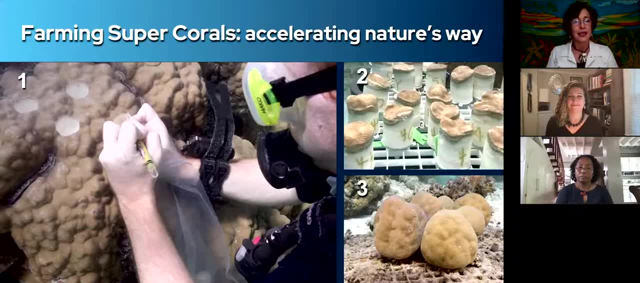 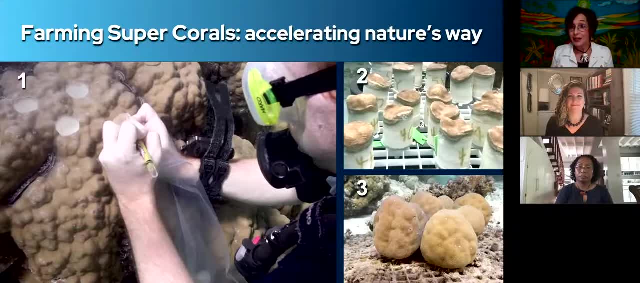 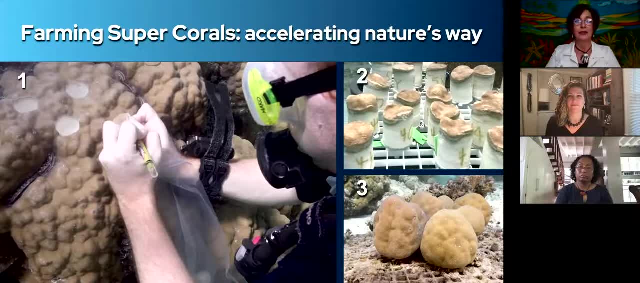 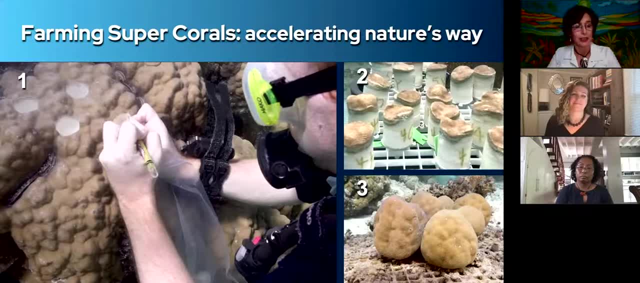 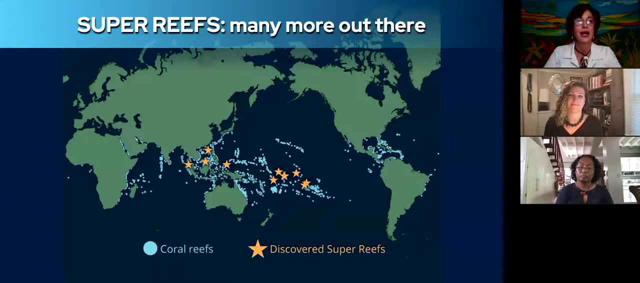 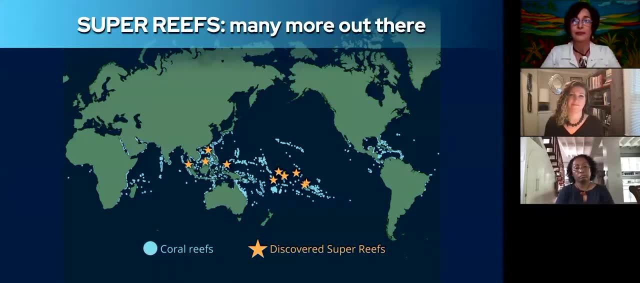 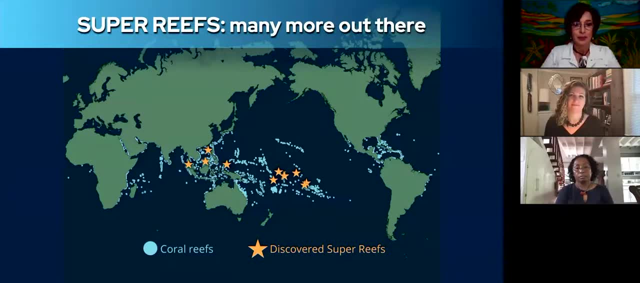 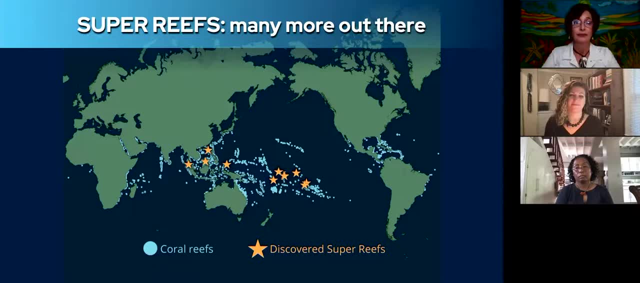 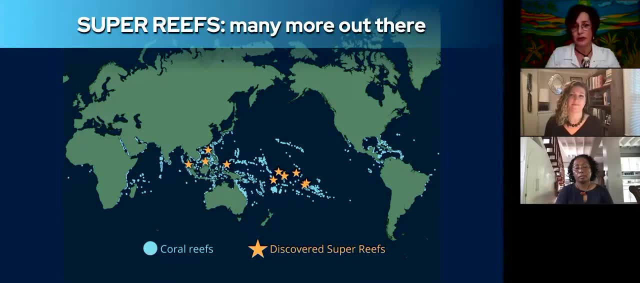 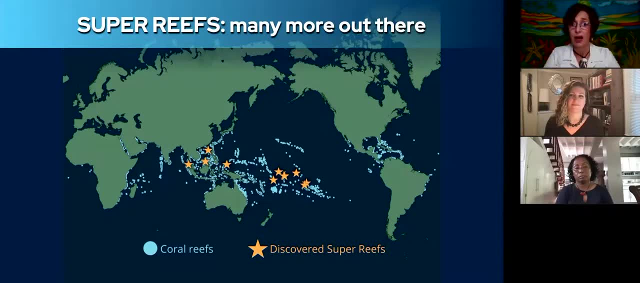 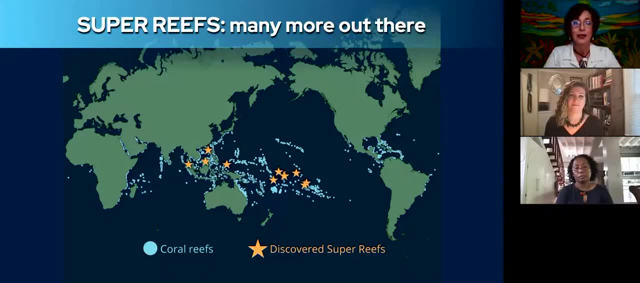 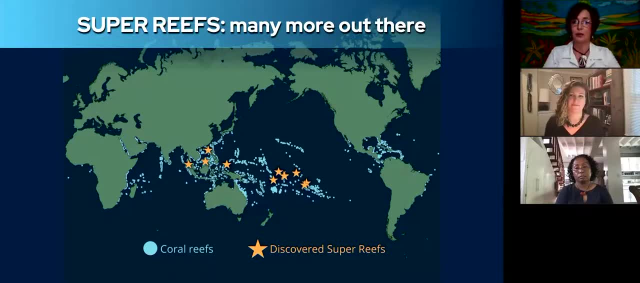 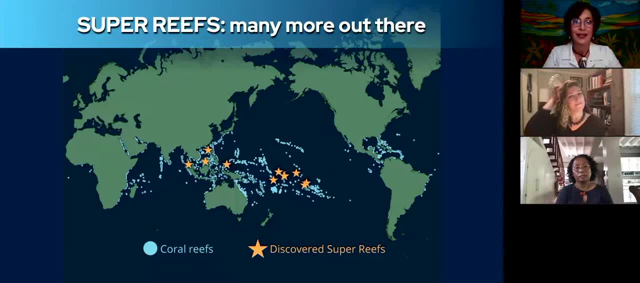 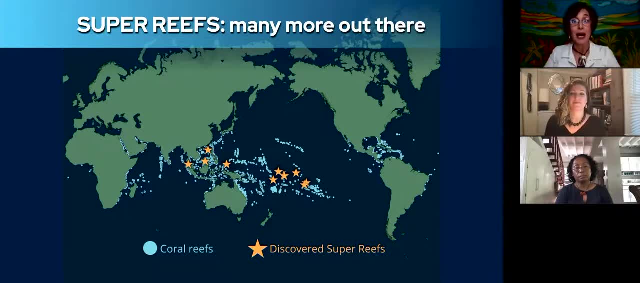 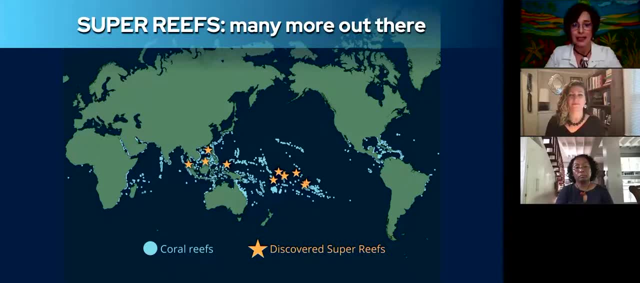 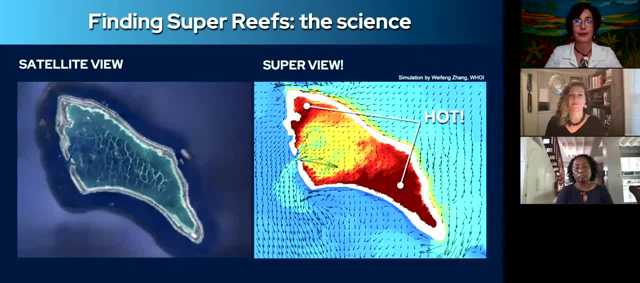 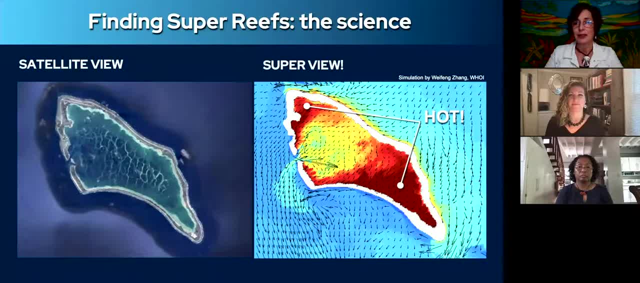 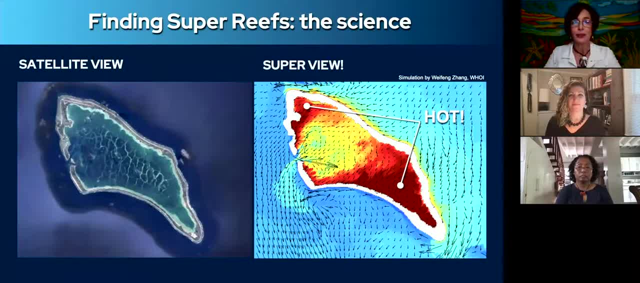 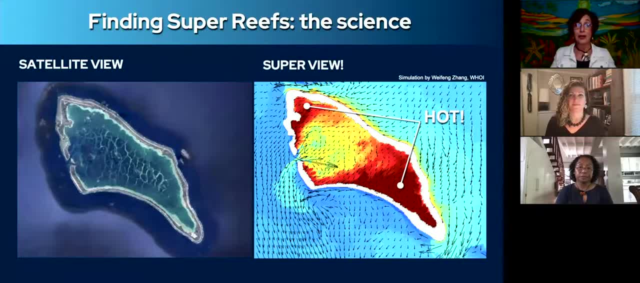 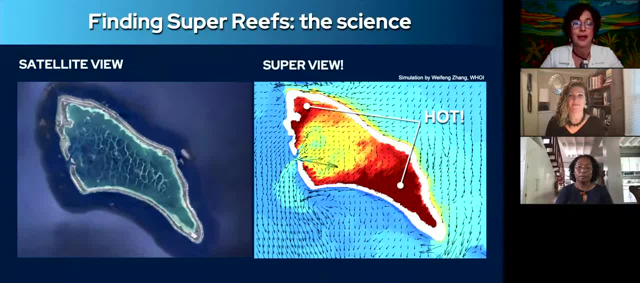 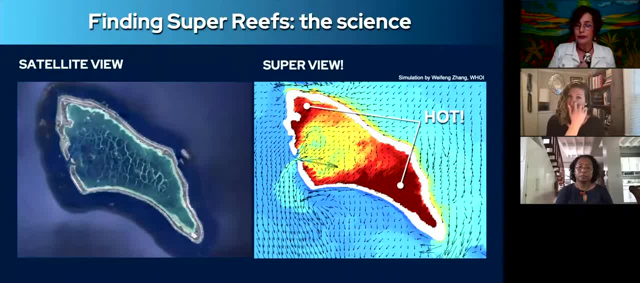 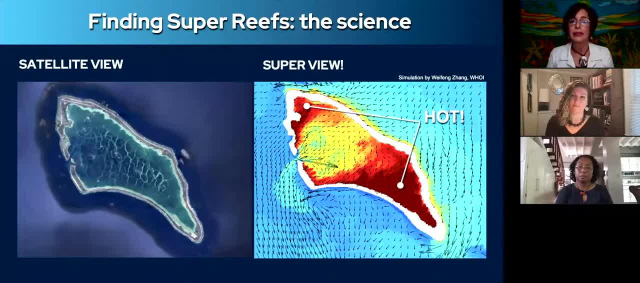 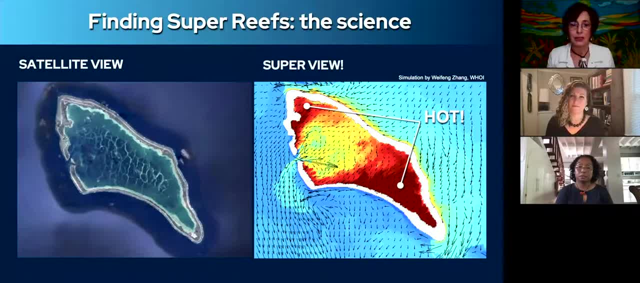 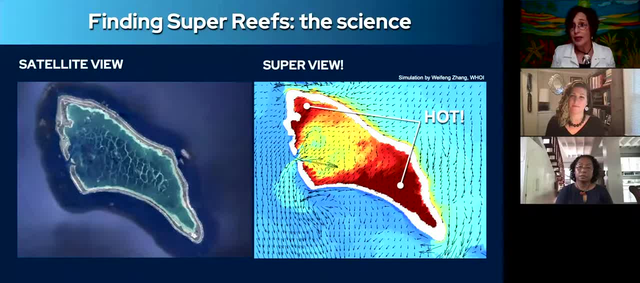 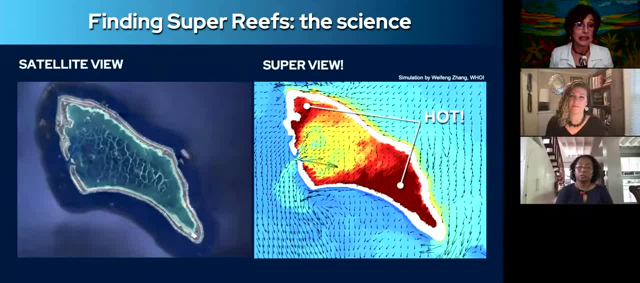 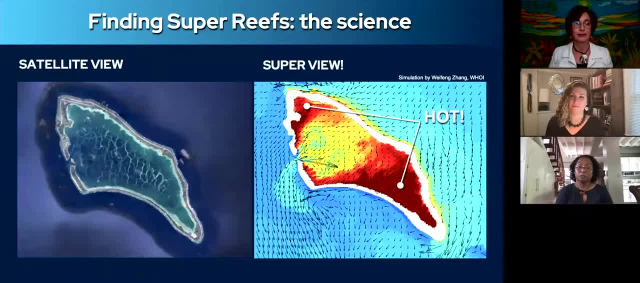 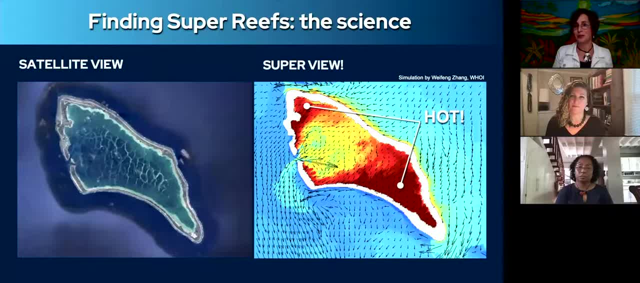 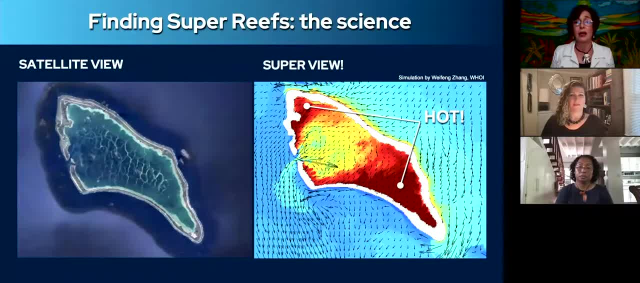 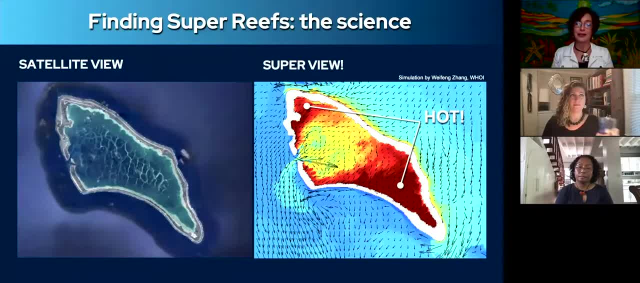 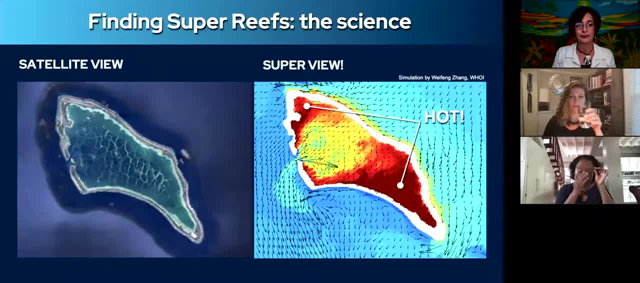 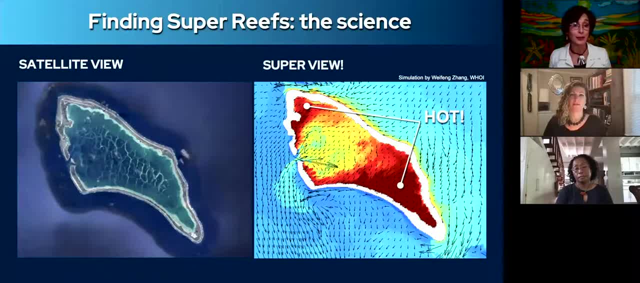 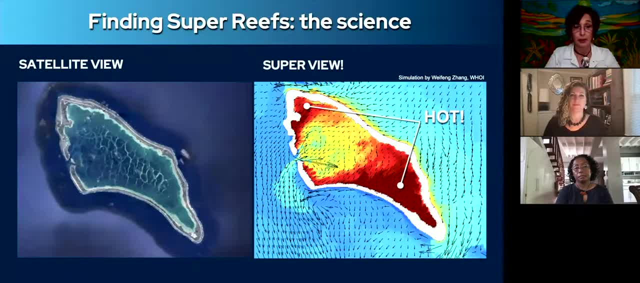 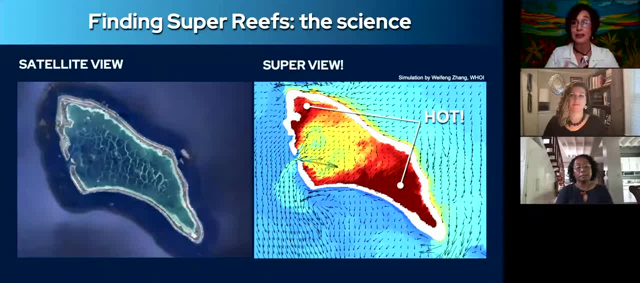 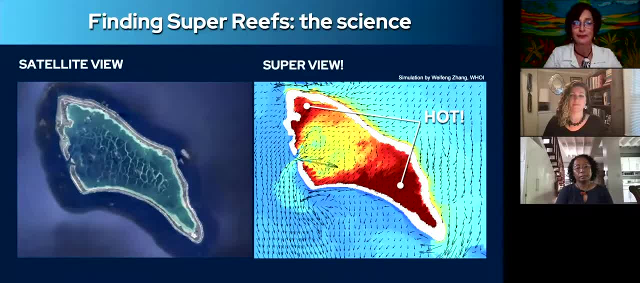 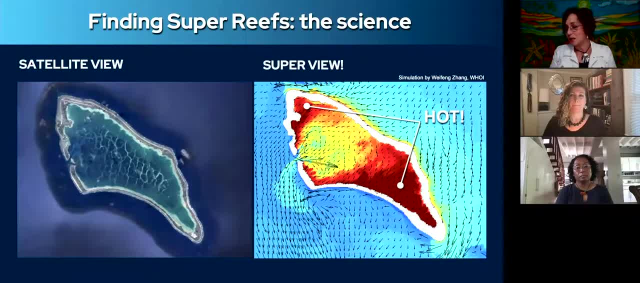 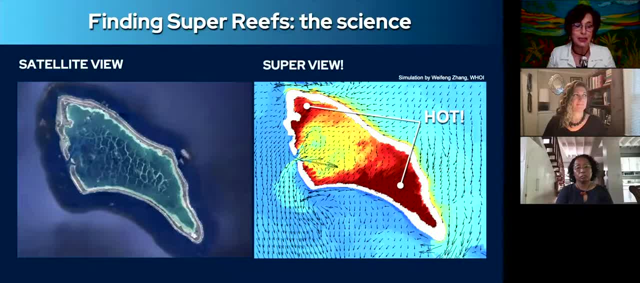 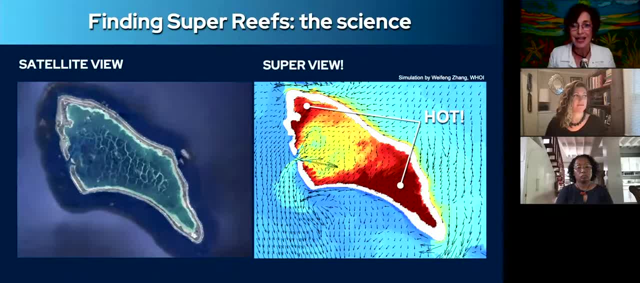 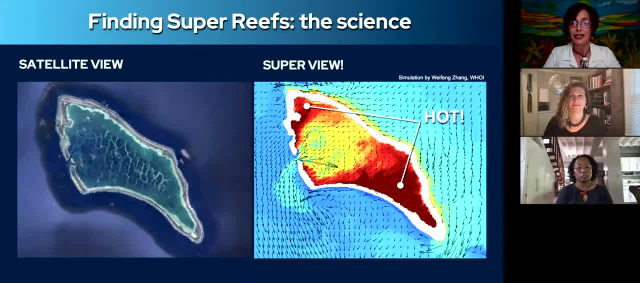 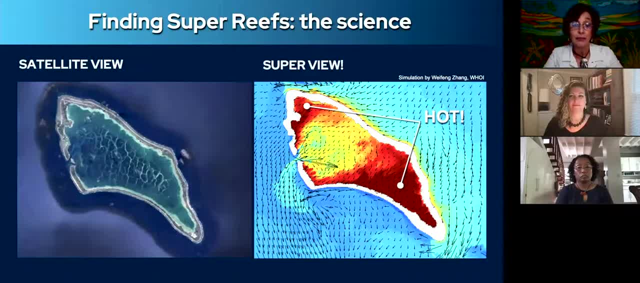 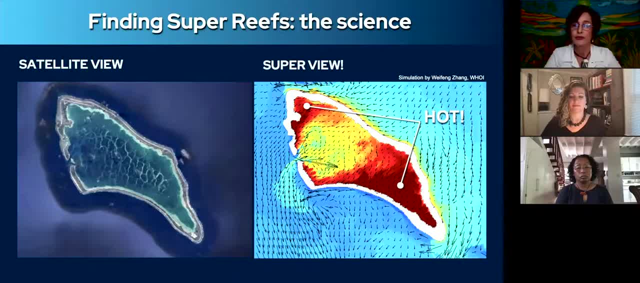 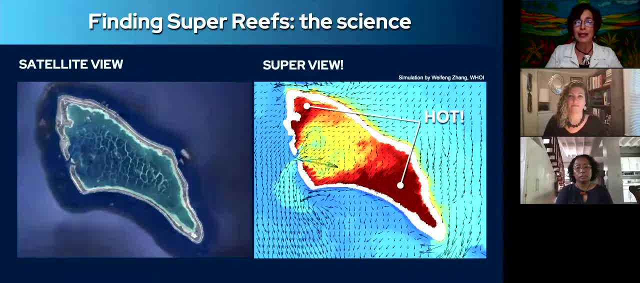 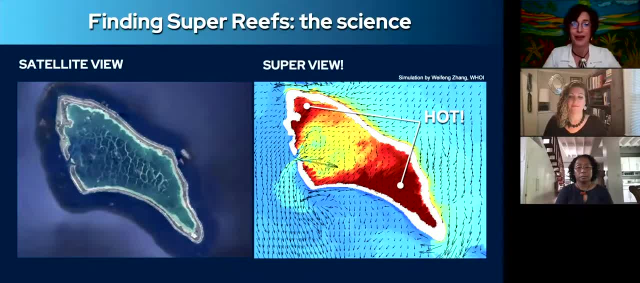 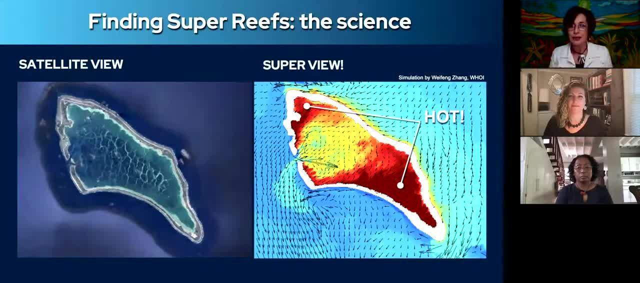 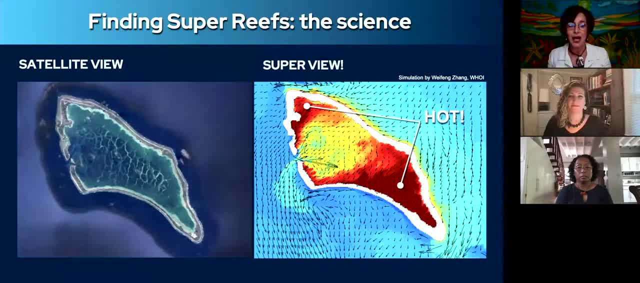 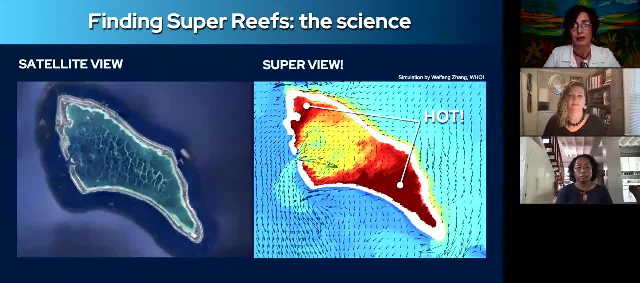 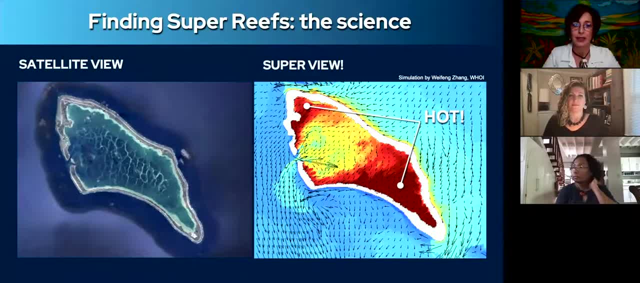 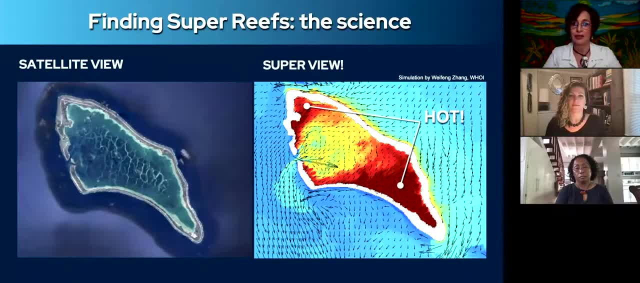 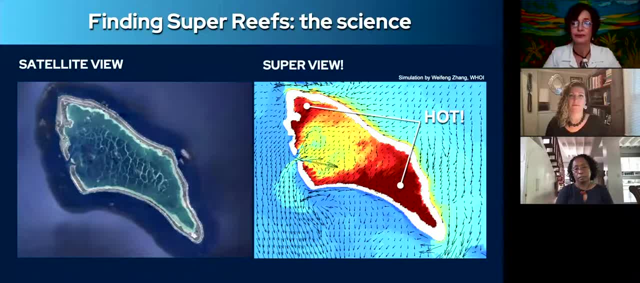 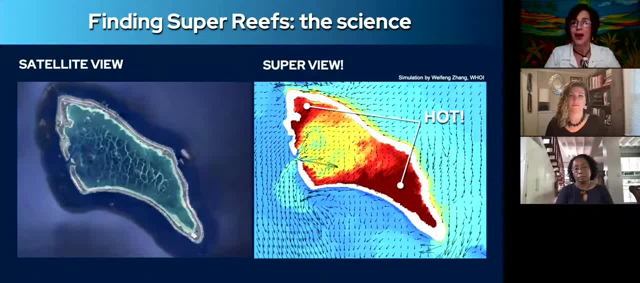 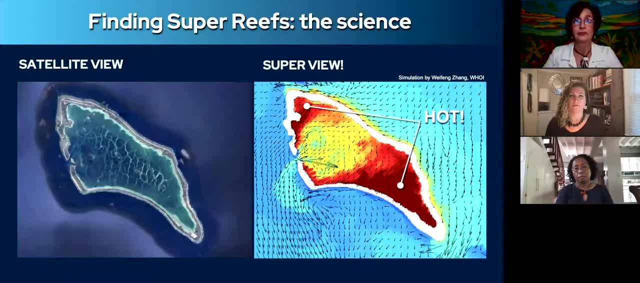 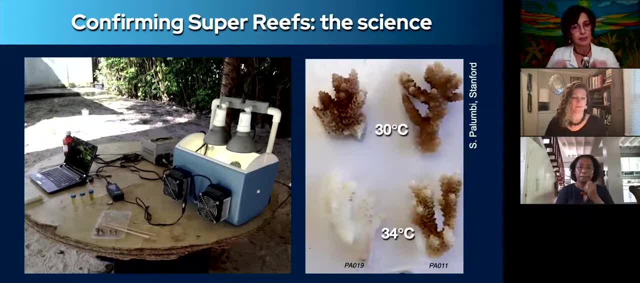 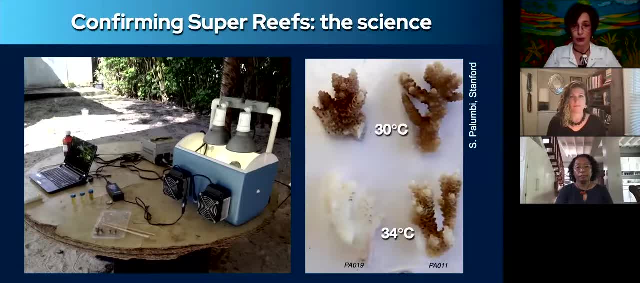 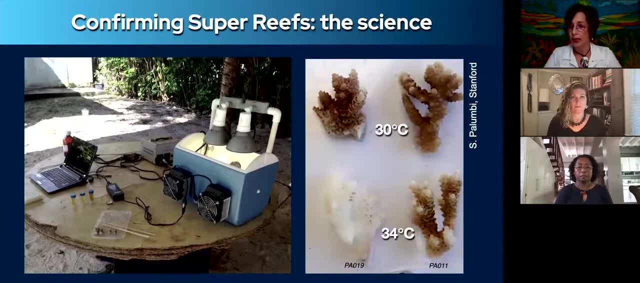 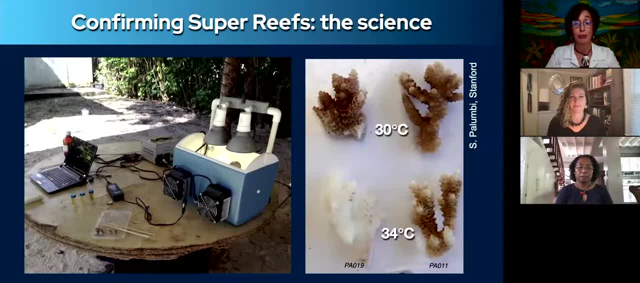 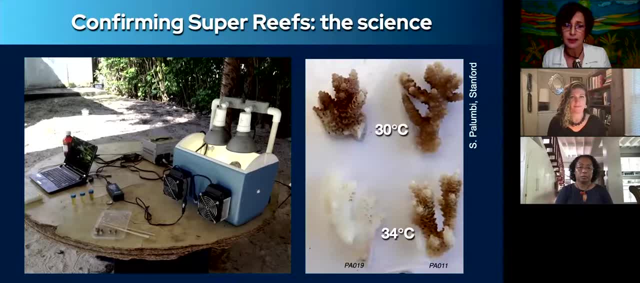 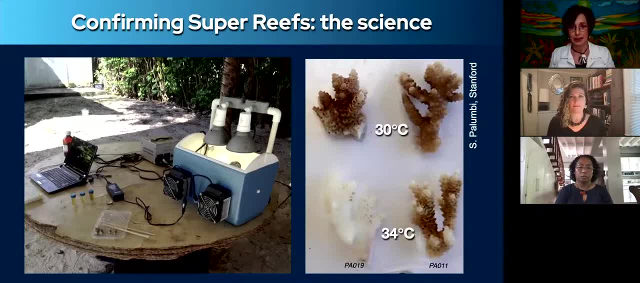 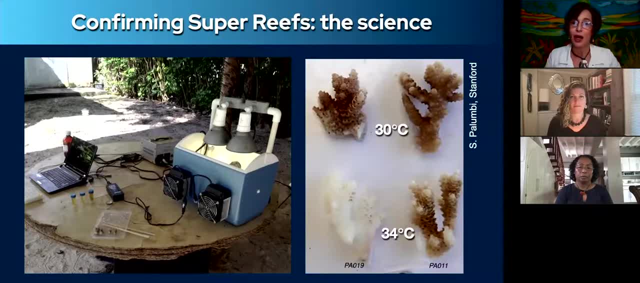 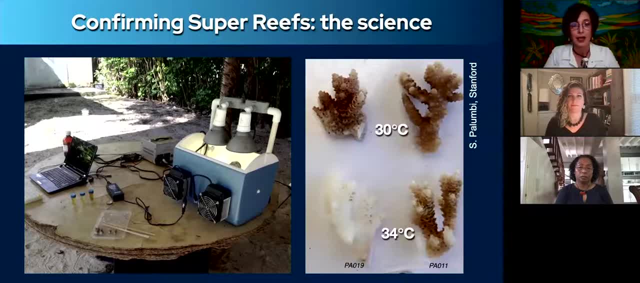 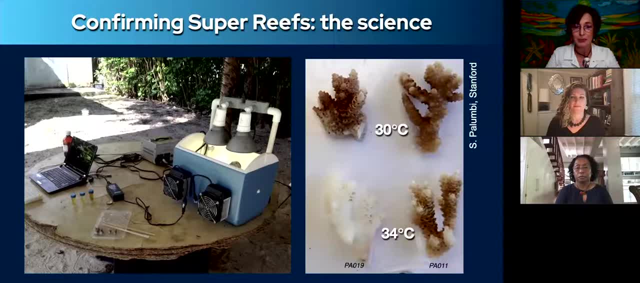 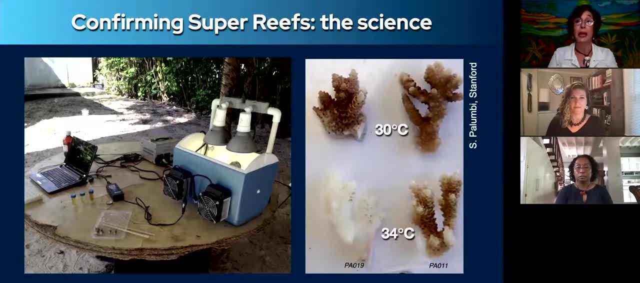 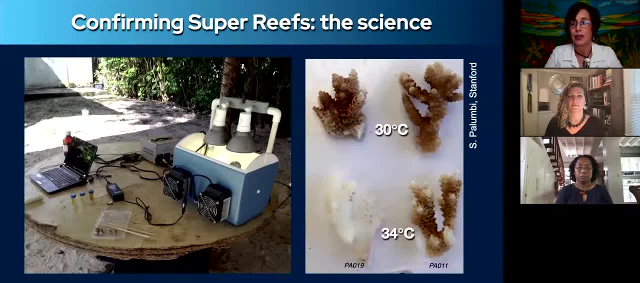 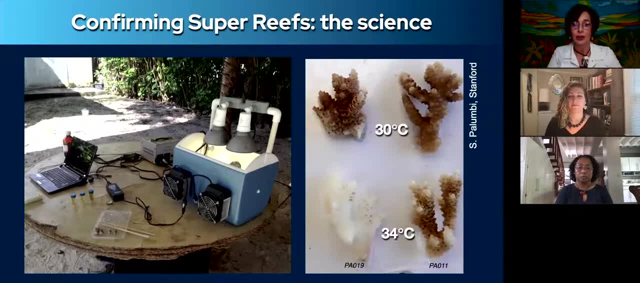 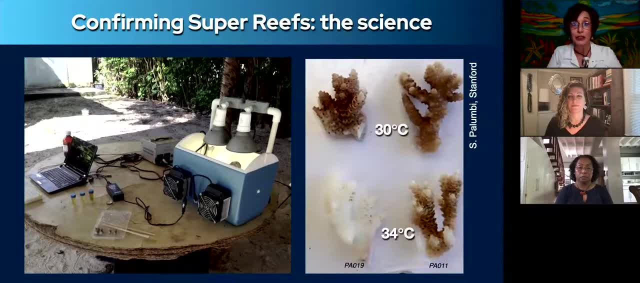 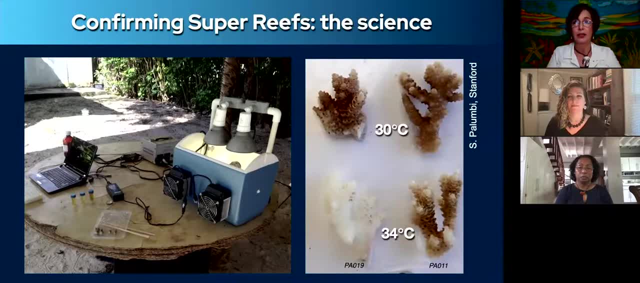 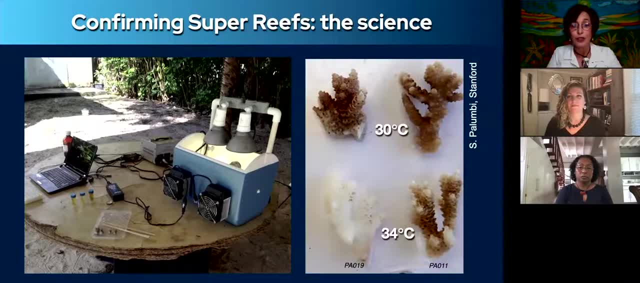 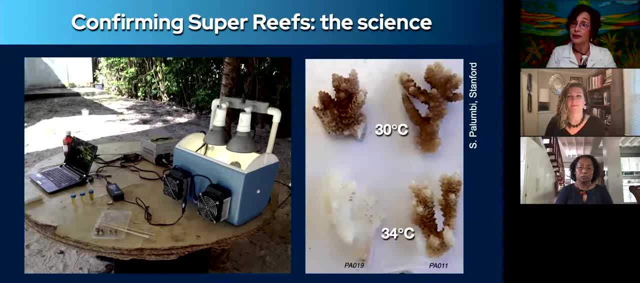 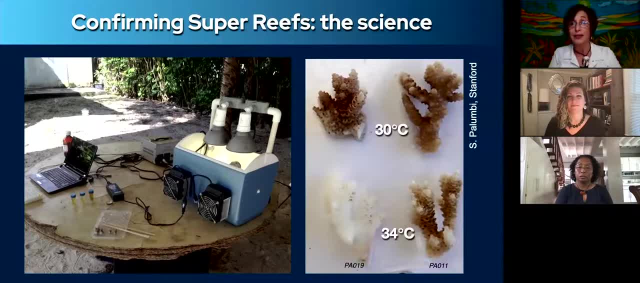 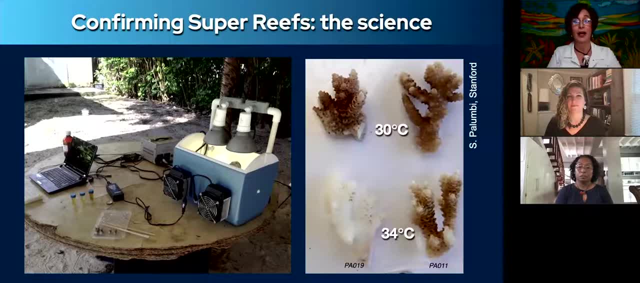 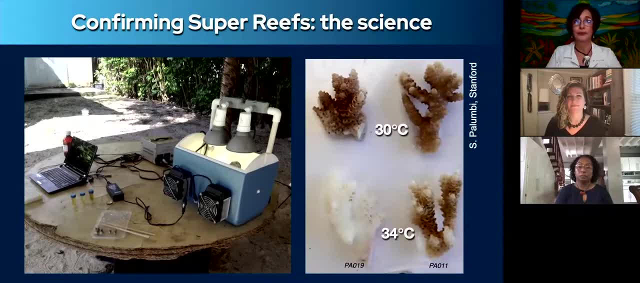 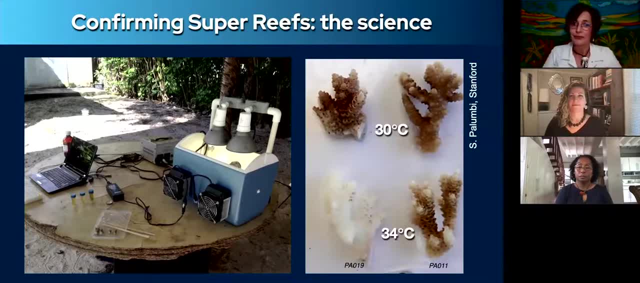 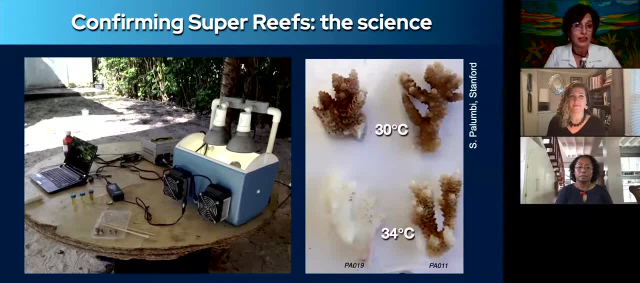 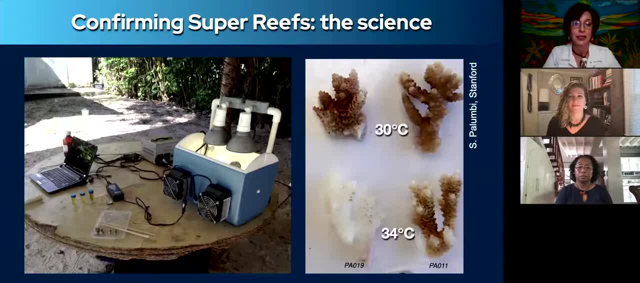 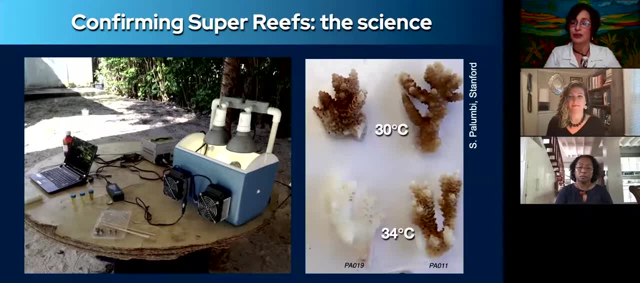 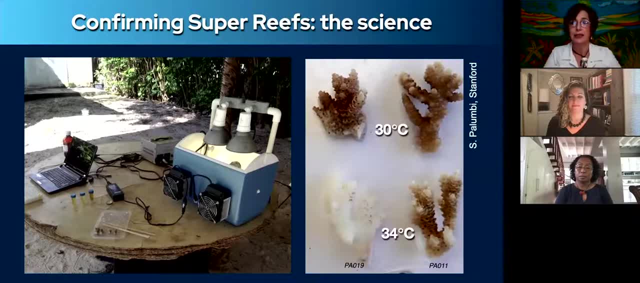 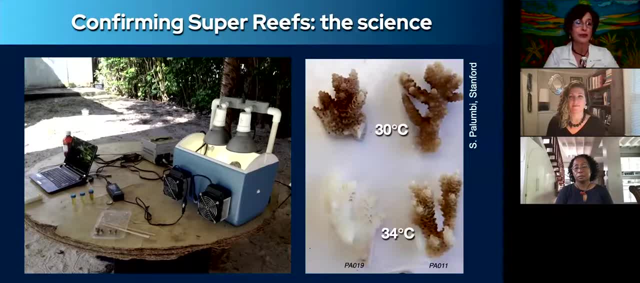 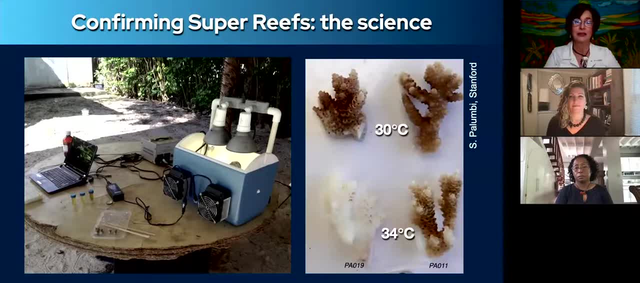 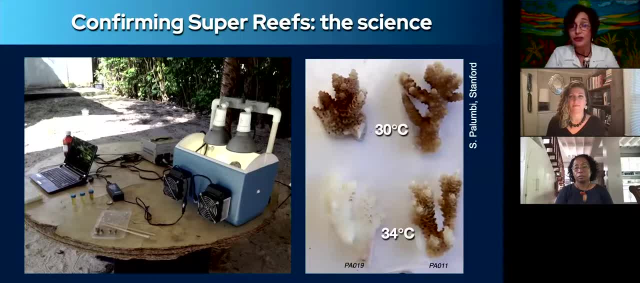 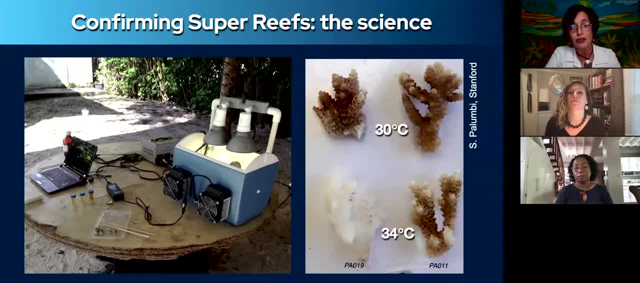 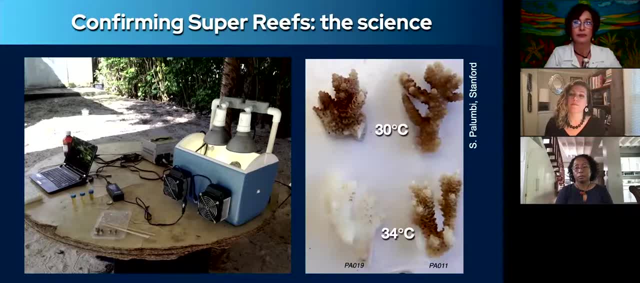 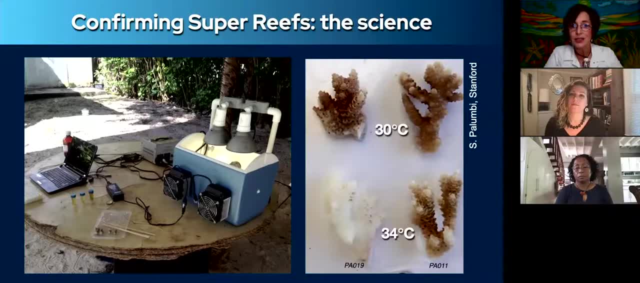 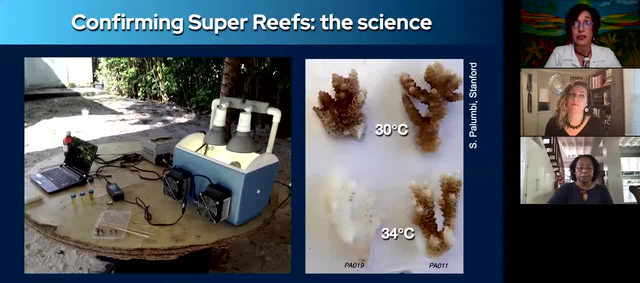 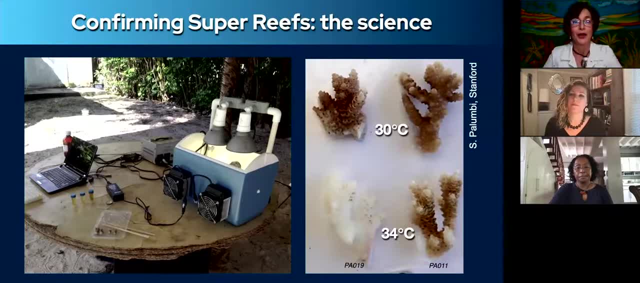 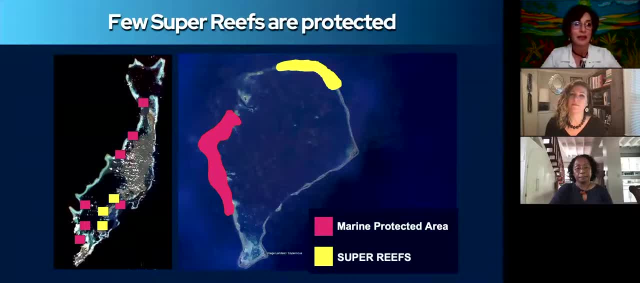 But just because we know these things ei doesn't make it happen In the real world. In fact, at the time we started this project, few super reefs were protected. What this means is that the coral reefs that can survive climate change, that can survive. 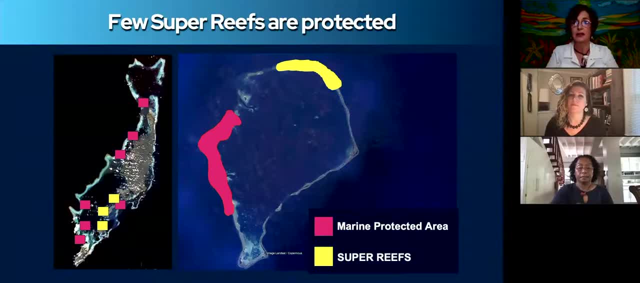 the changes that we're going to see over the next few decades to the local stresses that you'll hear about from Stacey and Anne later in this presentation. These are the stresses like dynamiting, overfishing, erosion, runoff from land. 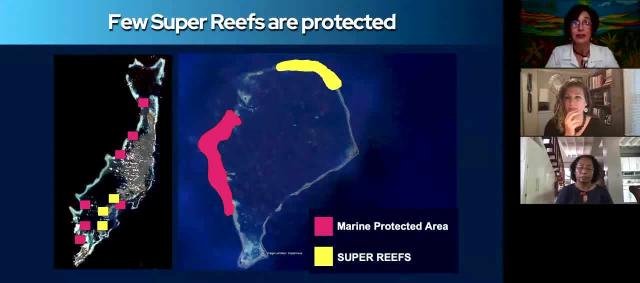 And it's not because coral reef countries aren't protecting their reefs. they are, In fact. Palau- you can see at the left- is a world leader in marine protected areas. It was just that when we started discovering Palau's super reefs. 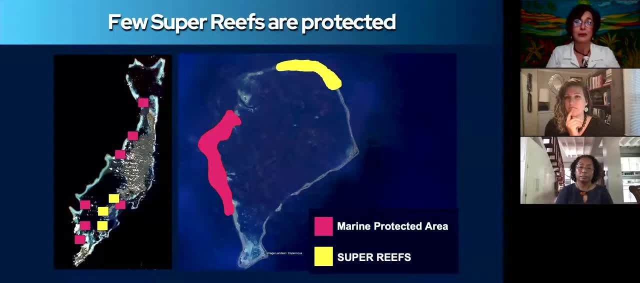 those reefs shown in the yellow were not protected at the time, And at right is a satellite image of an atoll called Funafuti. home to 10,000 people, Funafuti has a huge marine protected area on its west side. It's an incredible accomplishment. 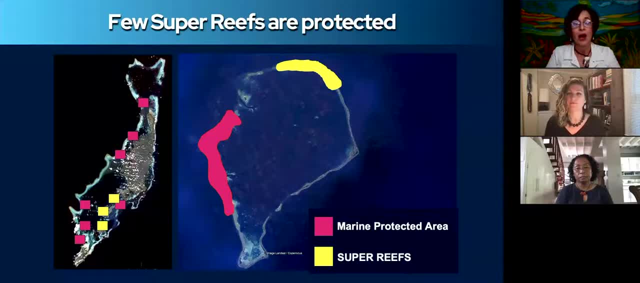 But the corals that dodged the heat wave in 2015 are actually the ones that are protecting it. They're actually located in the north of the atoll, in that yellow area, And they are currently unprotected from the local stresses like jet dredging. 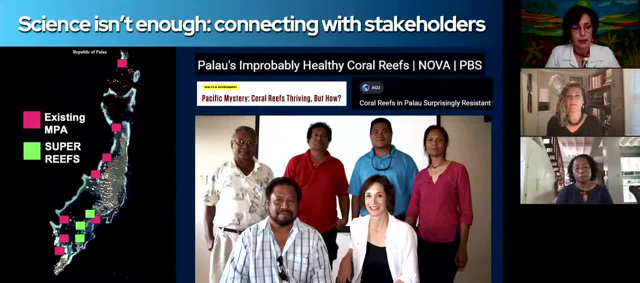 So this is where I realized that the science that I was doing could really make a huge difference to the future of coral reefs on this planet. But publishing in the best scientific journals just wasn't enough. Conservation decisions are being made every day based on the best available science. 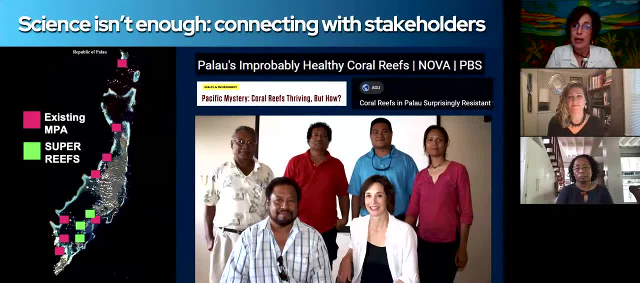 But the scientific process is actually quite slow. Getting papers to press can often take a year or more. So I started to seek opportunities to connect And, to be honest, I was stepping way out of my comfort zone And I made a lot of mistakes along the way. 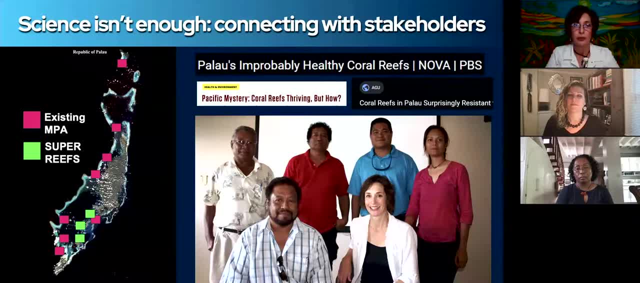 But I also learned a lot And I met wonderful people, very receptive people. I connected with people in super reef countries, with scientists, with government ministers, with conservation organizations. I used every opportunity I could get to get attention on super reefs. 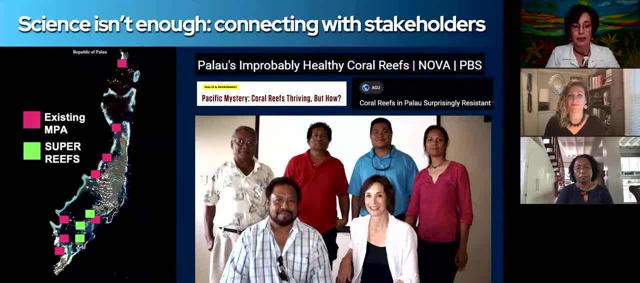 Actually, one day I was sitting at my computer and I got an email from the producers at NOVA And they asked me to review the script for a movie that they were producing on coral reefs And they were talking about how climate change was devastating coral reefs around the world and how 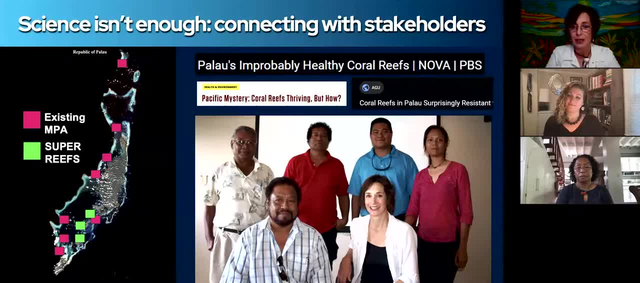 this was an enormous problem, which of course it is, But they had completely left out the super reefs And I said to them: you know, you really can't make this movie without talking about Palau. Palau has coral reefs that are going to survive climate change, that are surviving climate change. 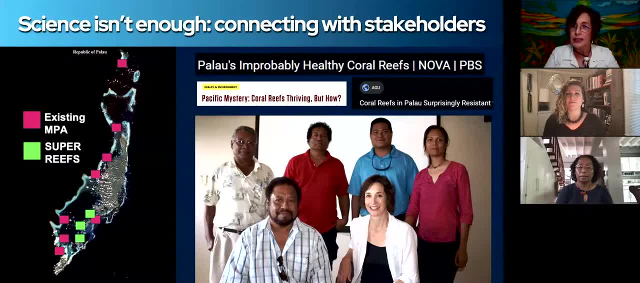 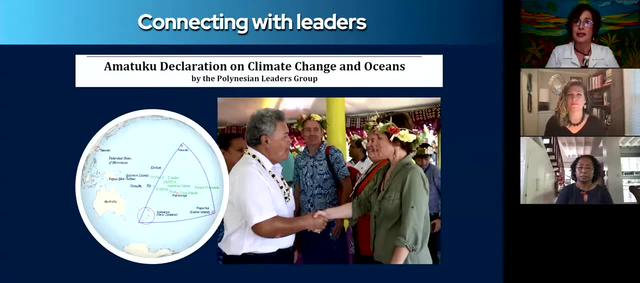 And it was through this, these efforts connecting with the people and the scientists of Palau like I did in this photograph, photograph that, in fact, Palau's super reefs now have elevated protection status. In fact, the last time we visited Palau, it was very difficult to get into our super reef sites. 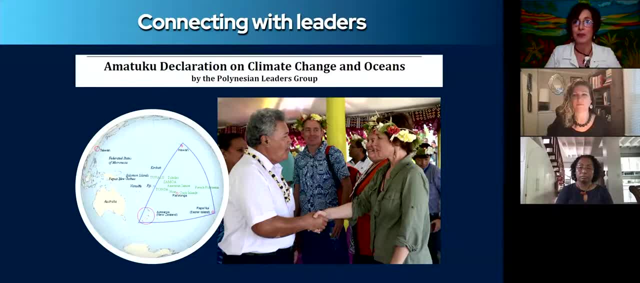 because now they have such better protection. And those efforts and the incredible people that I made along the way connected me with others And in 2018, I was invited to present super reefs to the Polynesian Leaders Group in Tuvalu. I was actually pretty terrified because I mean 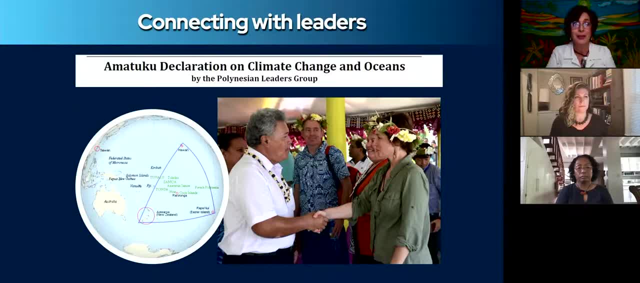 this was like high levels of government. These were presidents and prime ministers of nine Polynesian nations. But here too, super reefs was well received. And at the end of the summit, in the Amatuku Declaration on Climate Change and Oceans, nine Polynesian nations committed to find 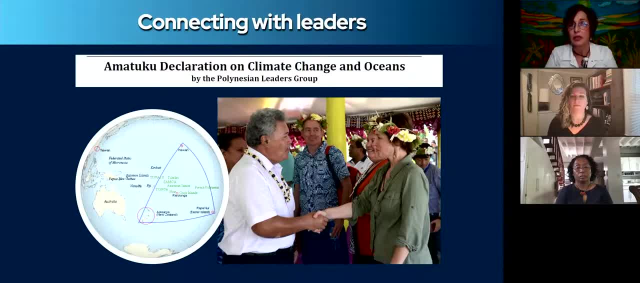 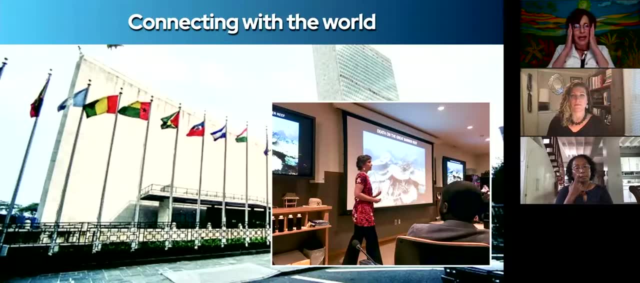 manage and conserve their super reefs across Polynesia. For many island nations, for many coral reef nations, protections can mean tremendous sacrifice And we must see these efforts and acknowledge that. And we must see these efforts and acknowledge that And we must see these efforts. 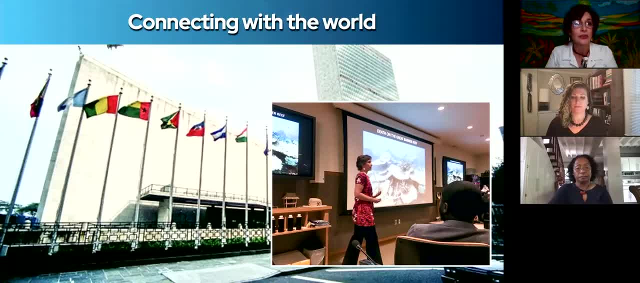 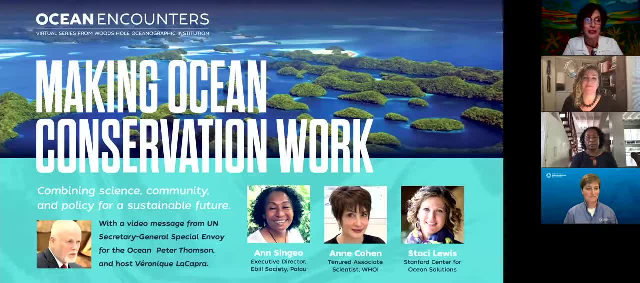 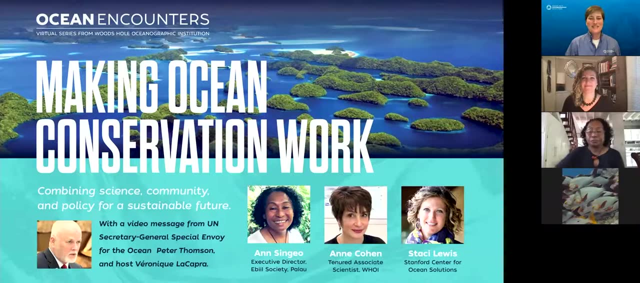 It's been wonderful to share the story with you. I look forward to your questions. Thank you, Lance and Anna. I love that image of the corals sending their eggs out on the currents when the moon is full. That's terrific. Now let's hear from our next presenter, Stacey Lewis. 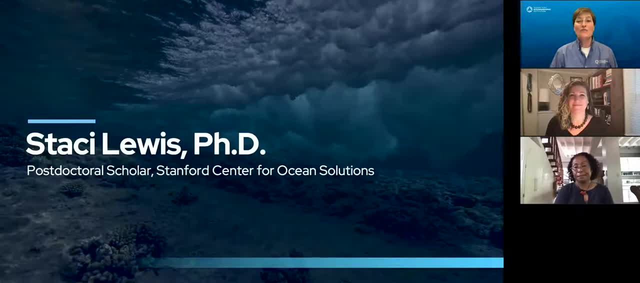 Stacey is an ocean conservation scientist with over two decades of multidisciplinary experience studying coral reef ecology, ocean governance and the human nature of marine life. Stacey is an ocean conservation scientist with over two decades of multidisciplinary experience studying coral reef ecology, ocean governance and the human nature of marine life. 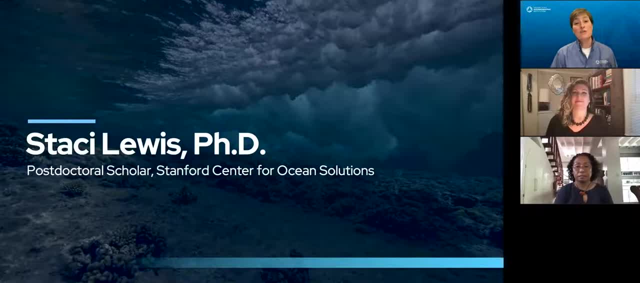 human dimensions of ocean sustainability. She has experience as a policymaker in Washington DC and as a researcher in Palau, an archipelago of more than 500 islands in the Western Pacific Ocean, where she has studied the relationships between local residents, coastal ecosystems, fisheries and policy. 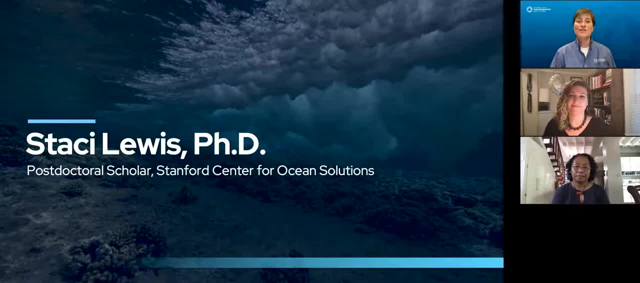 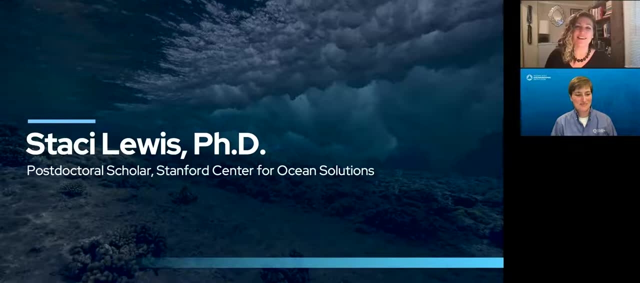 Stacey is currently with Stanford Center for Ocean Solutions, continuing her work in Palau. Welcome, Stacey. Thanks Veronique And hi everyone. Thanks for joining us tonight. I am absolutely honored to be here on this virtual stage with Anne Cohen and Anne Senior. 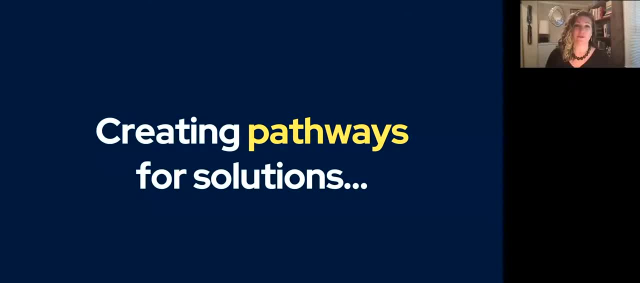 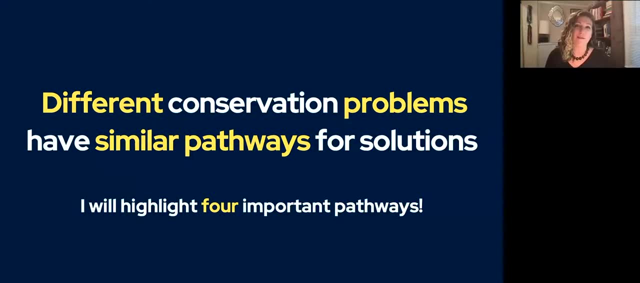 Tonight I'm going to talk about creating pathways for solutions, And the message I want to get across to you tonight is that different conservation problems have similar pathways for solutions, And I'm going to highlight four important pathways, And my story takes place in the Republic of Palau. 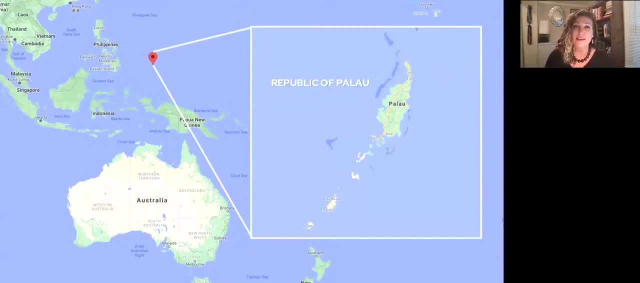 As Veronique said, it's an archipelago in the Western Pacific made up of hundreds of islands, 12 of which are inhabited by Palau's 18,000 residents, over the landmass the size of San Jose, California. Now, while Palau, as you can see in these next images, is an ocean- a big ocean, small island. 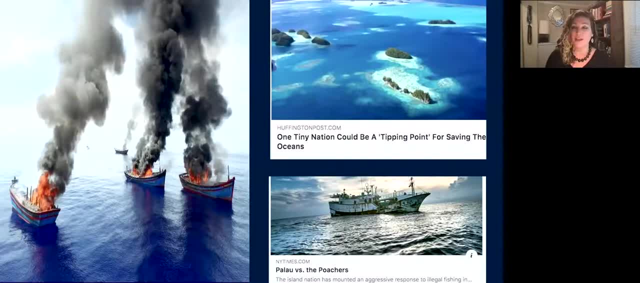 nation. It has a global reputation for its successful strategies in tackling some of the biggest ocean conservation problems, whether it's their aggressive response to illegal fishing or their bold action in 2020 to close 80% of its waters to foreign fishing. But Palau has been successful in other ocean conservation problems, like this one. 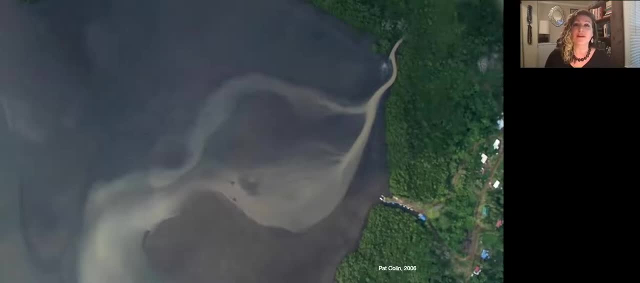 Sediment, Sediment, runoff Sediment, coming out into the coastal zones, smothering corals and degrading these vital ecosystems for the Palauan people. Just like other conservation problems, in order to find solutions, we have to understand. 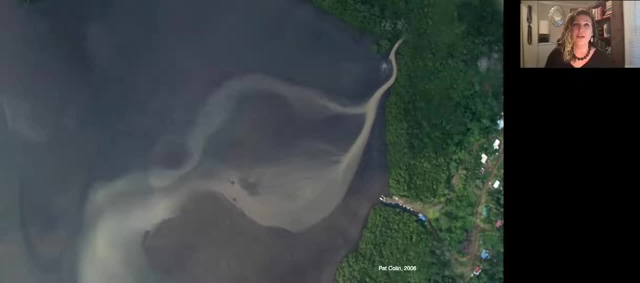 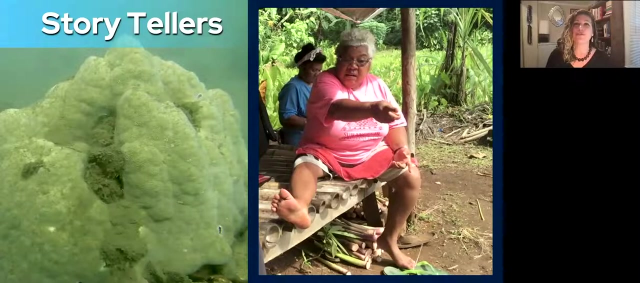 the drivers of those problems And for sediment runoff. those drivers can be told by two storytellers. The first storyteller Is coral reefs that can trace the environmental change in the history. Next slide, please. The second storyteller is the farmers and the fishers who've witnessed those environmental 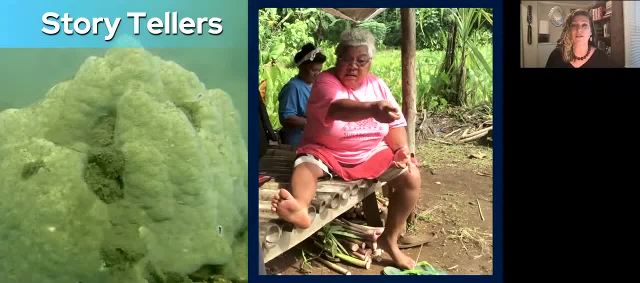 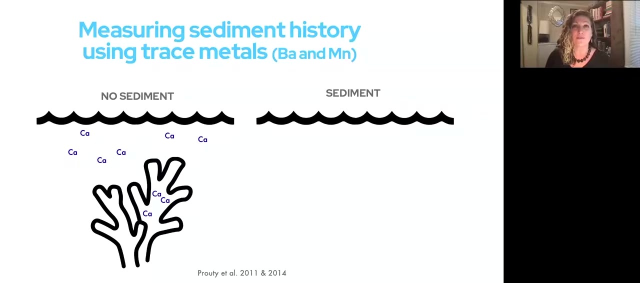 changes. But you may ask yourself, how can corals tell us the story of environmental change? And that has everything to do with how corals grow, And in this next slide You'll see that As corals grow, they draw down calcium from the water column to build their calcium carbonate. 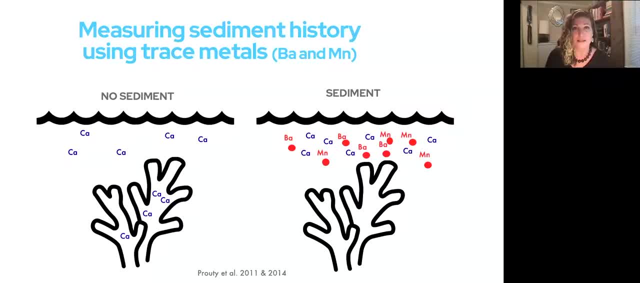 skeleton. But when sediment, particularly land-based sediment, is in the water at the time of growth, that sediment brings trace metals into the water that's similar in structure to calcium, And so corals will draw down those trace metals and have an environmental timestamp in their 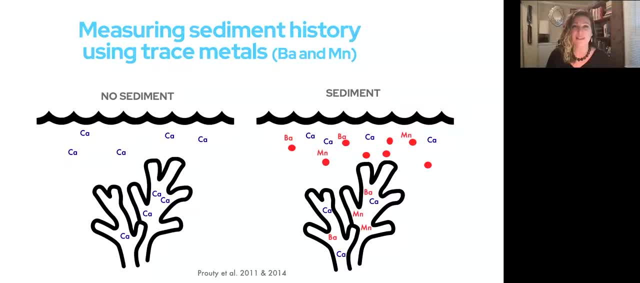 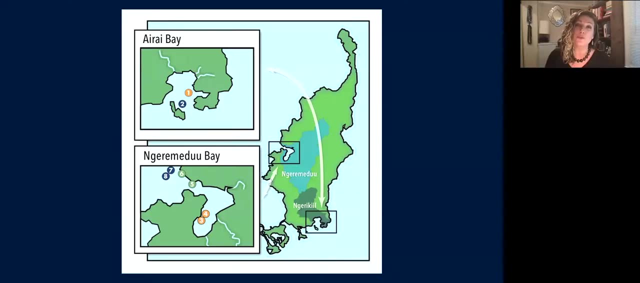 skeleton And for those of us Who are interested in measuring sediment history using these trace metals, we can design experiments and sampling strategies in different watersheds, And on the next slide you'll see my approach to sampling corals in two different watersheds. 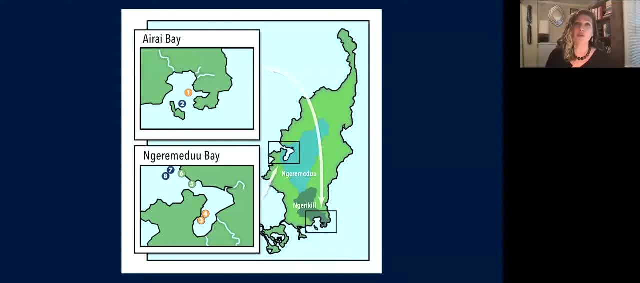 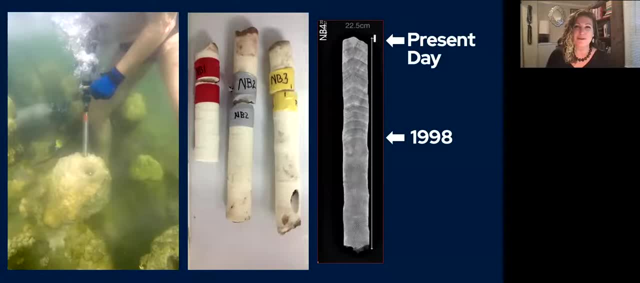 the near Badoo watershed and near Akil, sampling corals near river mouths to the open ocean. And in the next slide you'll see me sampling some of those corals, and then we can use isotopes To establish a chronology or date them. 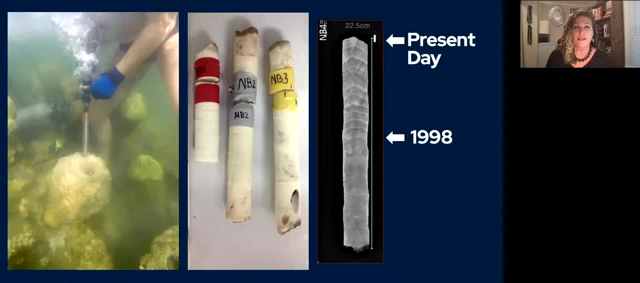 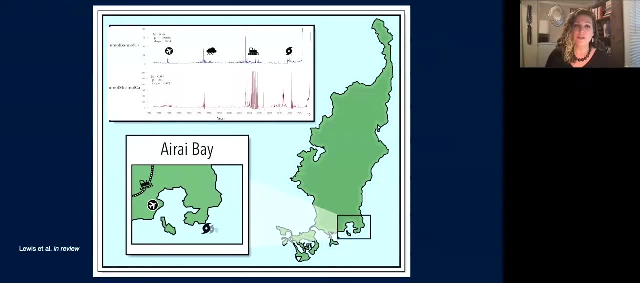 And then we can measure these trace metals in the coral skeletons and compare that with the dating. In the next slide you'll see some of my results From my right bay, the barium to calcium ratios in the tops graph. manganese to calcium ratios. 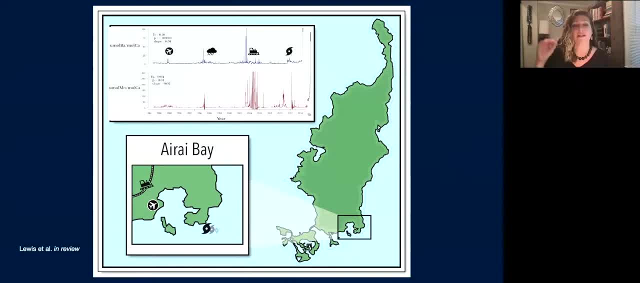 in the bottom. the higher the peak, the more sediment at the time of growth. Now, using historic records, I connected Some of these Peaks to land use change, like airport expansions and road construction, as well as some weather events. But it's important to remember that science is just one cog in the solution wheel. 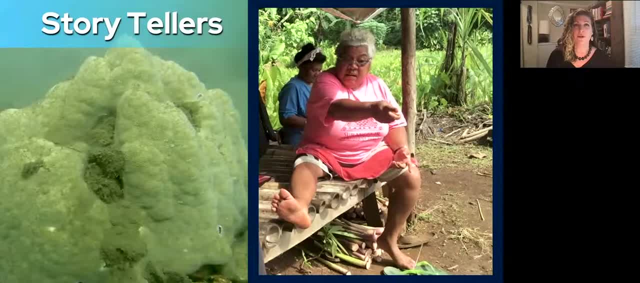 And in order to validate our work, but also to make sure our science gets taken up into policy considerations, We need to talk to our second storyteller, And that's people like oolong. But how do we find these storytellers? And this leads me to the first pathway. 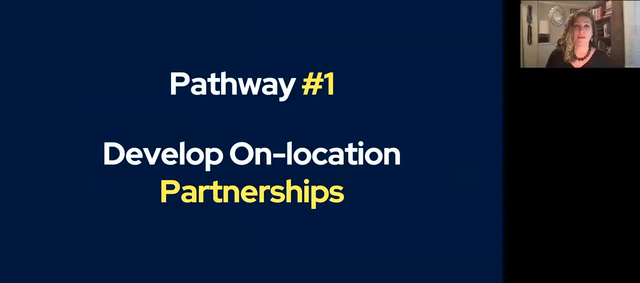 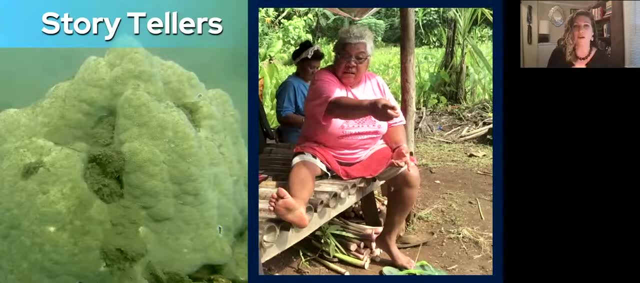 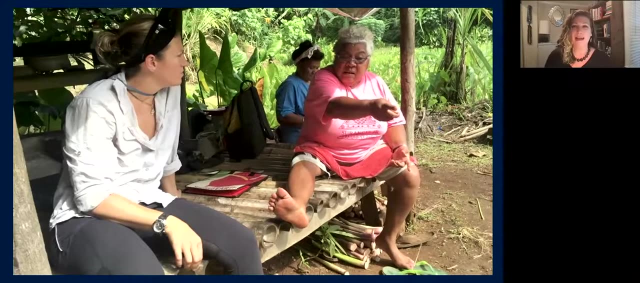 Develop on location partnerships, That's, reaching out to different organizations, community groups, So that we can identify those storytellers. And that's what I was able to do And I spent time with oolong On on those mats in the taro patches. 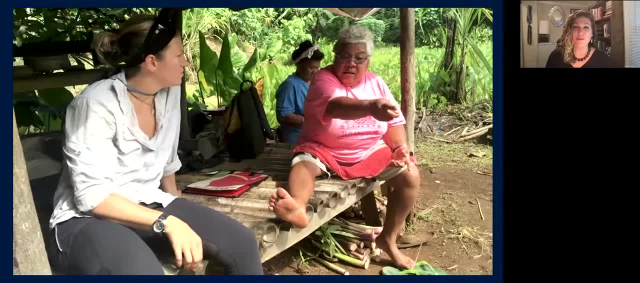 Learning from them How to To Farm those taro patches. Learned about the changes that they've seen. Spent time with reef fishers. Spent time in those rivers to really understand the system, but to also understand their stories of environmental change. 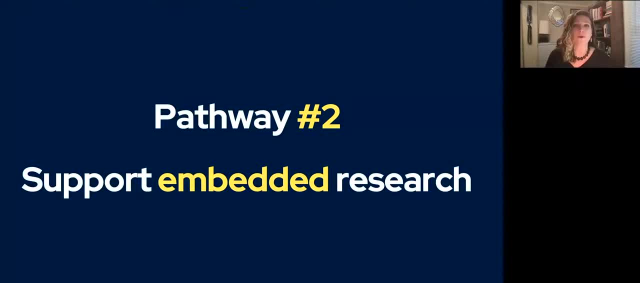 This leads me to my second pathway: Support embedded research. Anthropologists and scientists from humanities embrace embedded research as a way to contextualize their subjects, And I implore Natural scientists to consider embedded research in their approach, whether that's supporting grad students to have extended time in the field. 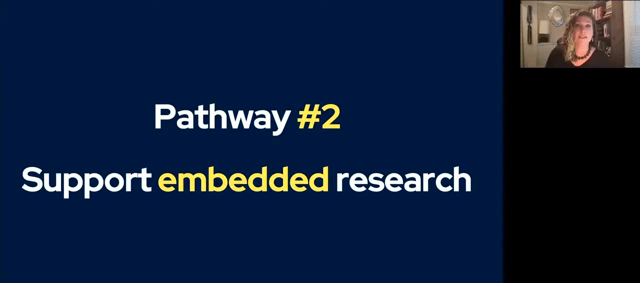 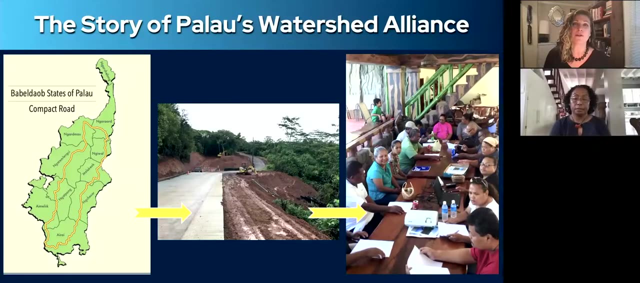 Or establishing long-term collaborations with the places of interest in those groups. But it's through that embedded research that we can really get that thick understanding of what's going on in the field. Through my embedded research it started to become clear the way that Palau was able to. 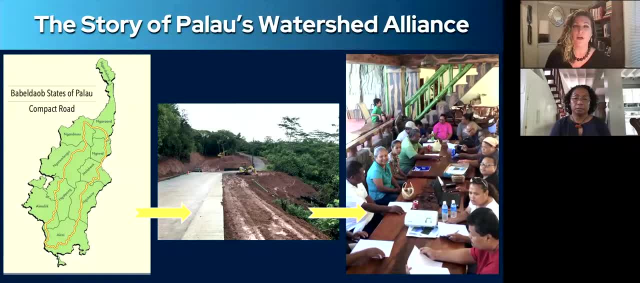 tackle The conservation problem of sediment runoff was through the story of Palau's watershed alliance. It all started with the construction of the compact road, or the ring road, around Babaldab, which took about nine years to construct, And during this time, large areas of land were cleared, leading to large amounts of 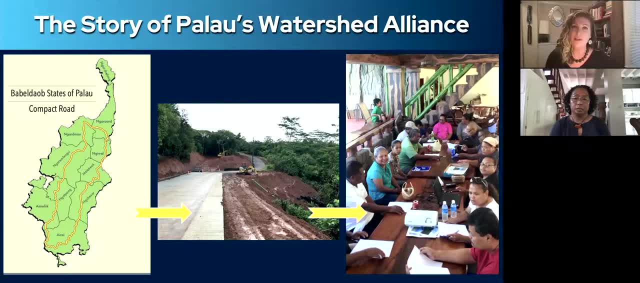 sediments, sediment going into Palau's rivers, clogging up the riverways and smothering their corals. These visible signs of change Mobilized people to come together and ask questions about how do we, how do we, address this problem? 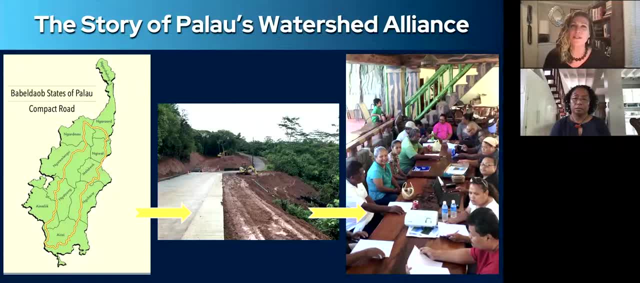 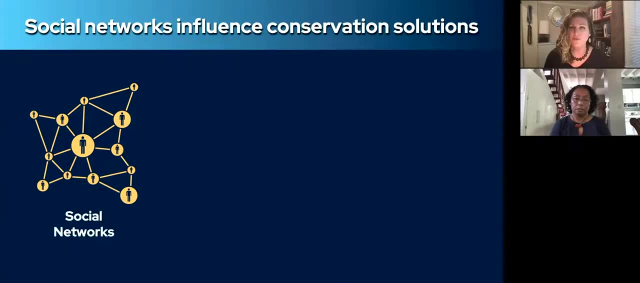 What are the solutions? This mobilization of different actors really motivated me to ask questions about how social networks influence conservation solutions, And when I talk about social networks, I mean people and how they're connected to each other. This is an emerging part of science. 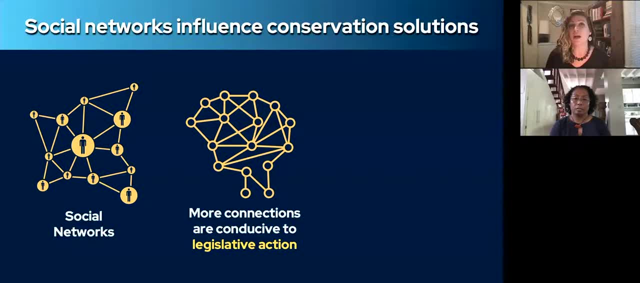 And theory tells us that more connections in a network are conducive to things like legislative action. that requires compromise and consensus. You need to have people who know each other and have higher degrees of trust for that type of decision. Less connected networks are conducive to things like learning. 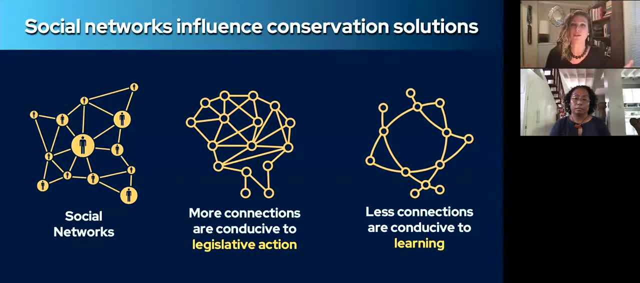 You have diverse stakeholders in a network. They might not know each other, but they might have different ways of knowing and coming together. They can learn from each other, And what I wanted to do is apply these theories and see how it how the Watershed Alliance. 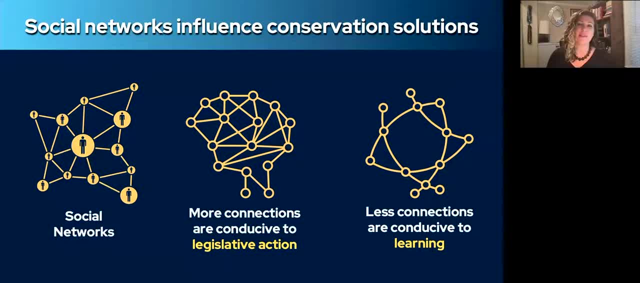 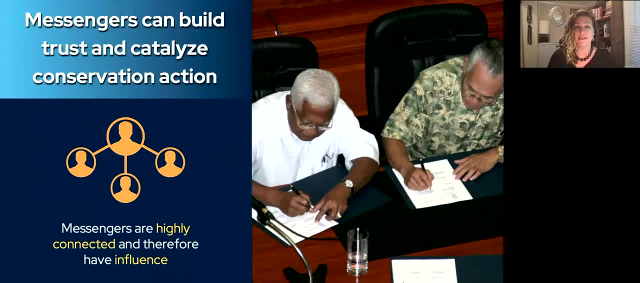 actually aligned with these theories. And that leads me to my third pathway: Find the messenger. And that's exactly what the Watershed Alliance did. They found the BWA, the Bilal Watershed Alliance. founding members realized they needed to find messengers. 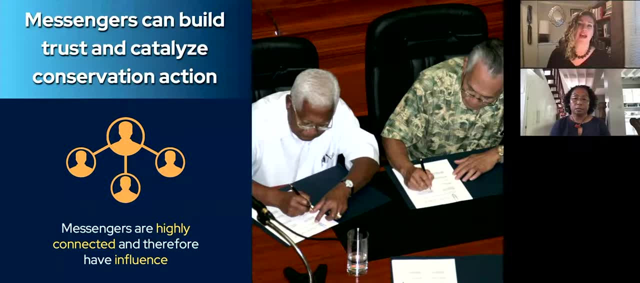 That could build trust And catalyze conservation action. And for Palau, those key messengers were the customary leaders still revered by communities for their authority on environmental stewardship. These messengers are highly connected and therefore have influence, And what they were able to do was to build communities' trust on what the Watershed. 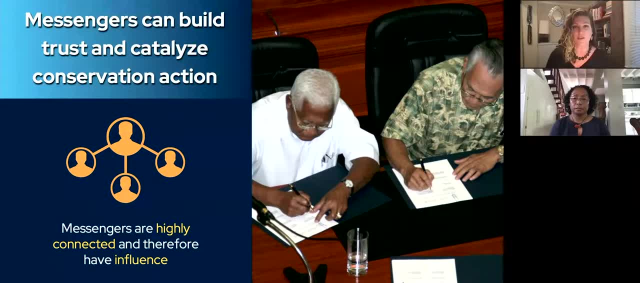 Alliance was trying to do, but also get legislators and state policymakers motivated to create past laws, to create protected areas on land and in the water, to combat the sediment runoff. But passing these laws and creating those protected areas, that's just the first step. 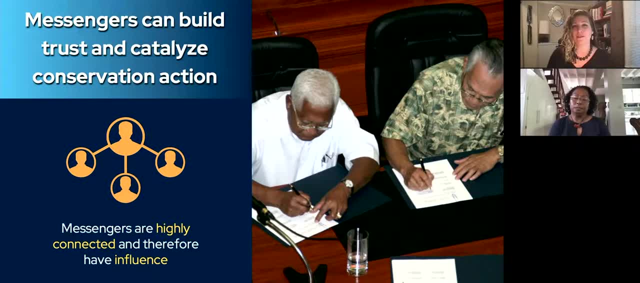 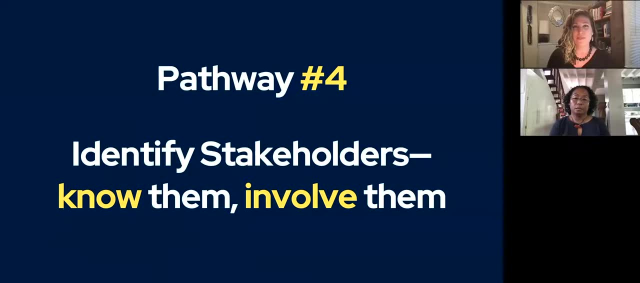 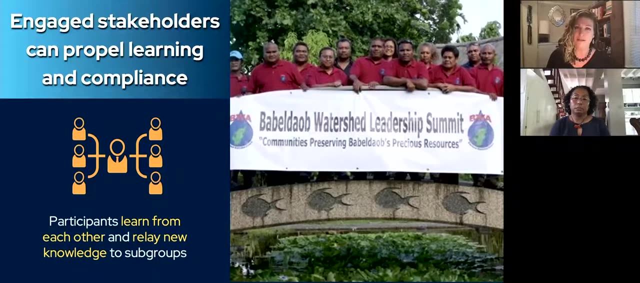 Now the real work begins, And that's my fourth pathway: Identify stakeholders, Know them, Involve them. And that was the next step for the Watershed Alliance. They engaged stakeholders To propel learning and compliance. They brought participants from different quarters of the communities to learn from each other. 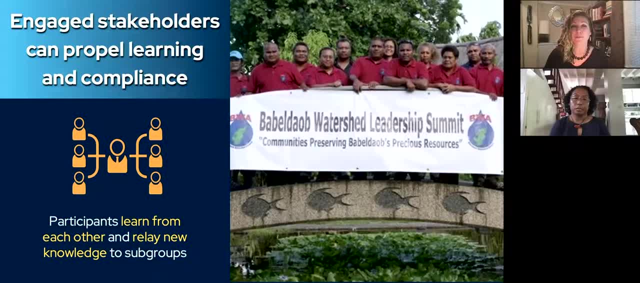 and relay new knowledge to subgroups. Through these efforts, awareness, there was an increase in general awareness, not only of the problem of sediment runoff, but the fact that individuals can change their behavior and that different outcomes could be changed. They could come out of just changing your behavior: complying, participating, cooperating. 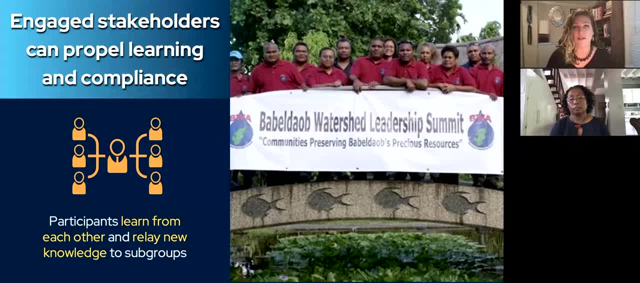 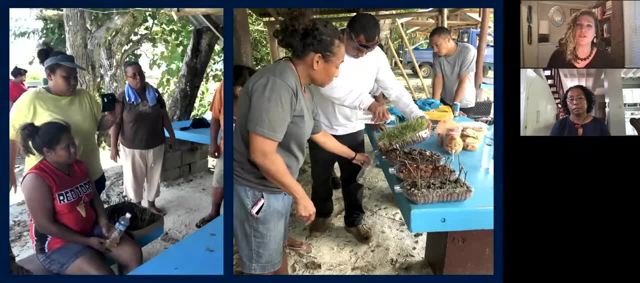 in these protected areas being part of the management planning process. These outreach and education events continue today And in the next slide you'll see pictures of a more recent demonstration- And this is our next speaker Encinio having one of these demonstrations of how water retention 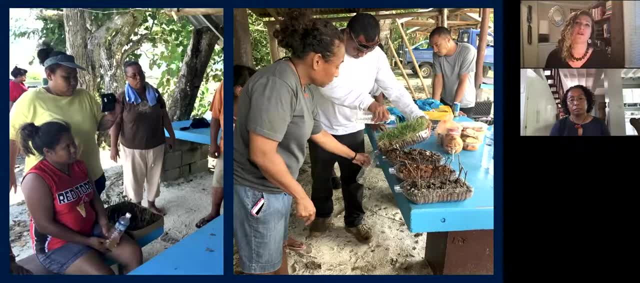 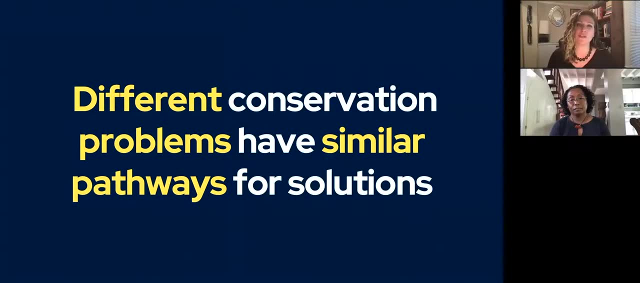 is different When you have grass versus dirt, When you have soil versus different types of soil, And so I'll go back to my message from the beginning. Different conservation problems have similar pathways for solutions. So when we're talking about coral reef conservation and protected areas, we think about those. 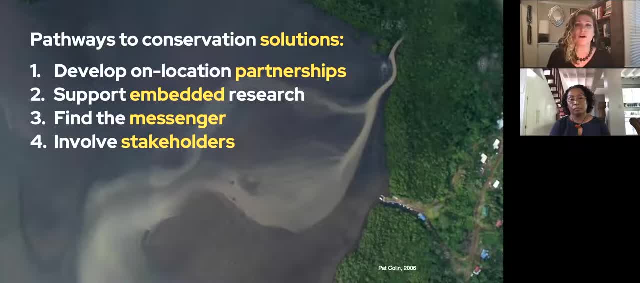 pathways for solutions. It's developing those on-location partnerships. It's supporting embedded research so we can connect what we're finding When we're finding what we're finding When we're finding these super reefs, connecting it with the people who depend on those super 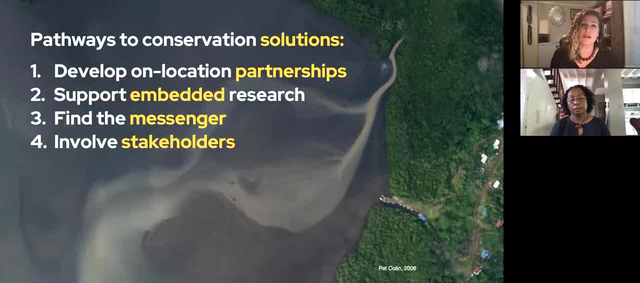 reefs, Finding those messengers to carry it not only to the policymakers but to the stakeholders and the other resource users, And involving those stakeholders who have so much to lose from not acting And they have so much to gain from these solutions. 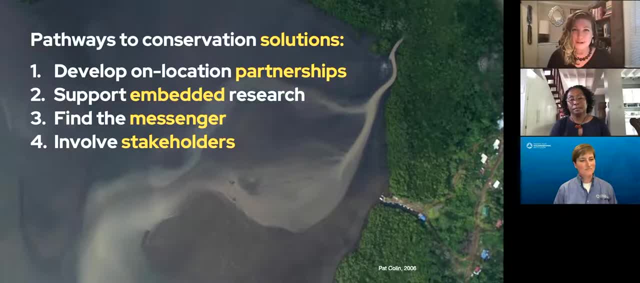 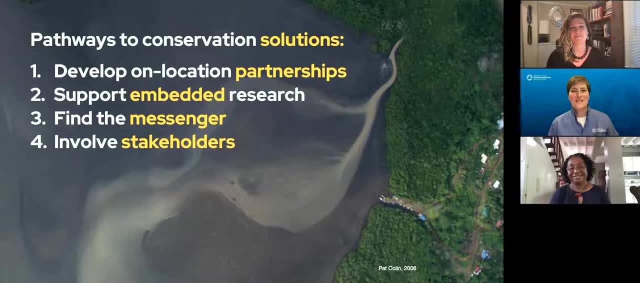 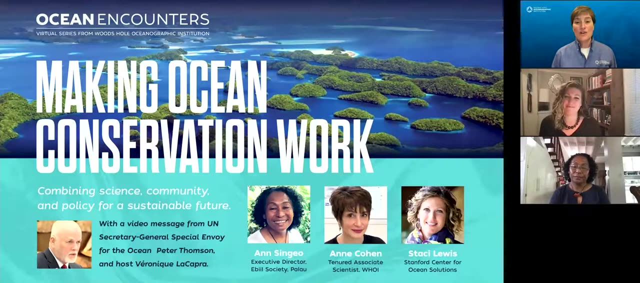 I can't think of a better messenger or researcher to talk more about these types of pathways than our next speaker, Anne Hsing Yu. Thanks so much. Thank you, Stacey. Before we go to Anne, we do have an audience poll that we want to do. 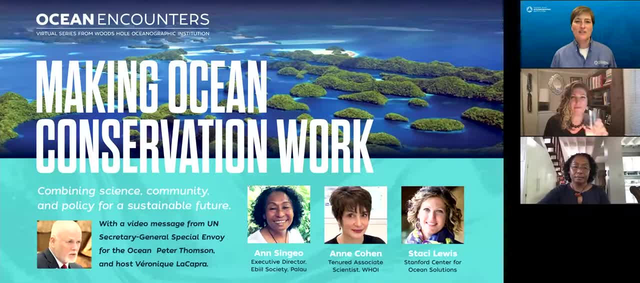 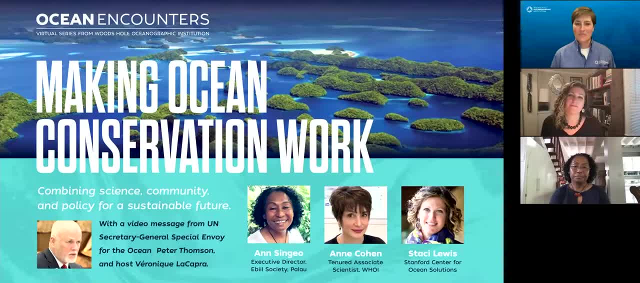 How much of the global ocean is protected. How much of the global ocean is protected And what is the percentage of the ocean protected? Anne Hsing Yu: Lots of people participating. That's great. All right, Our poll is now closed And, as most of you figured out, the answer is 7.5%. 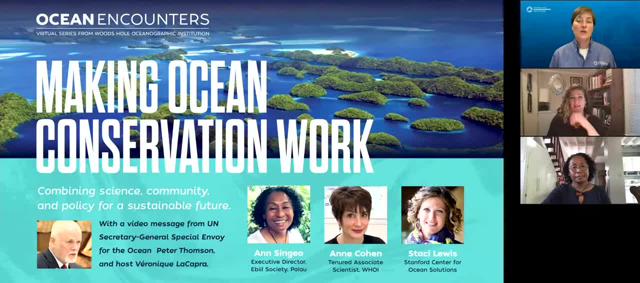 So not very much of the ocean is protected, Anne Hsing Yu. And the percentage of the ocean is protected- not clear ocean with protections that limit extractive activities like fishing and mining- is even lower. It's somewhere around 5%. All right, Now I'd like to introduce our third speaker. 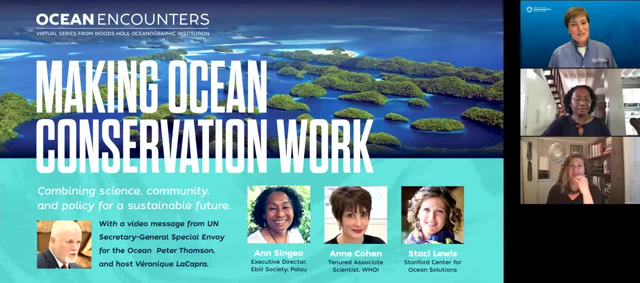 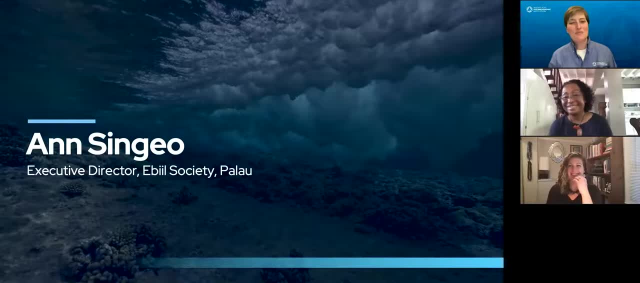 Anne Singale. Anne is actually joining us from Palau right now, where I think it's a little after 10 in the morning tomorrow, So we're spanning both time and space to bring you this event tonight. In Palau, Anne works with communities to develop programs to support. 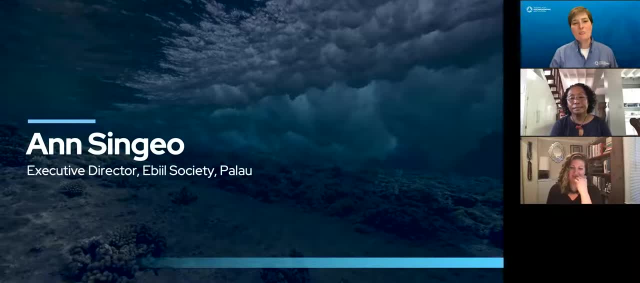 livelihoods and to sustain natural resources. Anne is the executive director of the Abil Society, a nonprofit organization that provides environmental education based both on traditional knowledge and science, and which also advocates for community-based governance for effective conservation and resource management. Anne. 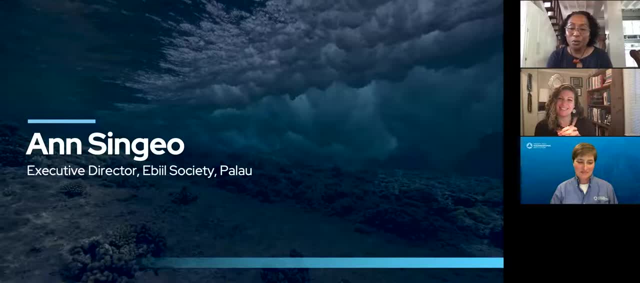 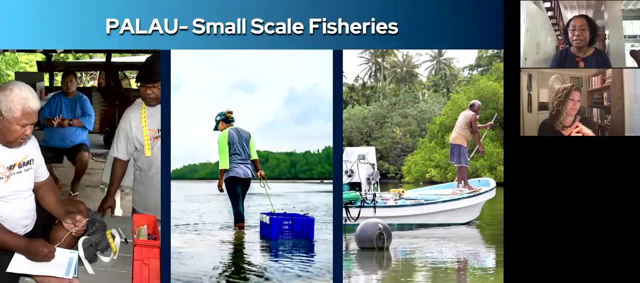 Thank you, Veronica, And good morning everybody from Palau. In Palau, and particularly at Abil Society, we work very closely with resource users on the land- farmers, builders and fishers- And in my presentation I'm going to use a current project that we're doing in Palau to 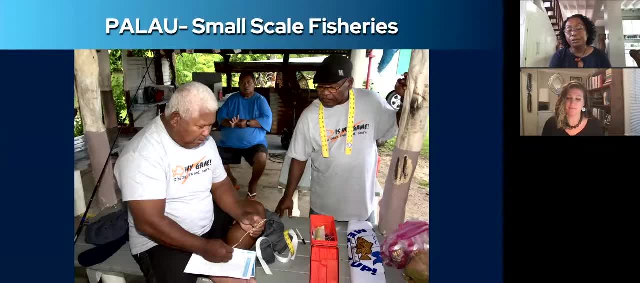 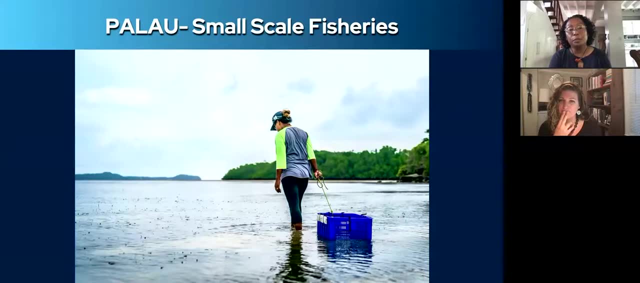 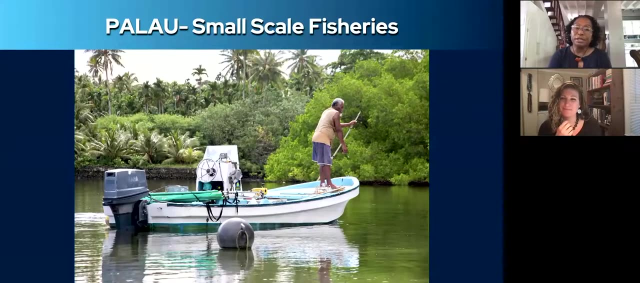 illustrate the importance of knowing who your stakeholders are and engaging them right from the beginning in order to develop successful implementation of conservation projects. So Palau, small-scale fishers, actually traditionally has an, and it involves men and women. Women are the fishers of the shallow coastal areas, from mangroves to fishers And in the 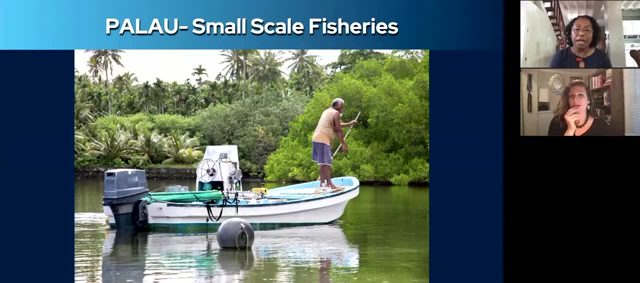 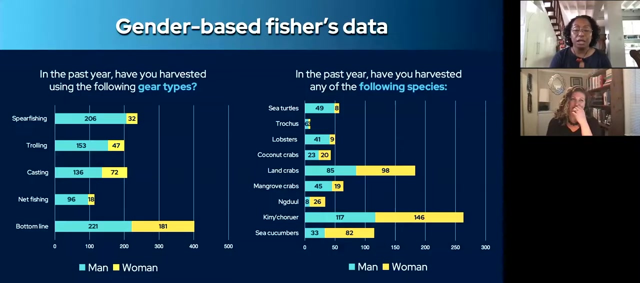 the nearest coral reef slope, and men tend to fish in the deep water but beyond the lagoon and also into the deep sea. But more recently, with all different types of science and development on fisheries programs and management, the tendency is to always assume that the men are the users of the ocean and would have a tendency to engage with men. 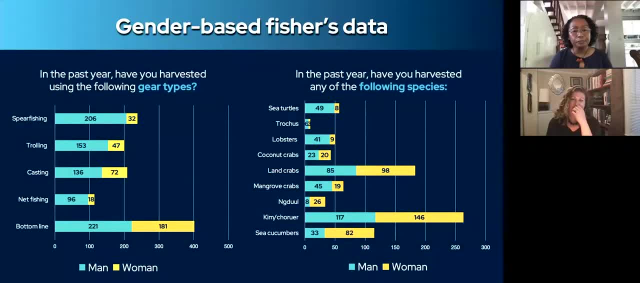 and exclude women in the conversations And, as a result, the the fisheries, where women are the the participants or dominant users. the habitats have been lost to degradation or permanent chains from unsustainable development, including overfishing Of the particular species in those habitat. In this graph, it shows how men and women are. 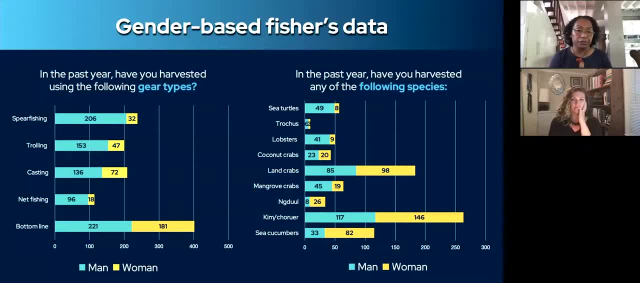 are both engaged in fisheries, and on the left side it shows gear types where men tend to dominate- spearfishing, trolling, casting, net fishing- but men and women are about equally distributed in the use of bottom line fishing, But when it comes to harvesting, gleaning and harvesting- you can see that women are more. 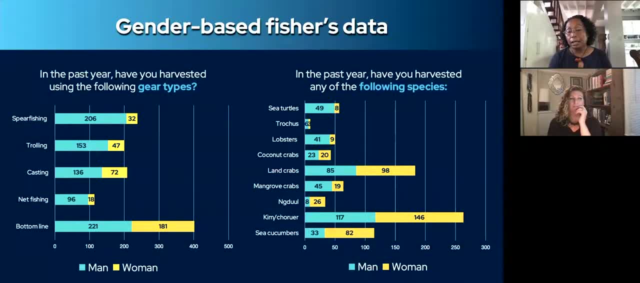 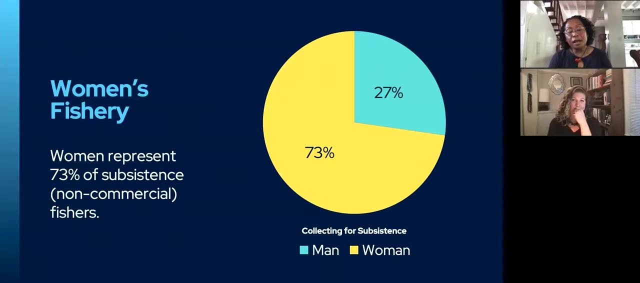 dominant fishers in collecting crab clams of different types and as, and so much more. in terms of sea cucumber species, Women are represent 73 percent of our subsistence market. This is also the basis of marine fisheries, As well as general marine fisheries. we are 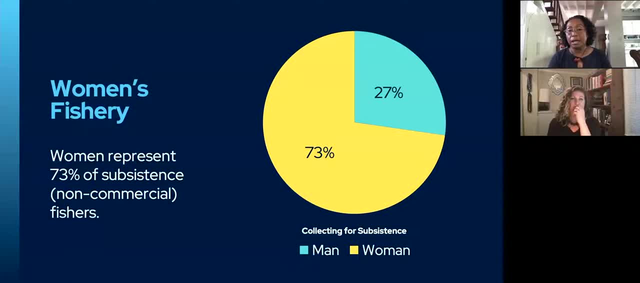 interested in the women, who are one of the main fishing species in our community, And so we are turning to traditional seafood and to use them as the starting point for our fisheries activities, which is a very important statement to make, Because not only are they the vast users of the nearby marine areas, but they are also 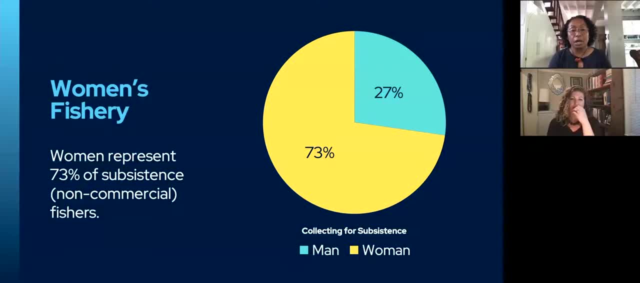 the dominant market traders of seafood in our small village market. And the women fishers are not just down in the river, They are also the men who are the most prevalent fishermen, Instead of what we call the women fishermen. women fishermen are the men who are the most. 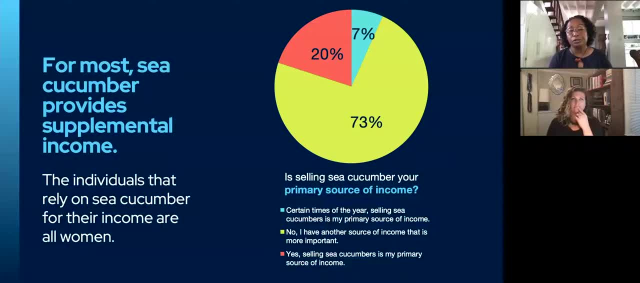 dominating the market, but they are also. they count on the sales of their fisheries to support their livelihood and as their primary source of income, compared to men, who most of them are fishing and selling to supplement a job that they already have. so not including women in conversations of management or even development programs for improving fisheries management? 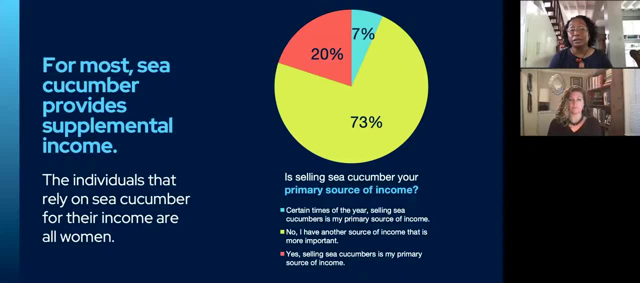 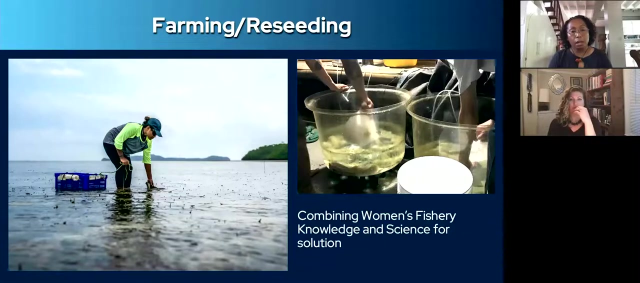 can really result in devastating loss of marine habitats, as well as impacting and displacing families and lives that rely on those resources for their livelihood. and so this from this research, where we had an had an opportunity to talk with various fishers across Palawa and visiting habitats with these women, including visiting interviews with local scientists. 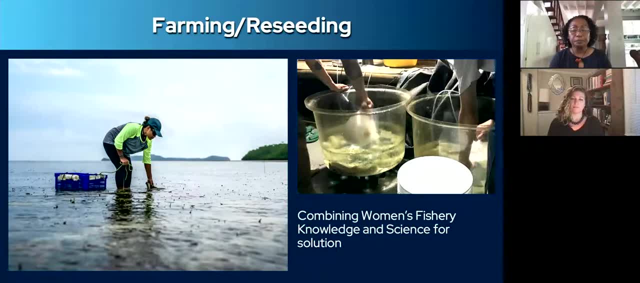 and abroad, scientists abroad, it became clear that the not only are we, should we begin to look at the managing better those resources that women rely on, but it is almost at a point of, at this point of depletion. it's, it's, we're at a point of almost a serial depletion. 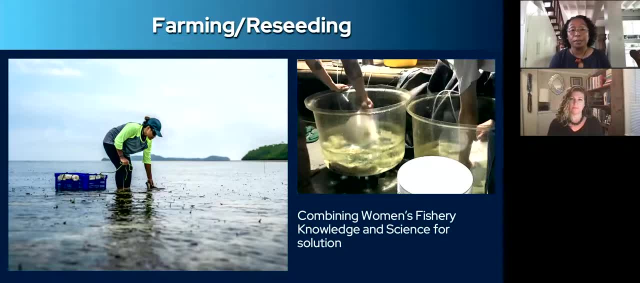 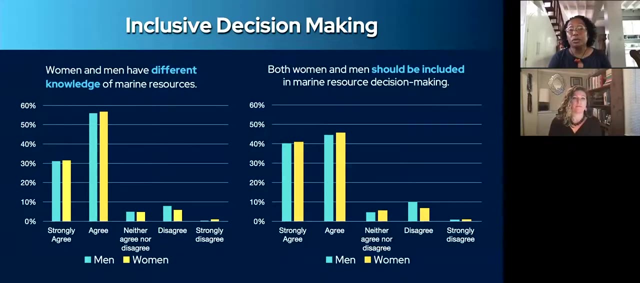 where, if we don't take quick and robust actions to restore our marine habitats, there is a chance that we could lose them forever. and so, with this, the results of this research and the information gotten from the fishermen, we have began to increase conversations about the size of the ocean, the location of the ocean. we have to look at the sea. 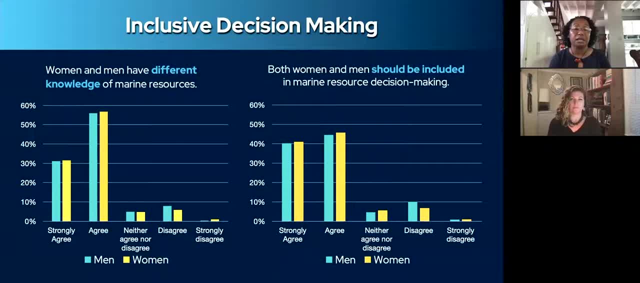 and as a result of this early discussions, I think we have managed to address the issue about the size of the ocean now. so it's a wide spectrum at the moment and it's a very big problem that we are currently facing with your work. I also have to consider this as a really big problem. 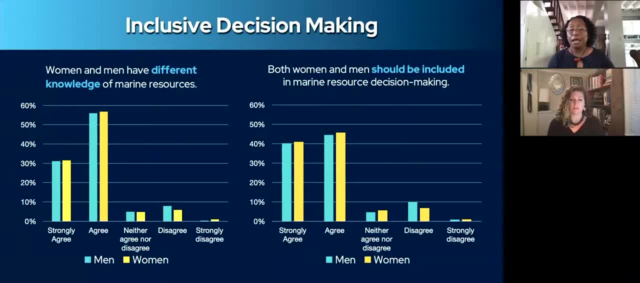 and I am not saying that we could not solve it, but I do think we can solve it, because it is a really big issue to learn how we can surely improve our marine habitat heute. thank you, thank you. it's a very important issue to learn about our ocean as a community or as a whole. 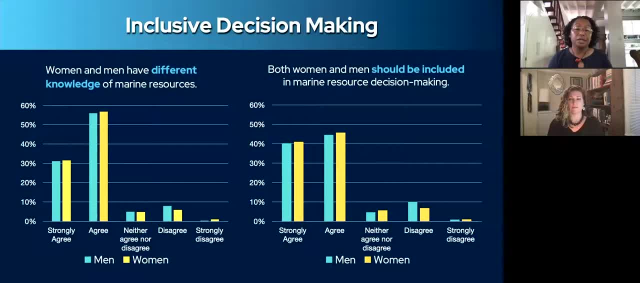 or greatly devastated those fishing grounds, And so, without including the comprehensive men and women resource users in this dialogue, you may design management plans that may not be as effective, And so, with this, our current project now is combining science and fisheries. women fishers' knowledge of lunar cycles. 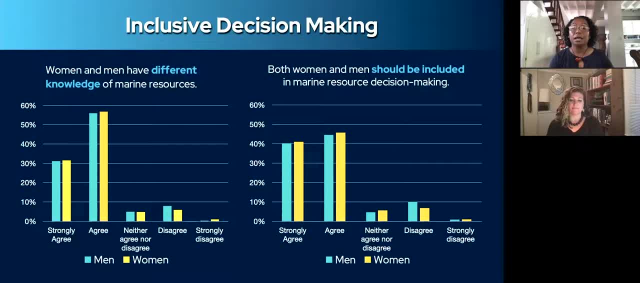 and spawning tendencies of the species that they target, to improve our hatchery spawning activities that will focus on restoring sea cucumbers into this natural habitat, This devastated fishing grounds, so that women can once again be able to rely on the same resources that they have for thousands of years. 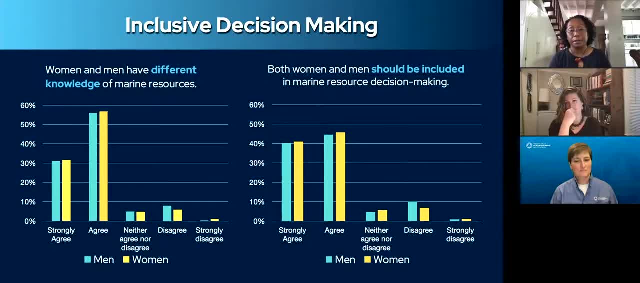 and continue to rely on those resource to support their families, And so taking a science approach and developing a solution that is conservation focused, that eventually will improve the social benefits deriving from improved seagrass and other marine habitats. Thank you, Thank you, Anne. 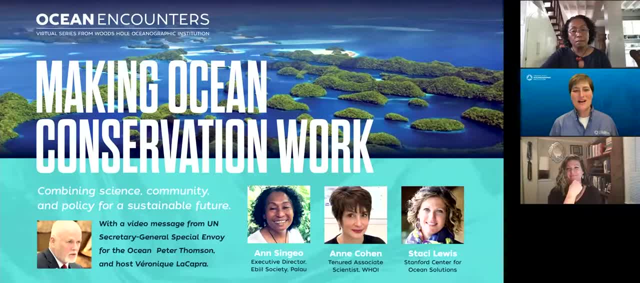 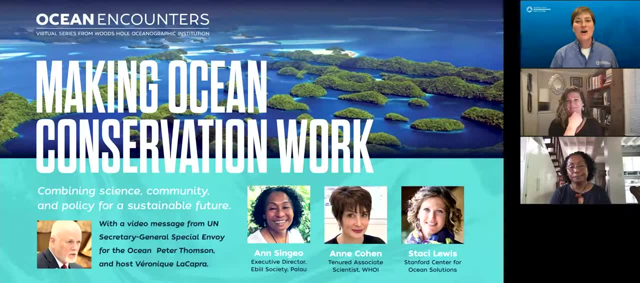 And thank you to Stacey and other Anne as well. Before we open things up for audience questions- and we've been getting a lot of questions behind the scenes here- we have one more perspective. We have one more perspective That we'd like to bring in to the discussion. 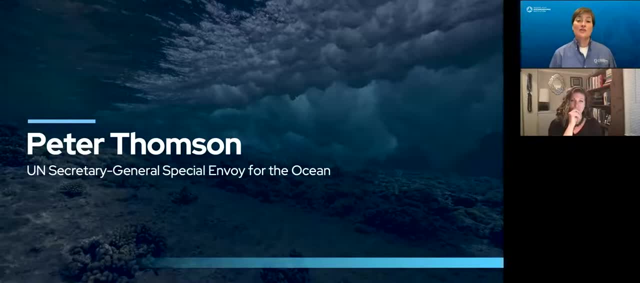 Peter Thompson is the United Nations Secretary General's Special Envoy for the Ocean And, as you'll hear, Peter is from Fiji, a nation of about 300 islands in the South Pacific Ocean and home to numerous coral reefs. Peter was unable to join us in person tonight. 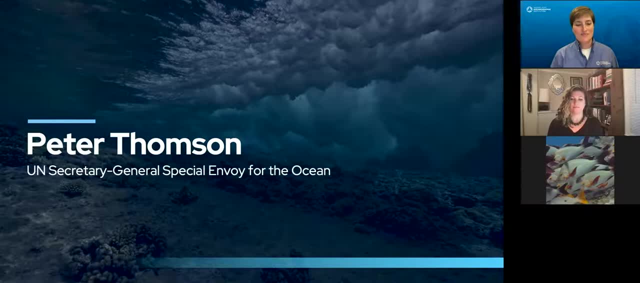 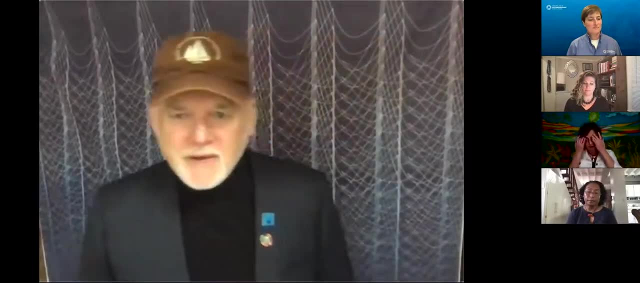 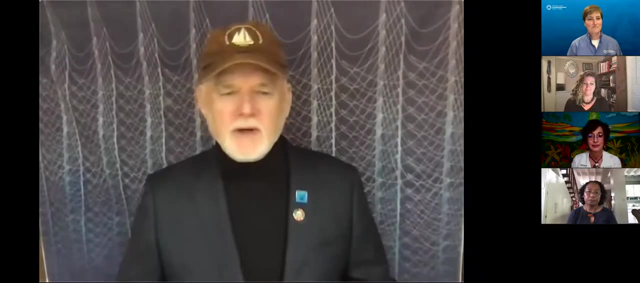 but he wanted to share this video message with you. Ladies and gentlemen, greetings to one another, Good afternoon and welcome to you all, Wherever you are today, And I hope that you and your loved ones are healthy and happy. And many thanks to Woods Hole Oceanographic Institution. 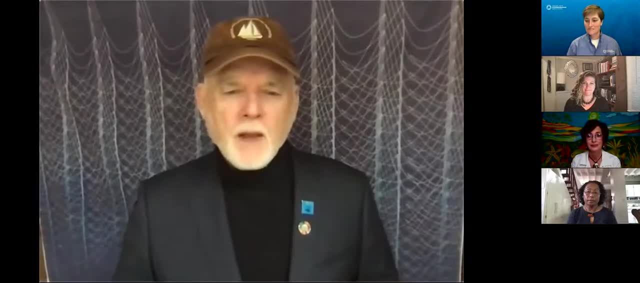 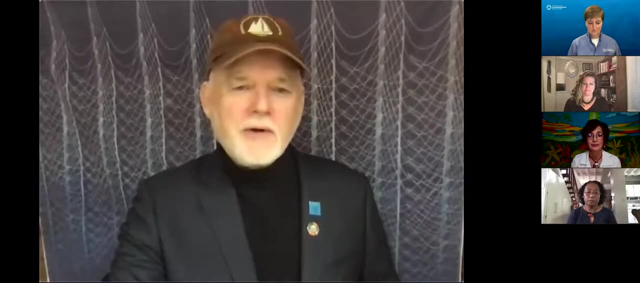 for the opportunity of addressing you all. As you may know, I come from Fiji And, in such, my earliest memories revolve around the ocean, alongside it and on it and in it. When I think of those times today, I remember the hardships of storms at sea. 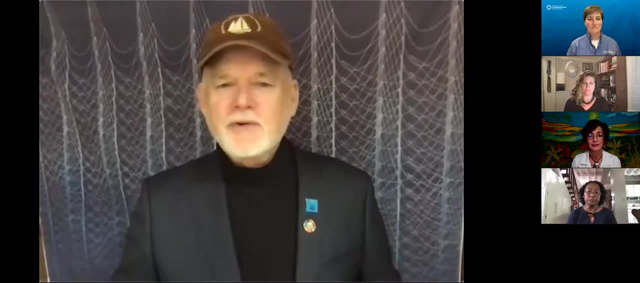 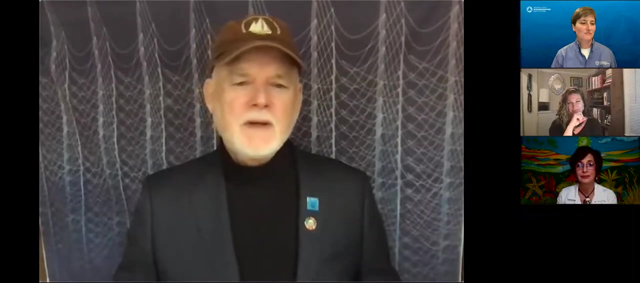 of seasickness and incessant ocean swells, Of being caught in currents and in the ocean undertoes when swimming or being stung by jellyfish and cut by coral. but then i remember the eternal beauty of seascapes, the wonder of arrival at islands by sea, the great joy of diving. 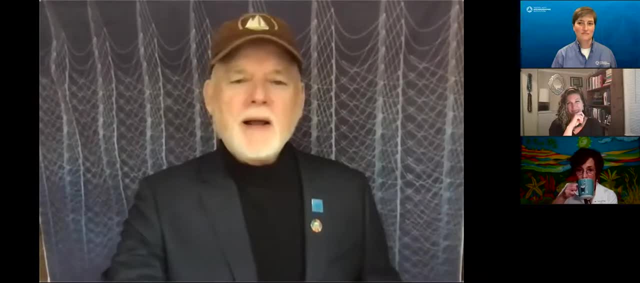 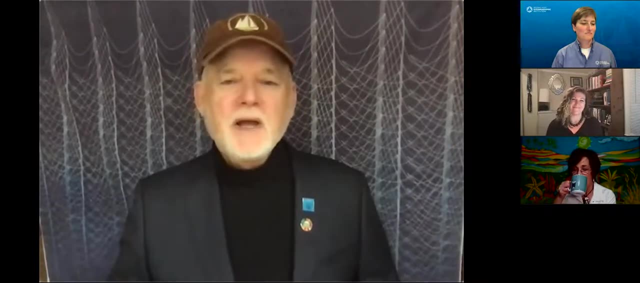 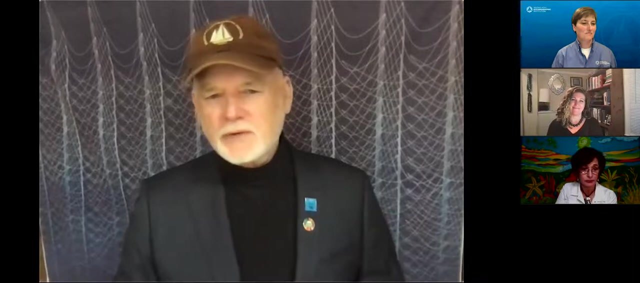 in coral canyons teeming with life, or paddling homemade tin boats through the mangroves and out into the lagoon, feasting on succulent seafood and breathing in the cleanest of air possible, propelled by southeast trade winds across thousands of open miles of the south pacific ocean. 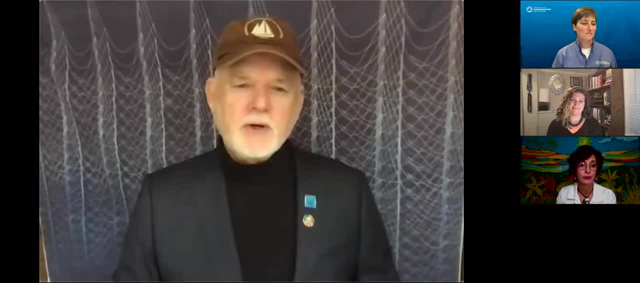 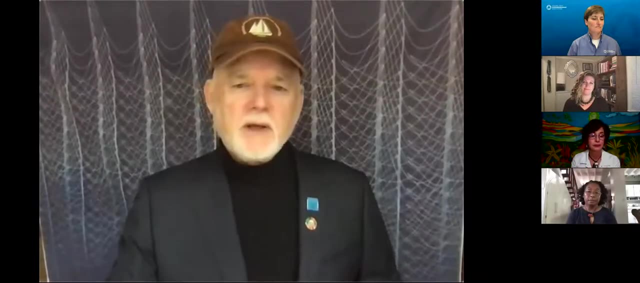 you know, it wasn't until well into my life that i heard the expression coral bleaching and witnessed its decimation when diving. the only desolation i can compare that to is the pictures i've seen of cities turned to lifeless rubble by incendiary bombs as a youth. 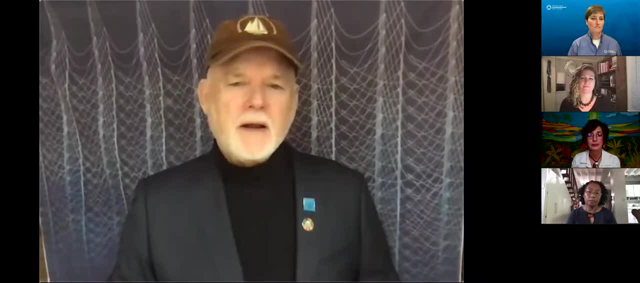 the only flotsam and jetson to be found on our beaches were organic shells, timber, seaweed, and if you were lucky enough to find them on the beach, you could find them on the beach. in the sea, you were lucky enough to find a nautilus shell or the occasional glass fishing float netted in. 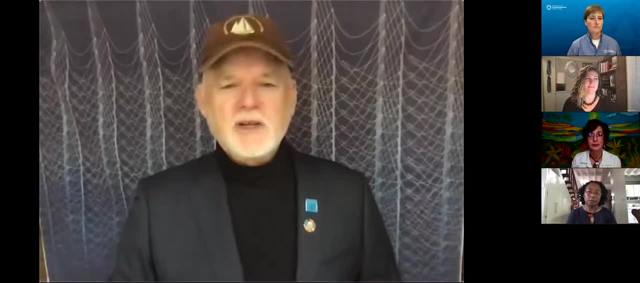 ragged rope. of course, those were the days before plastic, and i can clearly recall plastic's entry on the scene and its increasing evidence along the tidelines. what a plague upon nature plastic has proved to be these days. when i think of the ocean, i think of the respect it deserves. 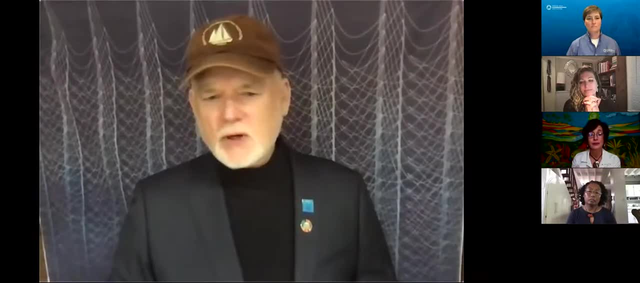 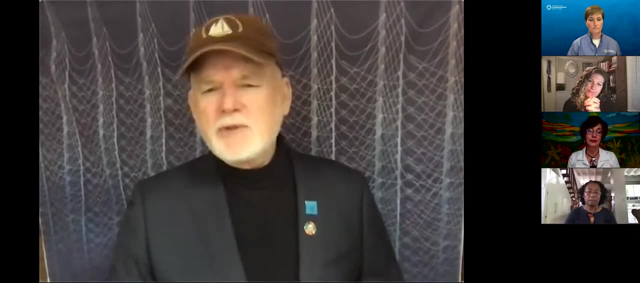 as the governor of our planet and the ultimate source of life. i think of the ocean as the governor of our planet and the ultimate source of life- life. Ladies and gentlemen, in my role as the UN Secretary General's Special Envoy for the Ocean, I'm charged with leading the global drive for the implementation. 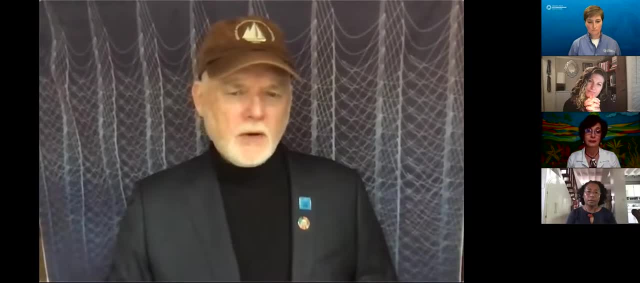 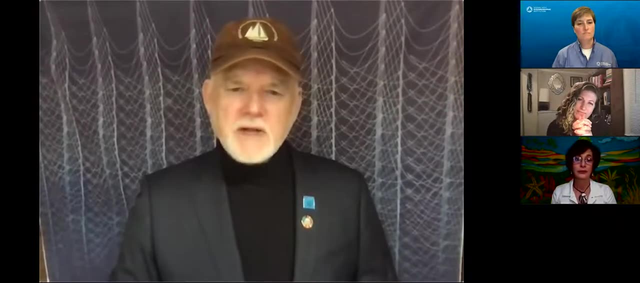 of the UN's 14th Sustainable Development Goal, known to most as SDG 14, or the Ocean's Goal. SDG 14 sets out to conserve and sustainably use the ocean's resources, and I'm sure you're all familiar with its ten specific targets.